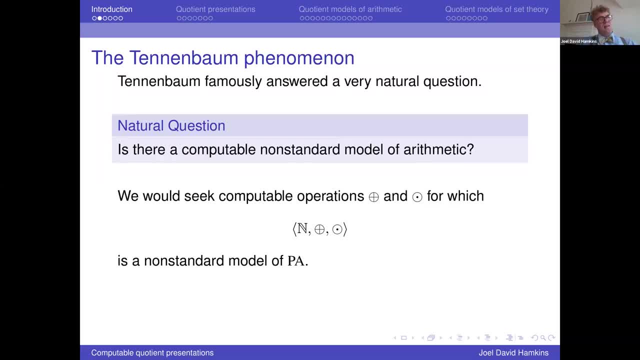 Now this question is, to my way of thinking, It's being highly relevant. It's philosophically relevant for the foundations of calculus in the following sense: Of course, Newton and Leibniz developed calculus on the basis of infinitesimals, and those were eliminated in the 19th century, of course, with the epsilon delta, familiar epsilon delta account. 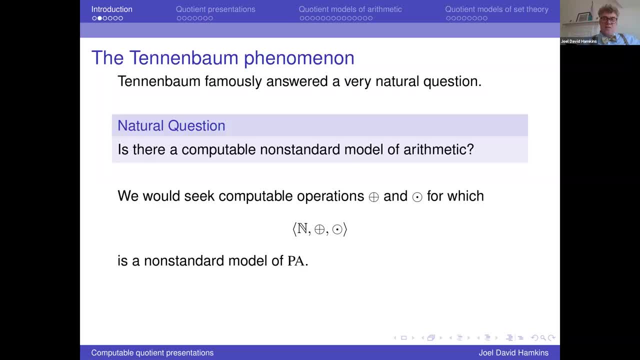 But then Robinson in the 1950s proved that it's possible to have a completely rigorous foundation for calculus using non-standard analysis. But then Robinson in the 1950s proved that it's possible to have a completely rigorous foundation for calculus using non-standard analysis, where we have a non-standard version of the reals that have infinitesimal elements and infinite elements. 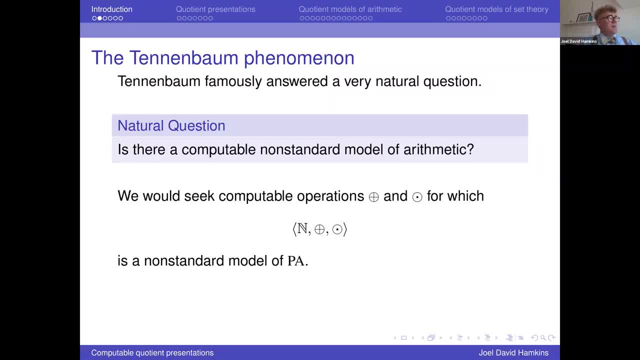 And, of course, a part of that non-standard analysis would be that you also have non-standard integers and non-standard natural numbers, non-standard rational numbers and so on, but in particular non-standard natural numbers, And so the fact that this question has a negative answer is pouring cold water. 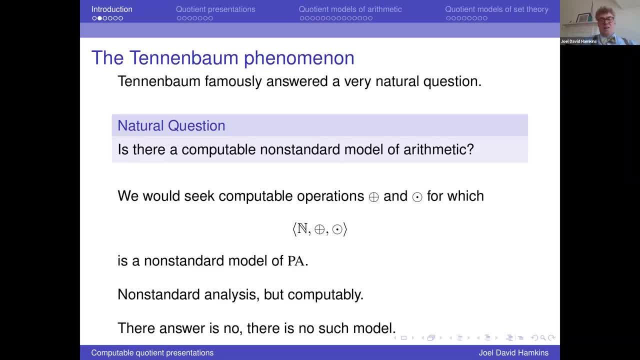 And so the fact that this question has a negative answer is pouring cold water to my way of thinking on the idea of this non-standard analysis done computably. We cannot have a calculator or a computer program that calculates in a non-standard model of arithmetic. 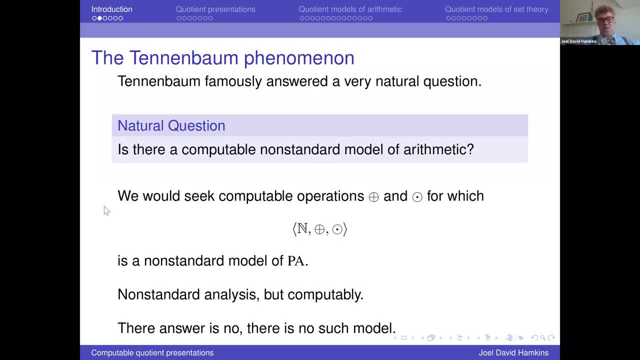 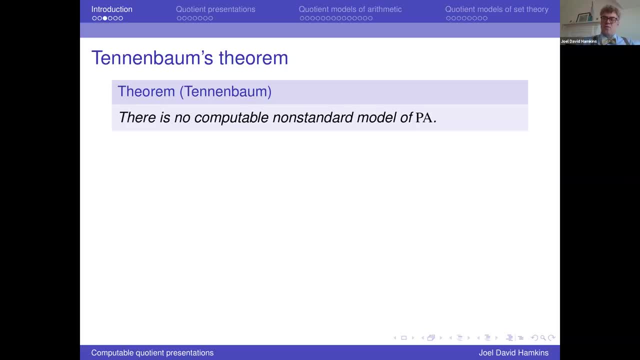 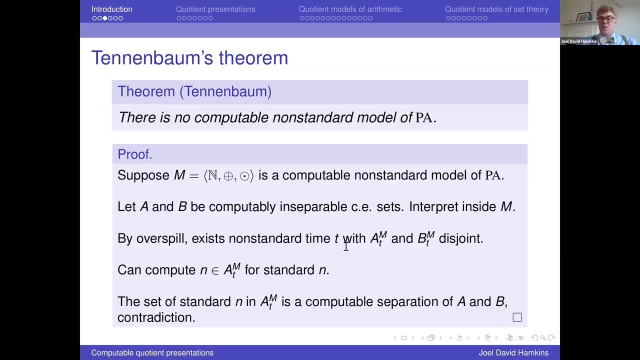 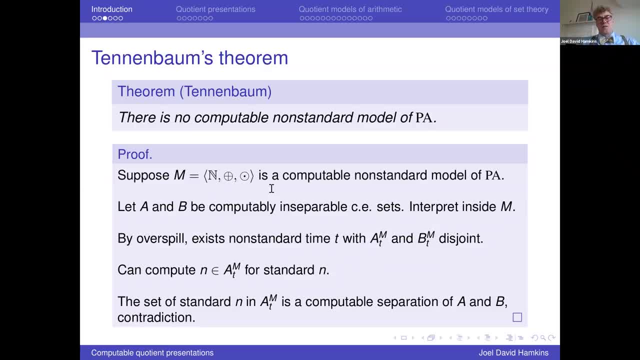 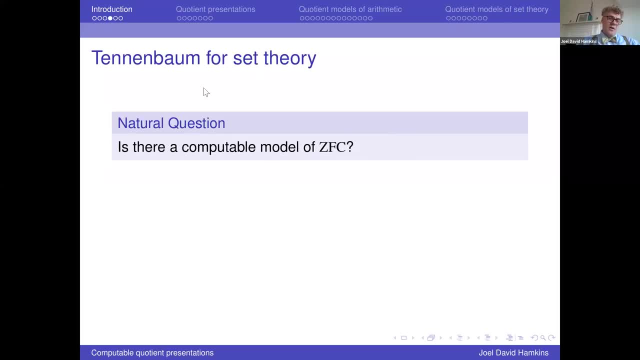 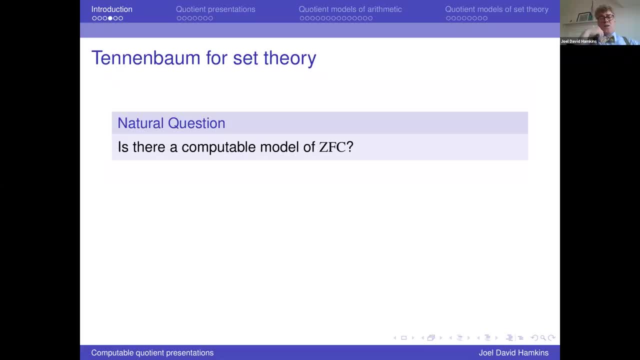 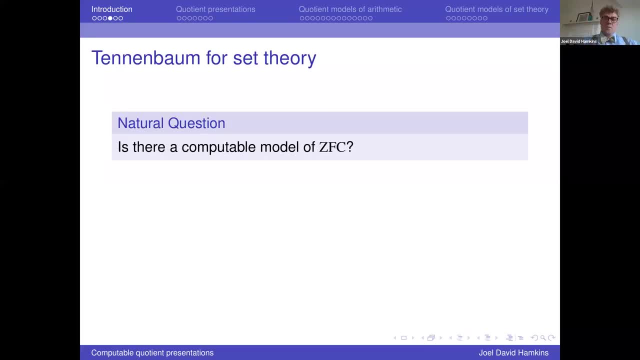 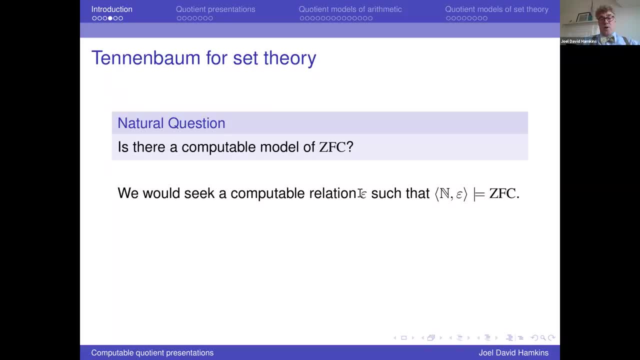 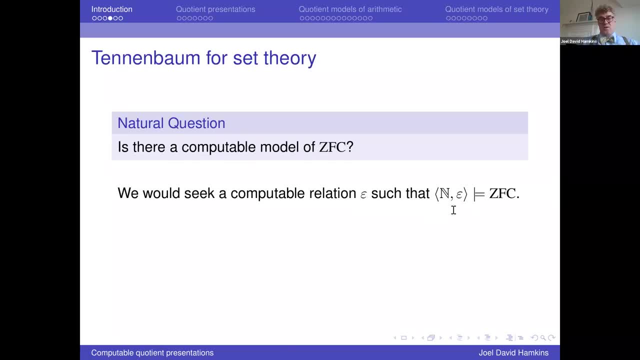 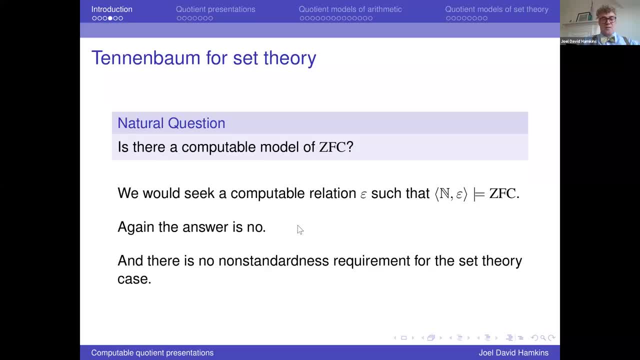 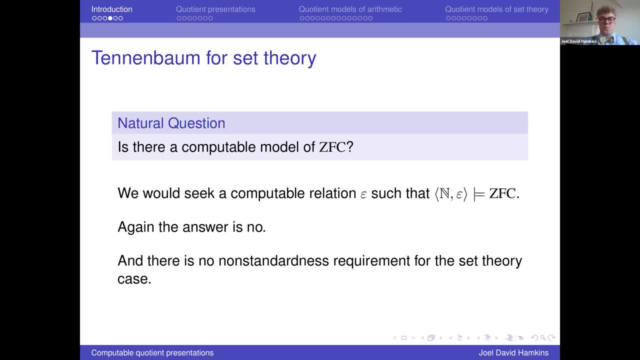 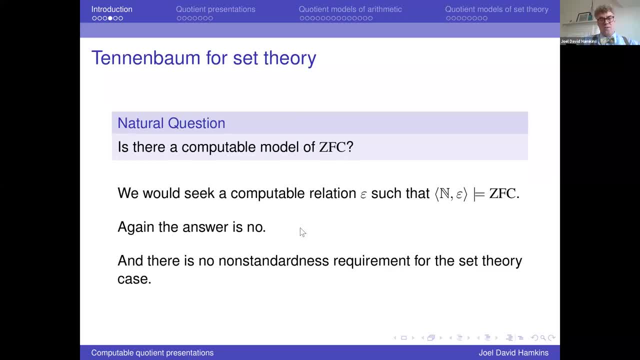 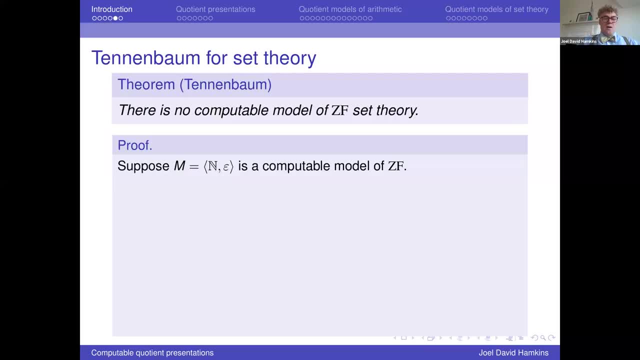 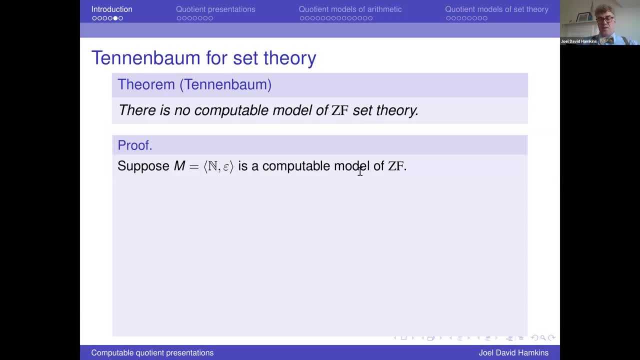 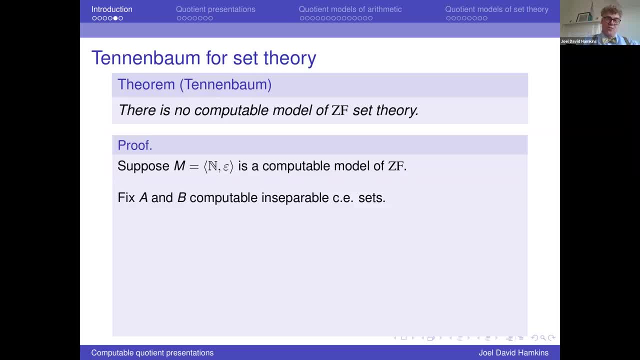 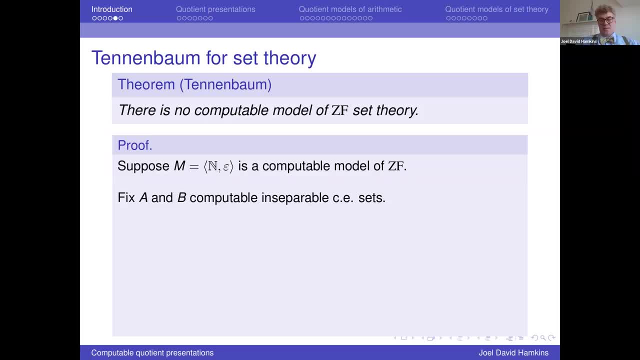 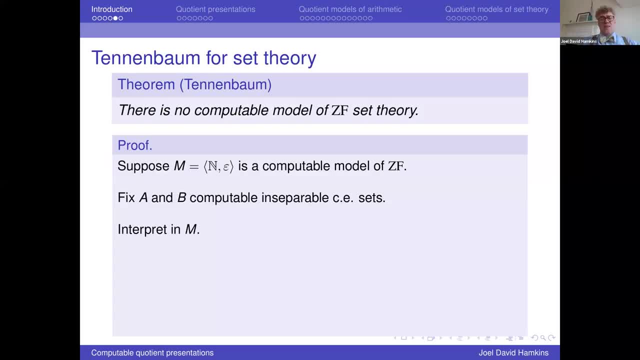 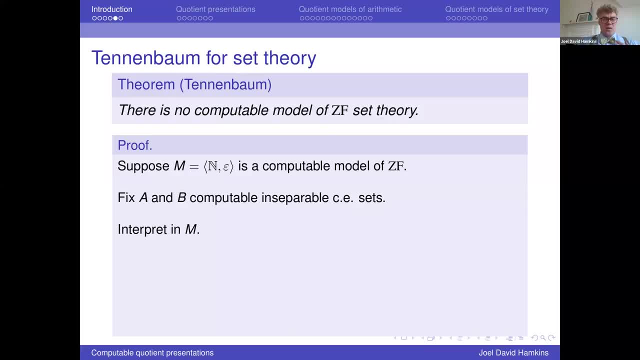 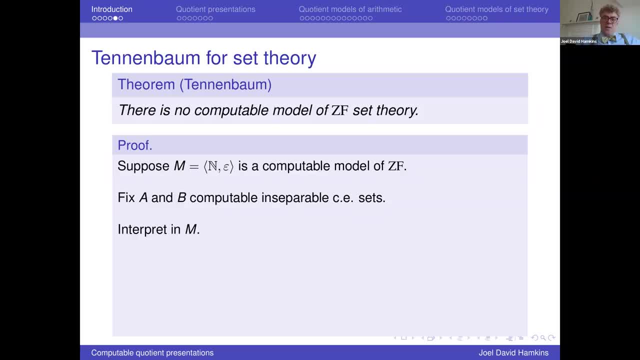 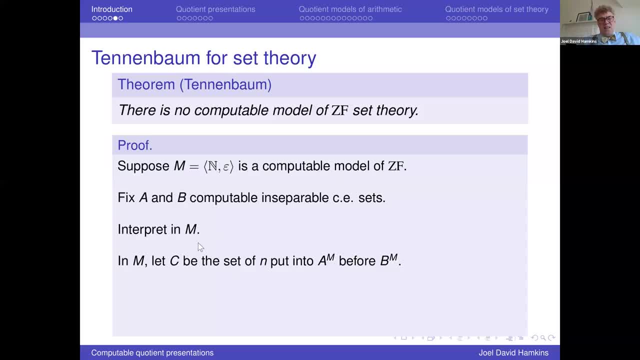 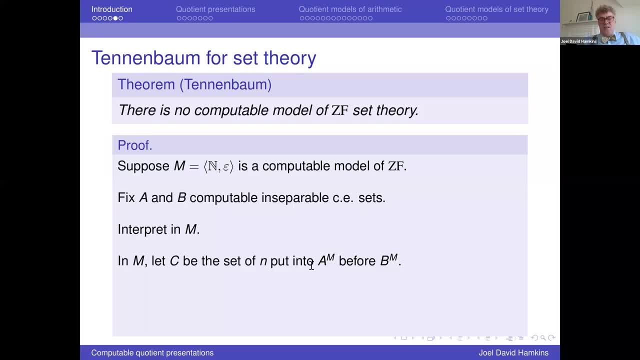 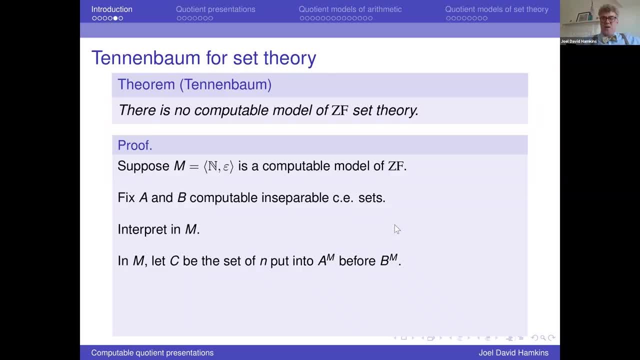 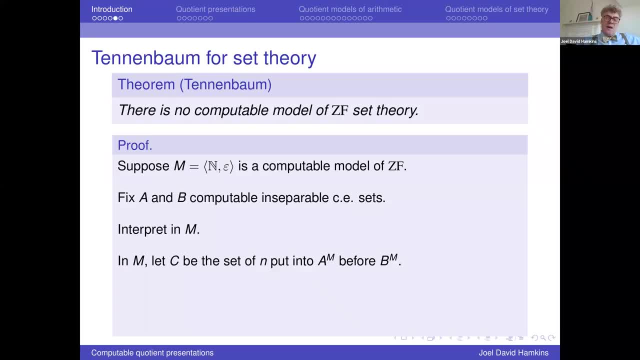 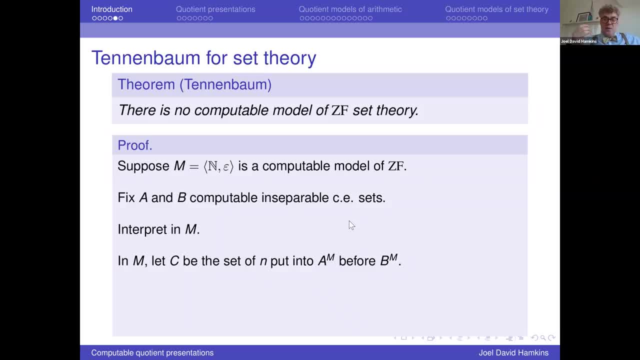 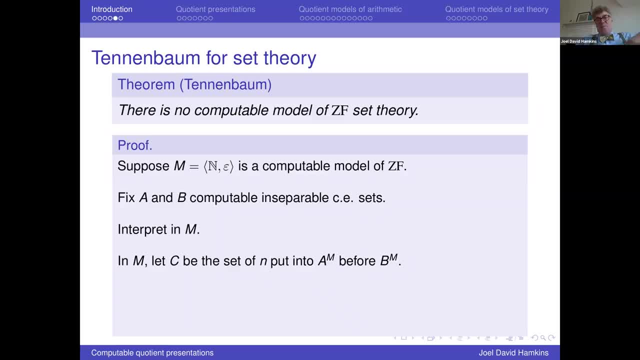 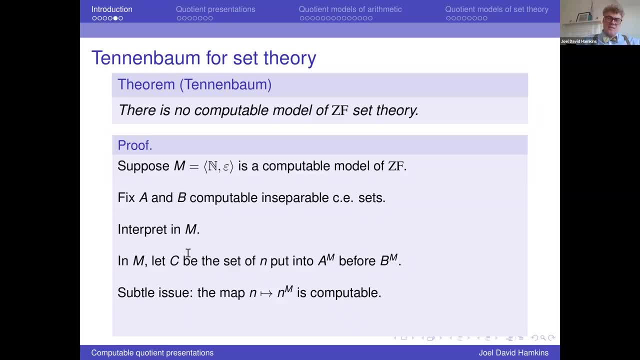 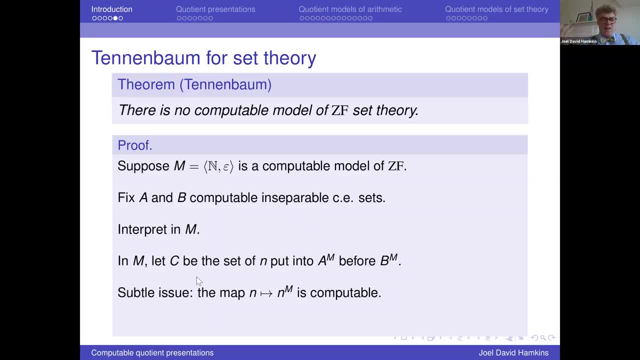 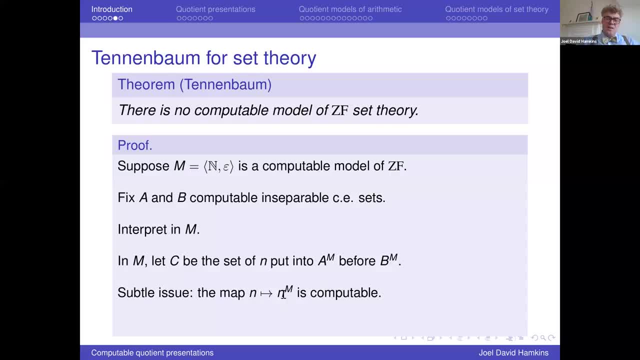 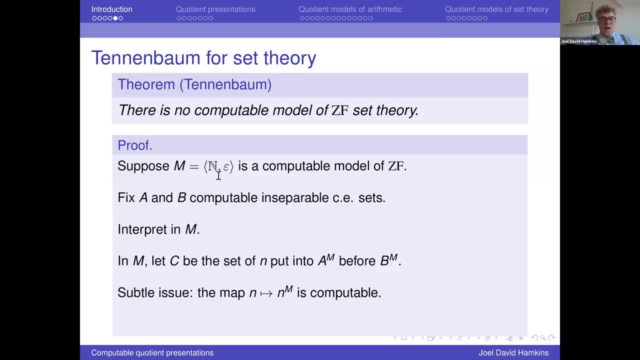 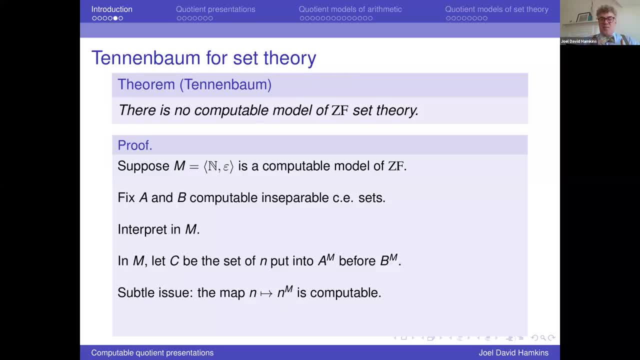 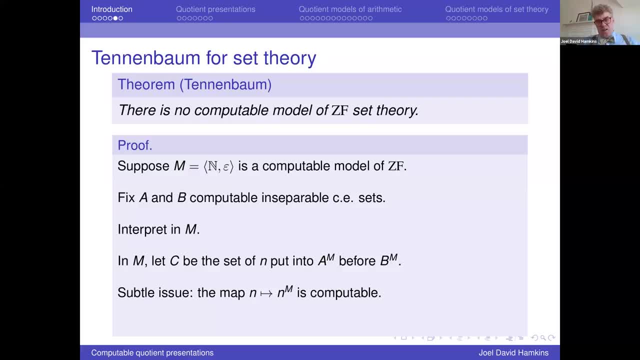 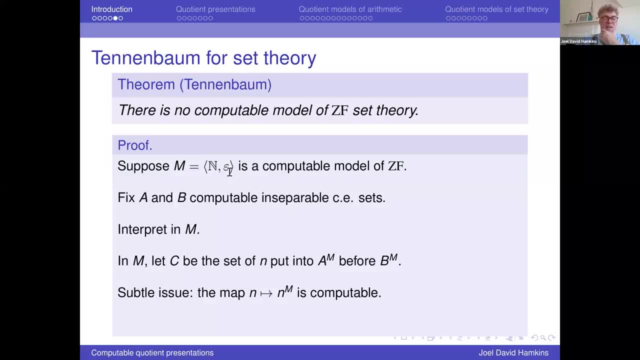 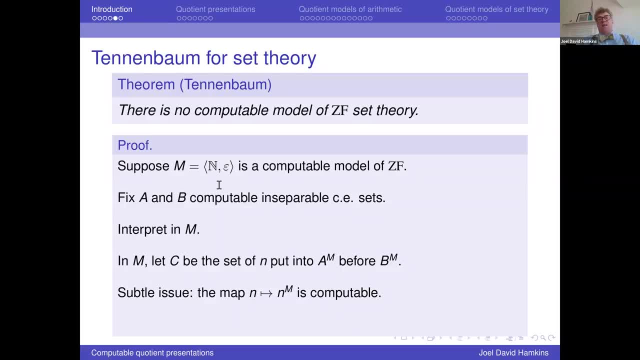 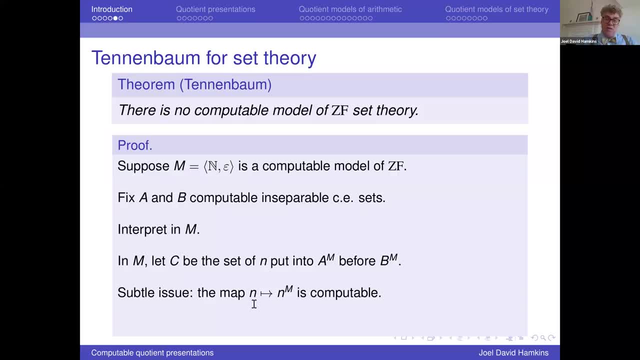 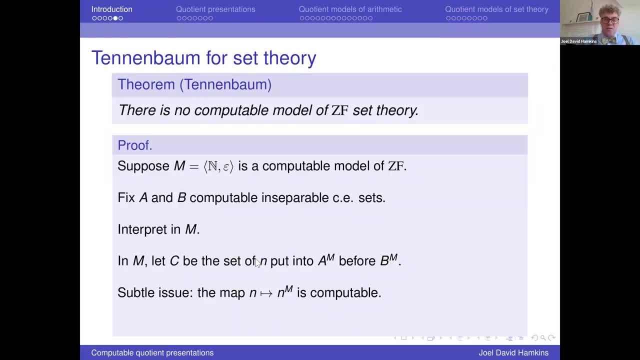 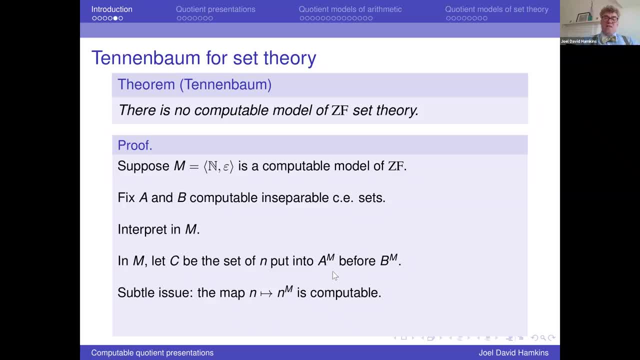 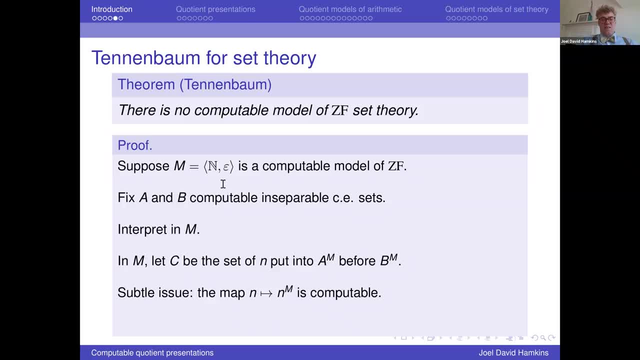 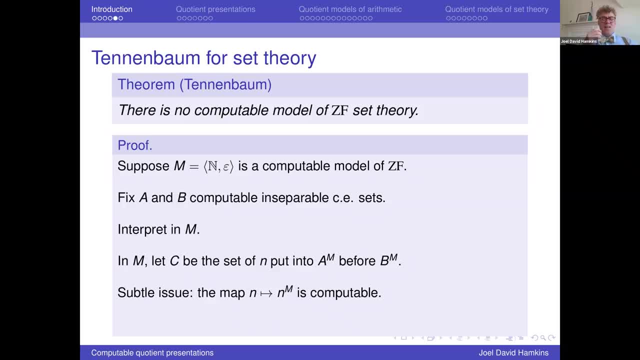 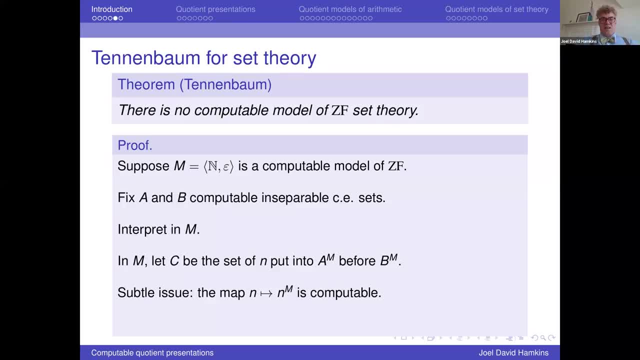 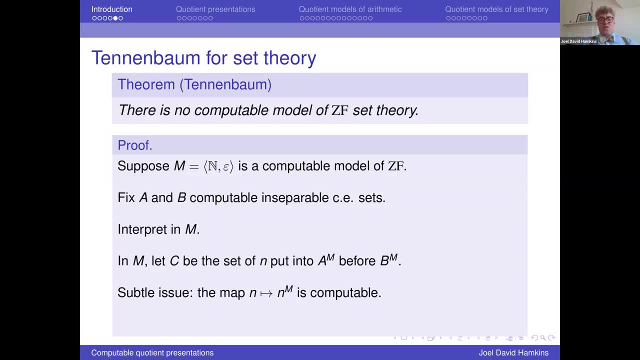 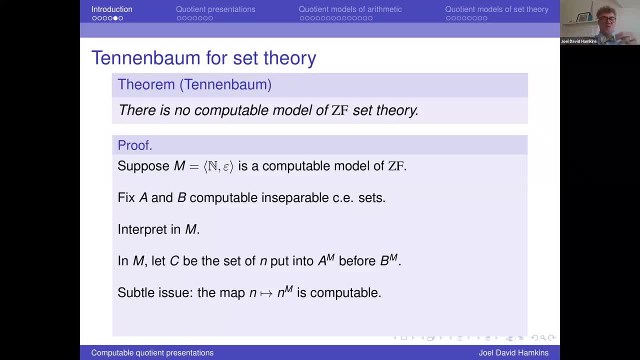 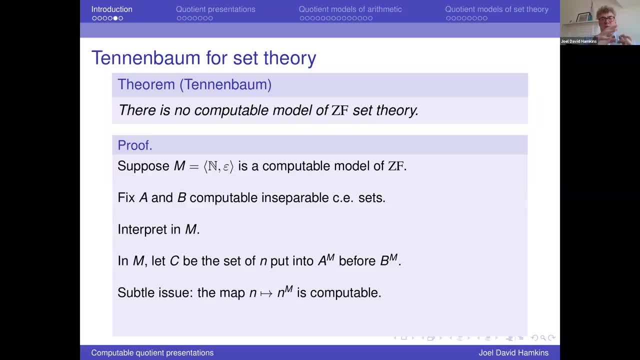 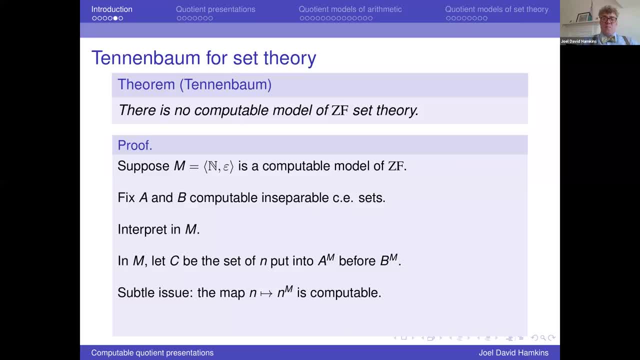 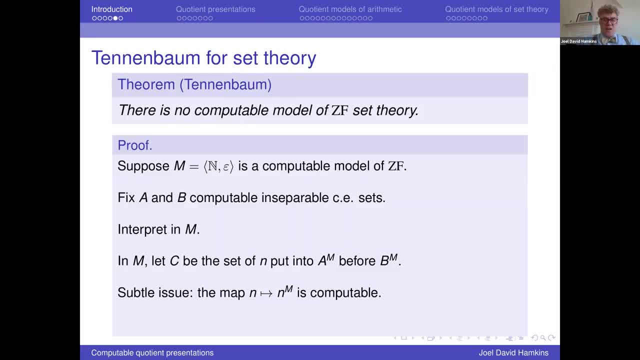 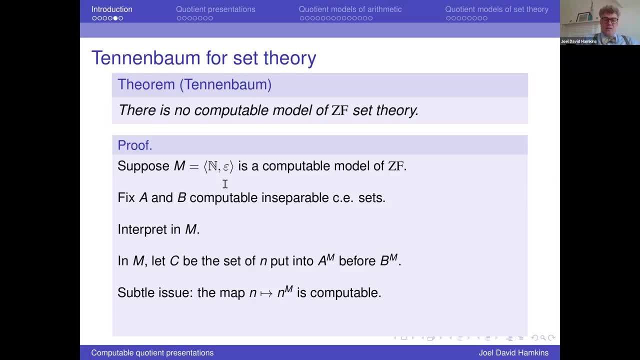 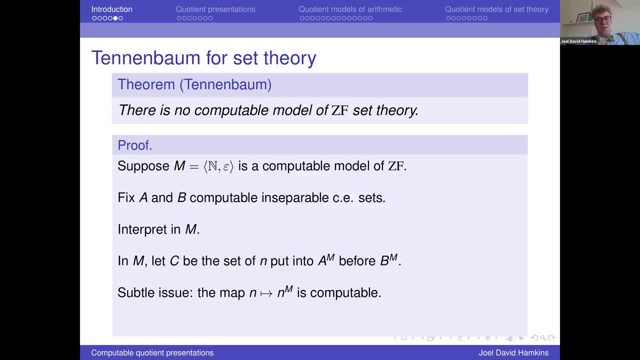 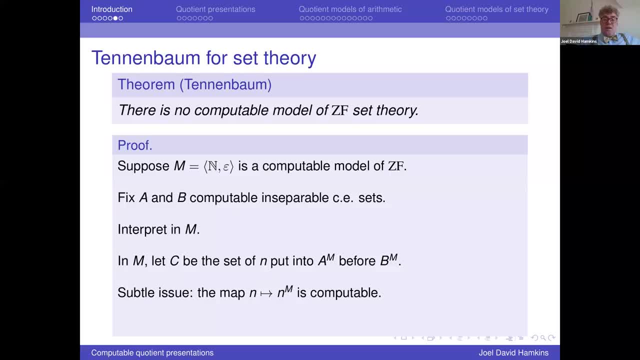 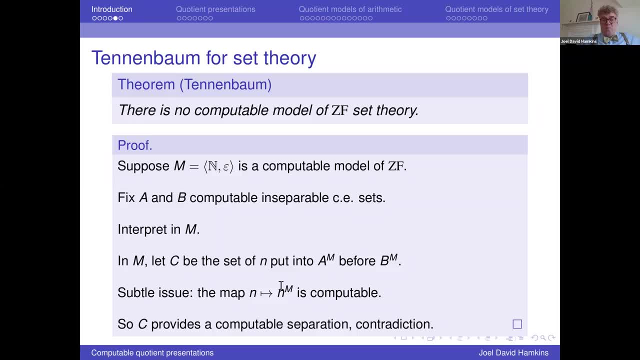 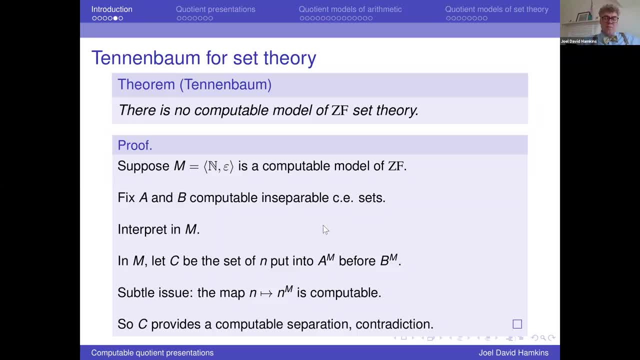 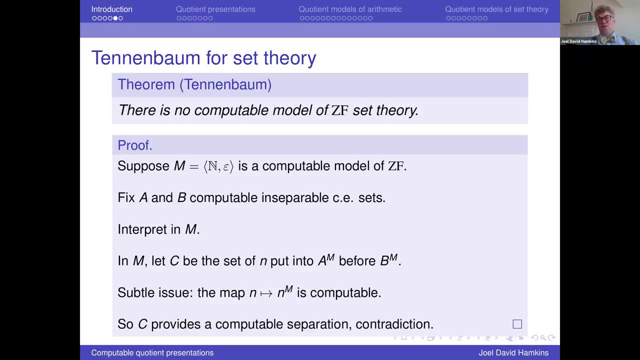 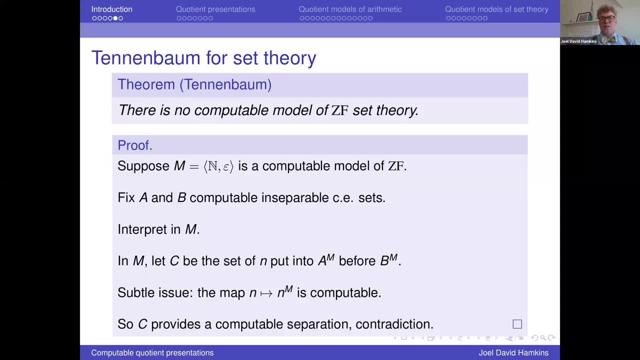 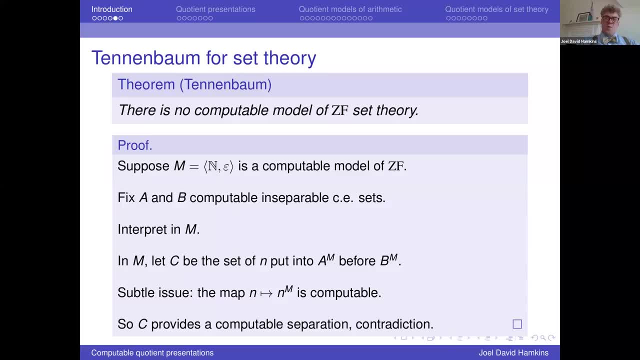 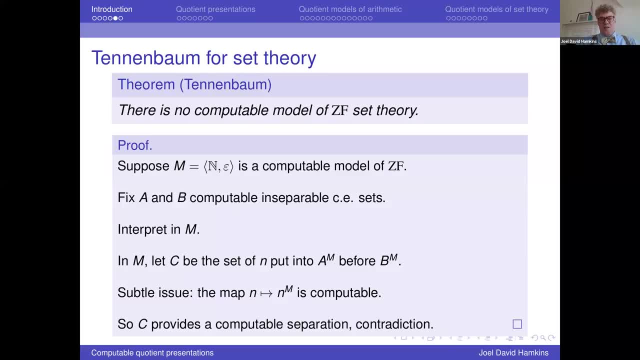 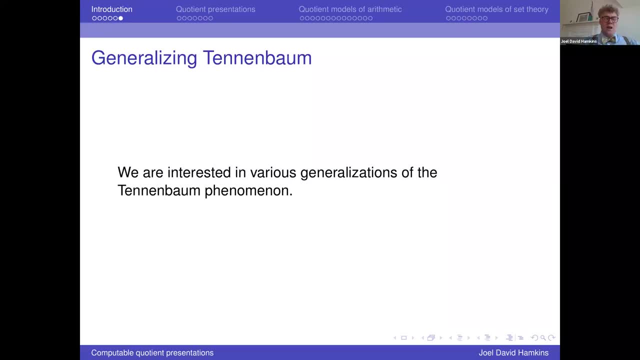 Okay, so there's no computable non-standard model of arithmetic. Okay so there's no computable non-standard model of arithmetic, something then we can hold off until the end. okay, so what i'm interested in in doing is generalizing the tenon bone phenomenon beyond. hang on one second. 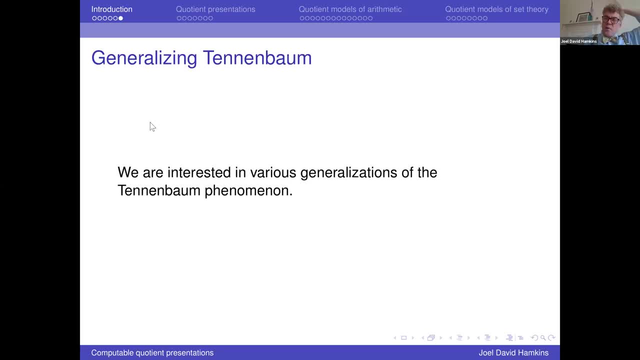 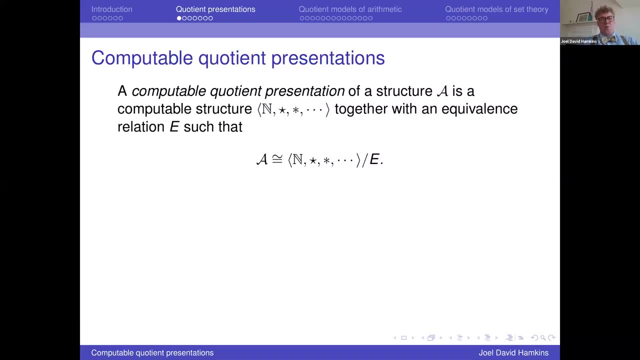 beyond those two cases, i want to look at various generalizations and in particular i want to generalize two computable quotient presentations. so what is that? a computable quotient presentation of a structure is a computable structure. so i've got the natural numbers with some computable functions and relations on it, together with an equivalence. 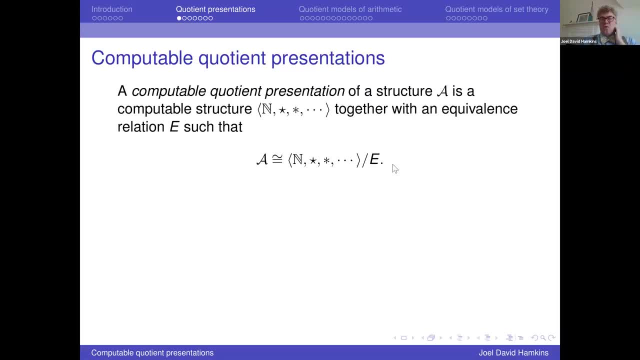 relation e, so that the given structure is isomorphic to the quotient. okay, so it's a. it's a quotient construction, but i don't insist that e is computable. okay, so i've got a. it's a quotient of a computable model. that's what a computable quotient presentation is. 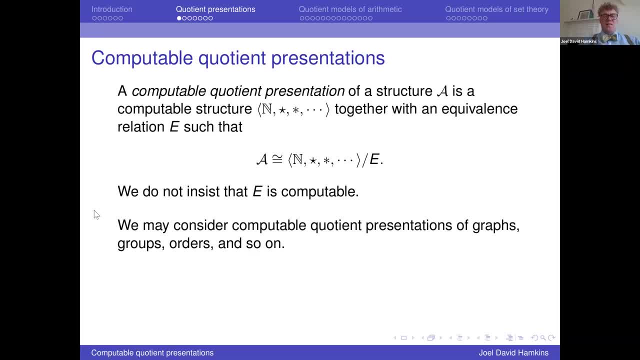 and so of course, one can consider computable quotient presentations of graphs or groups or orders or whatever you like, models of set theory, models of arithmetic. um, now in it, when you have sure question. so this is arnold. uh, can you, can you, can you ask for that a, that e is arithmetic or? 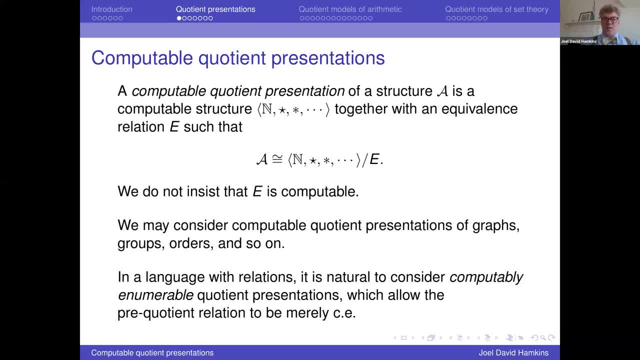 something like that, or define: yeah, sure, yeah, we're going to look at that refinement. so ce or coce or whatever arithmetic projective, whatever you like. yeah, and those are going to be interesting questions and in fact that issue is going to come up later. thank you, okay. so when you have, when you have. 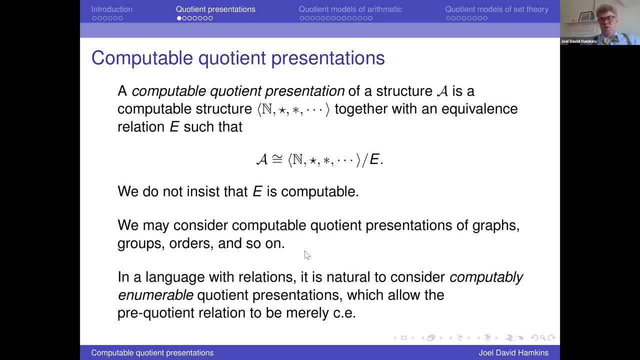 relations in your language, for example, in the case of set theory, then it's also natural to look at, say, computably enumerable quotient presentations where the relation is only ce, instead of being computable here. if they're functions and so on, then asking for a ce graph or computable, is the 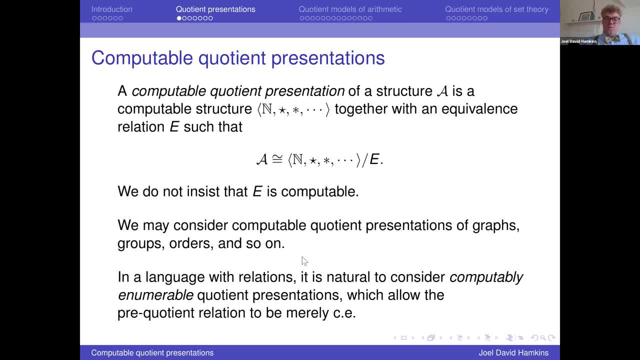 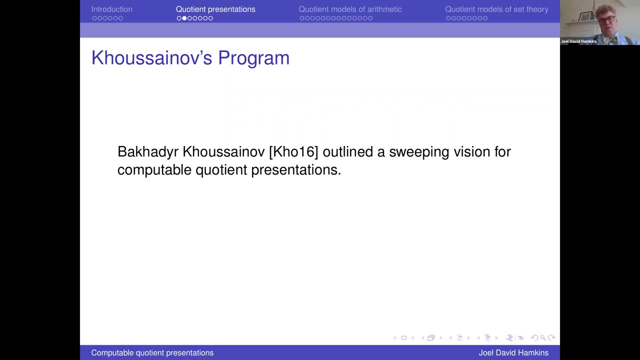 same thing, but when it's a relation, then it's a natural uh relation. so i'm going to look at that refinement of the situation to ask for the basic structure to be, say, merely ce instead of computable. okay, so let me mention bakaida kusainov's program. so in a 2016 conference in 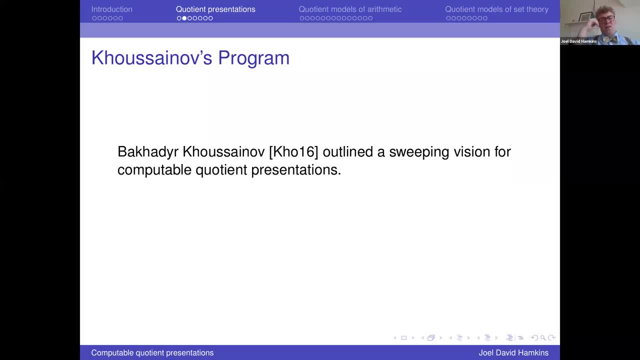 kyoto that i was at, he outlined a sweeping vision for computable quotient presentations and proposing them as a very fruitful alternative approach to computable quotient presentations. so in this case we're going to look at the notion of non-computable model theory with certain uh. 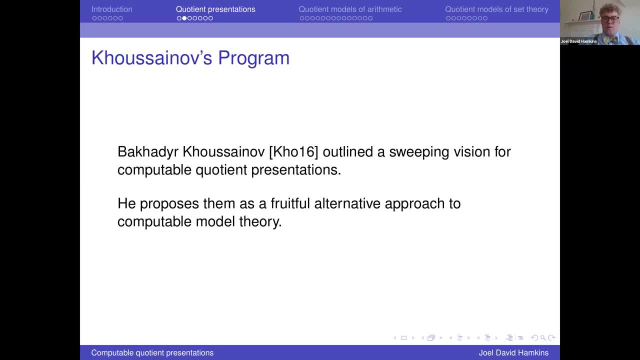 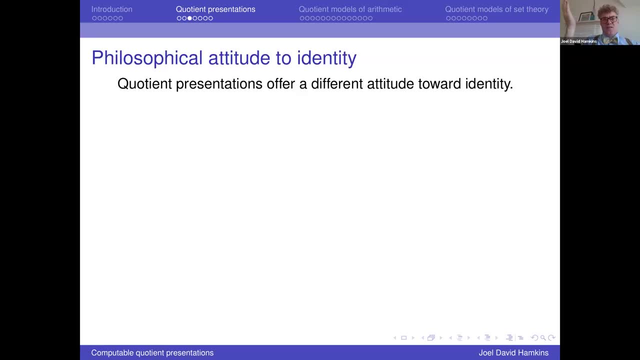 with a certain philosophical, uh attitude that i'm going to explain, and that is this attitude towards the identity relation. so quotient presentations offer a fundamentally different attitude towards equality. i mean, of course, because they're quotions. but, uh, and what is this in the case of computable presentations? so when you don't do any quotienting and you just do ordinary 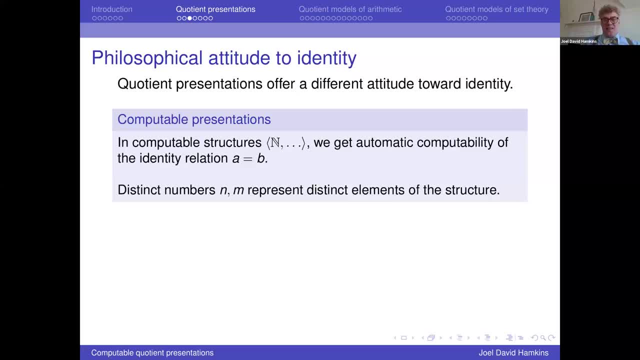 computable model theory, then you get automatic computability of identity. If you have two numbers, then if they're the same number, then they're representing the same object in the model, And if they're different numbers then they're definitely representing different objects in the model. And so it's kind of built. 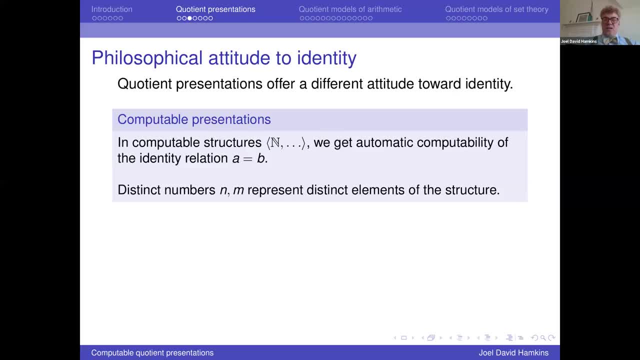 into the framework of ordinary computable model theory that you know when things are equal and when they're not equal, because if numbers are not equal, then they're not equal in the model. But in a computable quotient presentation we relax that property a little bit, So we can't. 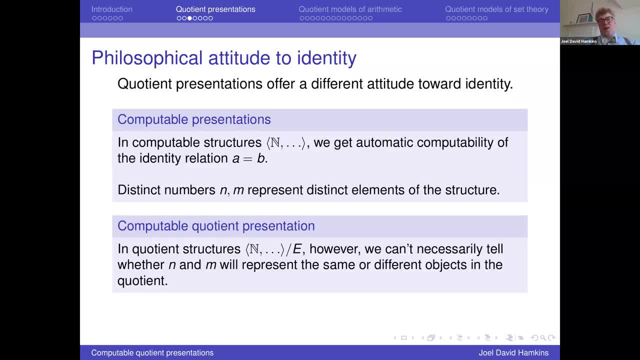 give in two different numbers. We don't really know whether or not they're representing the same object in the quotient or whether they're representing different objects in the quotient, because that has to do with the complexity of deciding the e-relation, the equivalence relation. 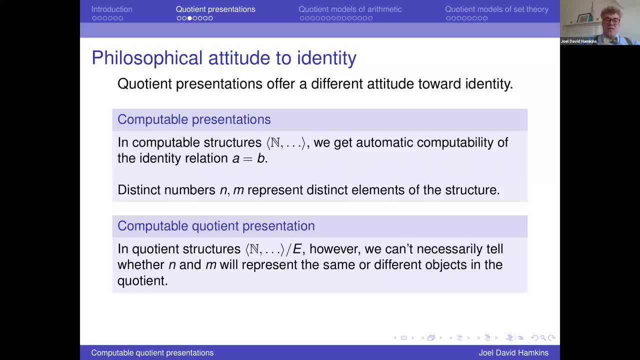 is the equality relation in the quotient, And so it could be that we can't tell whether we have different objects or not. Okay, So the part of the attraction of the quotient presentation is to loosen this computational grip of computable model theory on the identity relation. 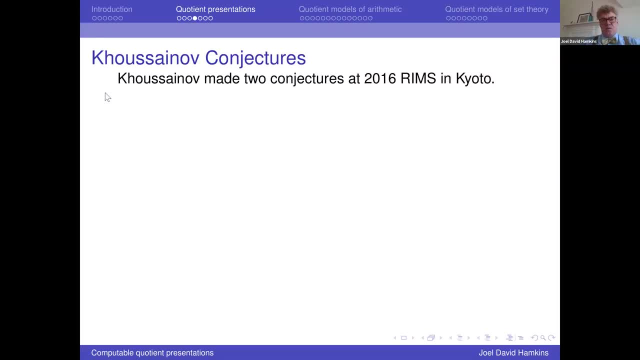 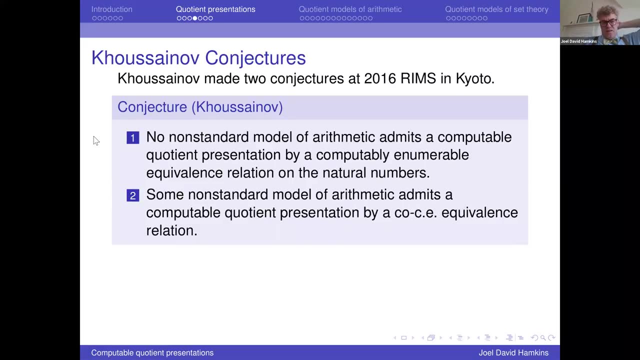 Okay. So at that conference in Kyoto, Bach had made two conjectures, the following. So he said: no, non-center model arithmetic should admit a computable quotient presentation by a CE equivalence relation. And: but if you allow a co-CE equivalence relation, then he thought it should be possible. 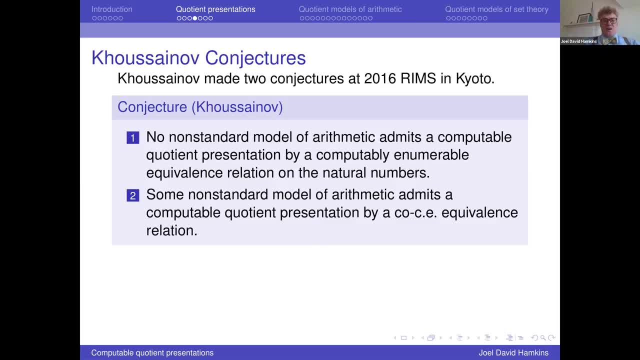 Okay. So those are the two conjectures. They're both generalizations of Tenenbaum. The first one is directly generalizing Tenenbaum, saying you can't do it with a CE relation, And this is sort of an anti-Tenenbaum theorem, saying with co-CE you should be able to do it, Okay. So in this talk, 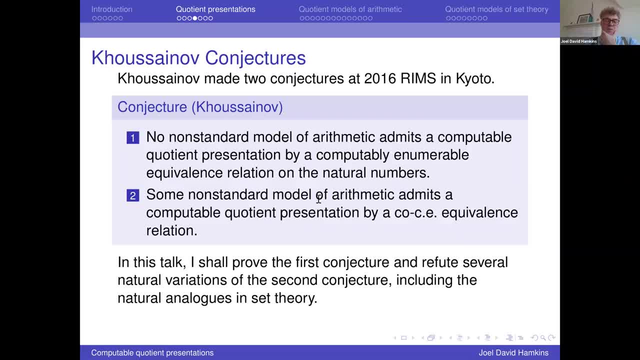 I'm going to prove the first conjecture and I'm going to refute some of the other conjectures that I've talked about. So I'm going to prove the first conjecture and I'm going to refute some of the other conjectures that I've talked about. 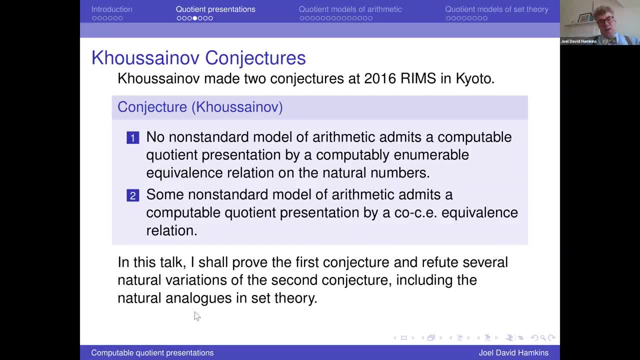 So I'm going to refute some of the other conjectures that I've talked about. Okay, So I'm going to refute some variations of the second conjecture, including the natural analogs and set theory, but some of the variations are still open. 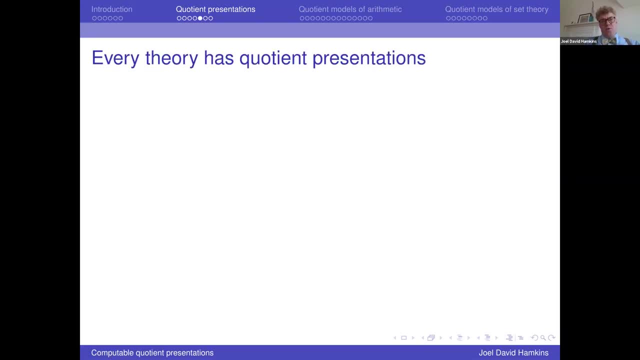 Okay. So let me, before doing that proof, let me just mention that there's a sense in which every theory has quotient presentation, So every consistency theory in a functional language. so if there's no relation symbols, then you always get a computable quotient. 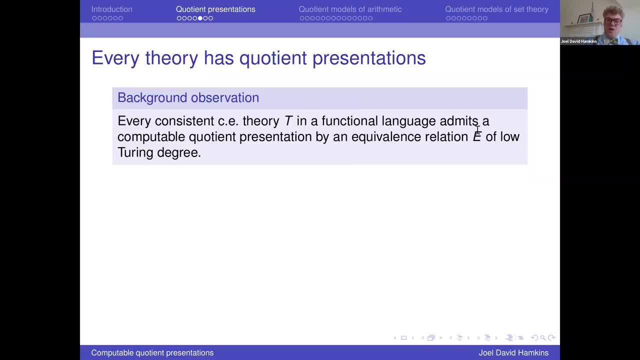 quotient presentation by an equivalence relation of comparatively low turn degree. So, Anand, you never need to go very high in the arithmetic hierarchy, just even low is good enough. And this is just following from the computably effective completeness theorem. So if you think, 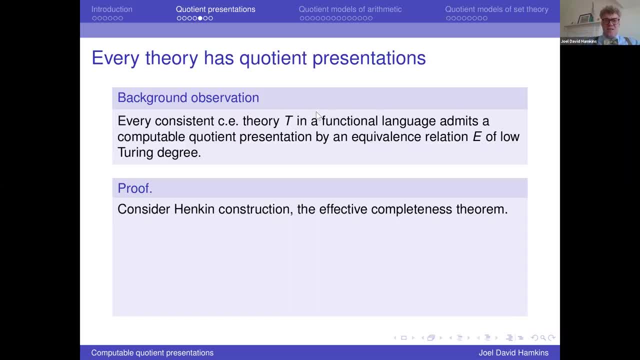 about the Henkin construction. you start with this consistency theory, then you add in the Henkin assertions, add in Henkin witnesses and you consider the tree of attempts to complete the theory. So we build the tree and we keep building the tree, but at any point when we're adding, 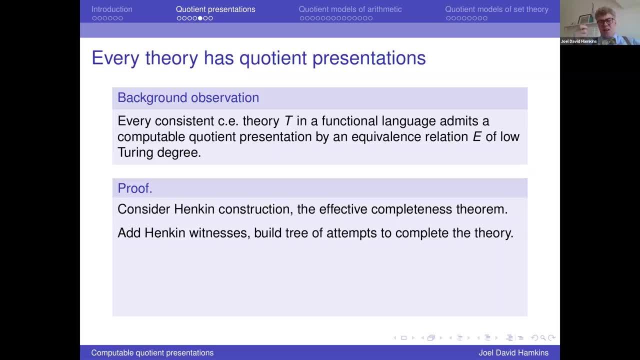 branches when we're adding nodes to this tree. so we add a sentence or a snagation and so on, as long as what we're looking at seems like it's consistent. But if we build high enough that we find the contradiction, then that node stops growing. 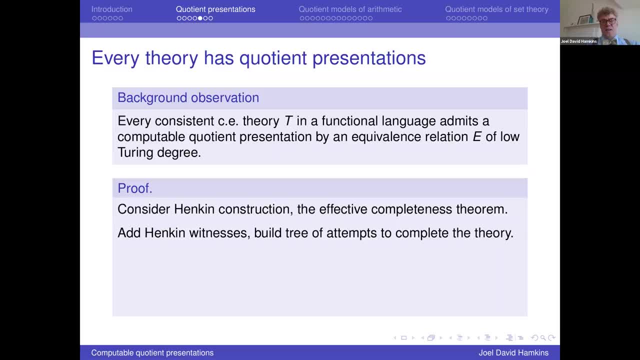 And so this is the tree of attempts to find a complete, consistent Henkin theory, extending the given theory, So that can be done computably, And the key point is that the term algebra, if we just look at what terms, what syntactic compositions of terms from the Henkin constants, 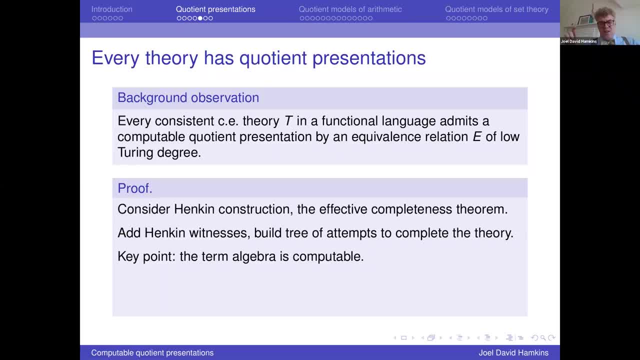 can you form? Well, you can take f and g and so on. You can build up the term algebra and that's computable. That's the main idea of this proof. The term algebra is a computable algebra If you don't have to. 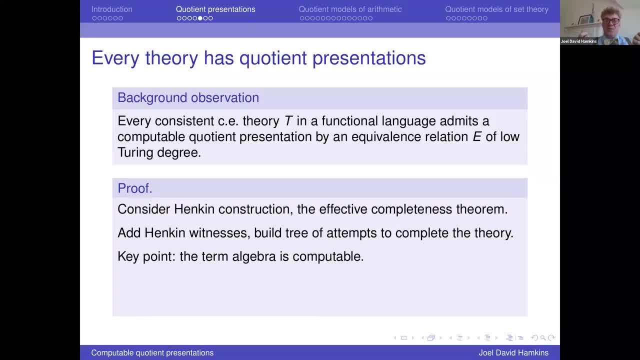 form, the identity between the terms. you just build the terms. then well, if I have a function symbol and I have a bunch of terms, then I can apply that function symbol to those terms by just building another term. And that's a computable thing to do at the level of syntax. And so the 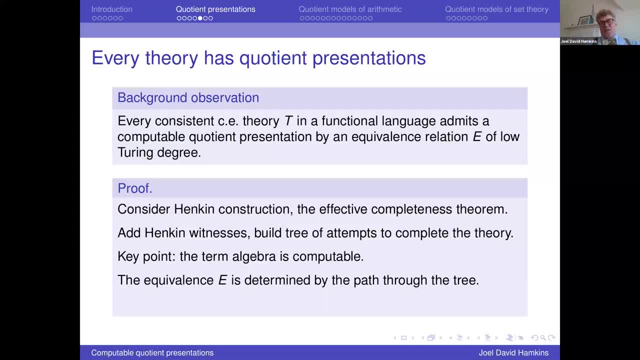 term, algebra is complete and the equivalence relation is what comes from the branch to the tree. Of course, I pick a branch to the tree that's going to tell me when I should identify two terms as being equal or not, And then 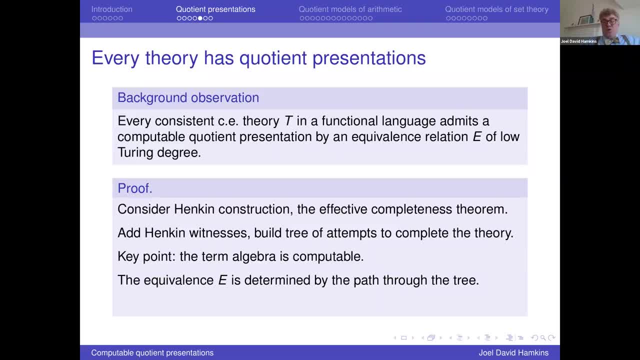 of course, the Henkin proof shows that the resulting quotient is a model of the theory, And so what we've got here is a computable structure, the term algebra modding out by the equivalence relation, which might not be computable. that comes from the branch to the 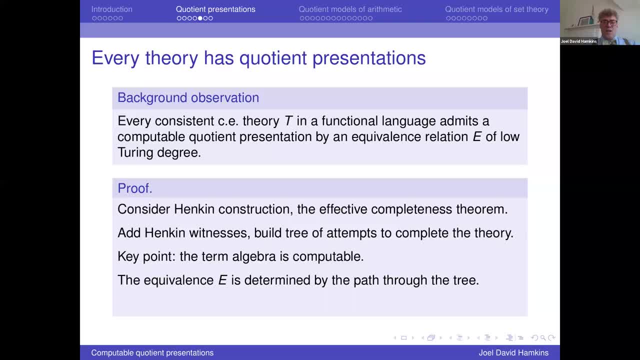 tree, But the equivalence relation will be low because every computable tree has a low branch. Okay, so the slogan is that the Henkin model is a quotient of the term algebra and therefore every CE functional theory has a computable quotient. presentation: 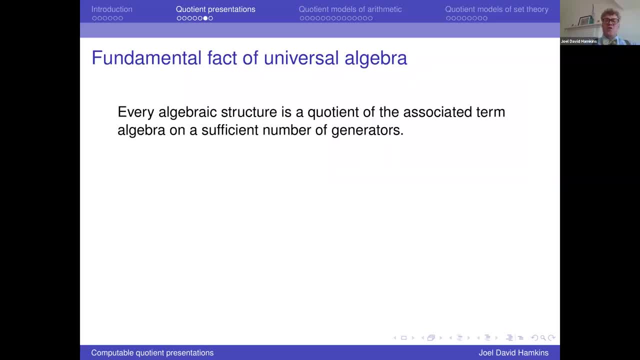 Okay, now of course, this is highly relevant in the context of universal algebra. When you're doing first-order logic, without any relation symbols of course, then you always have this term algebra hanging around, and every algebraic structures the quotient of the associated term algebra with enough. 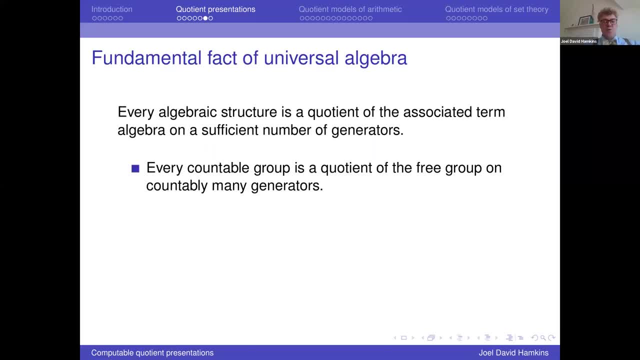 generics. So there's going to be a couple of questions here as to: is this something like a? So every countable group is a quotient of the free group. uncountably many generators and so on. In general, every countable algebra. 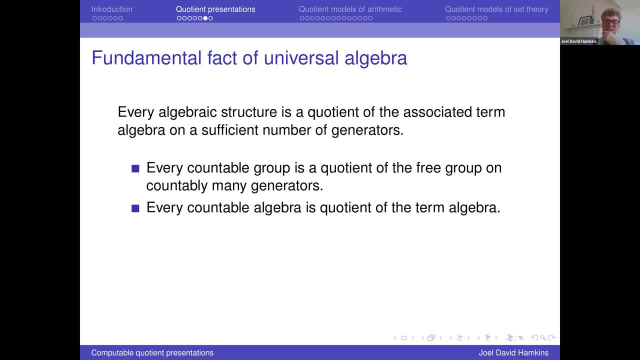 is a quotient of the term algebra, And so, in a sense, this computable quotient idea is much more relevant for universal algebra than for model theory. when you have relations, It works much, much better in that case. OK, so in purely functional languages, 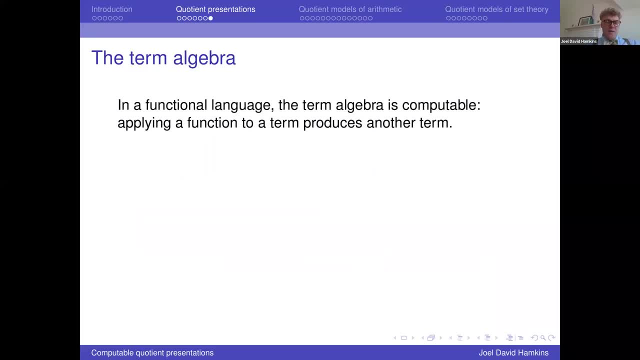 it's a much better and more satisfying theory. OK, oh, let's see this is a little redundant here. OK, so the term algebra is always computable because you can just apply the function syntactically to the terms and make another term. 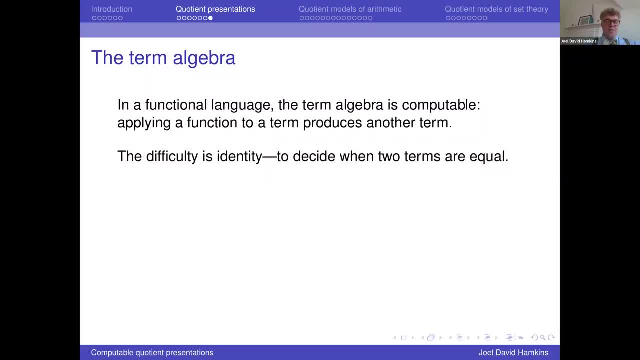 And what's difficult is to decide when two terms are representing the same thing, And that's where the identity or equivalence relation comes in, when you're forming the quotient. So, Buchheider, He presents this as what he calls the domain problem, Namely every equivalence relation E. 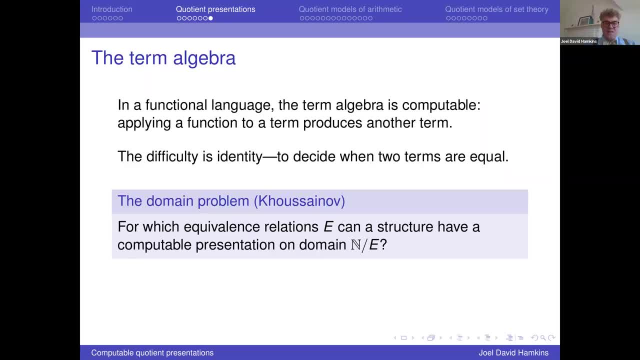 determines a kind of domain, the quotient, the equivalence classes, And the question is: for which equivalence relations can a structure have a computable presentation on that domain, Or which classes of equivalence relations, so CE or coCE, or a certain level of arithmetic hierarchy, or what have you? 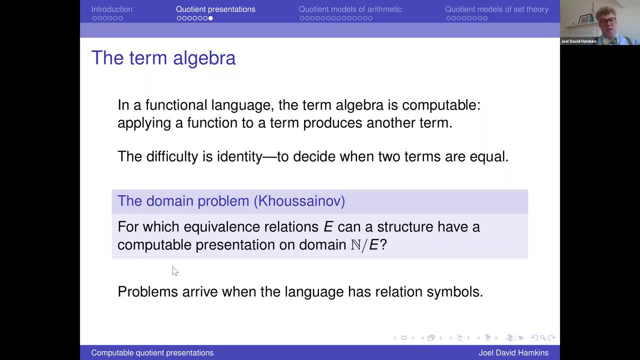 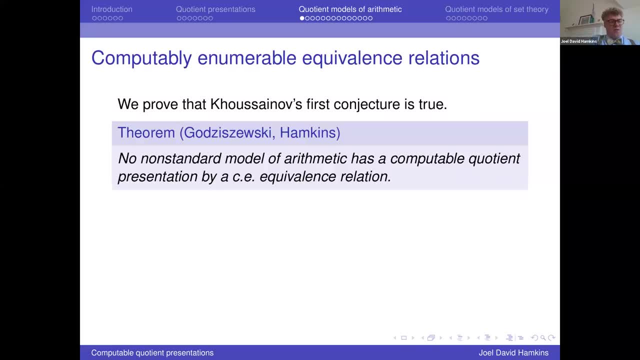 OK, so there's certain problems arise when you have quotient presentations of models of arithmetic, And I want to prove that the first conjecture is true. So this is our theorem. So no, non-centered model arithmetic has a computable quotient presentation by a CE equivalence relation. 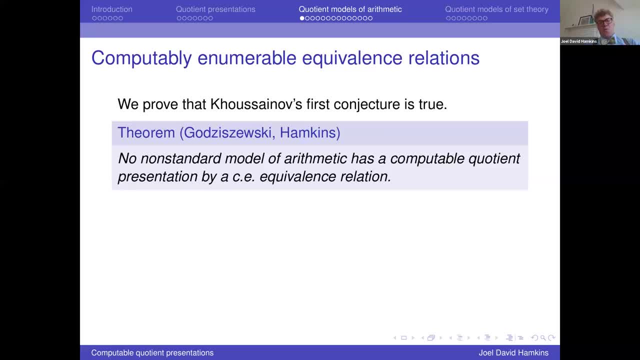 So this is Tenenbaum's theorem for quotient presentations by CE equivalence relations. So here's the proof: We're going to prove that the non-centered model of arithmetic has a computable quotient presentation by a CE equivalence relation. So let's see: 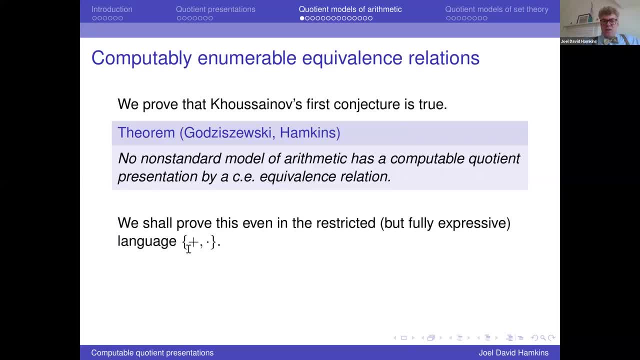 OK, We're going to prove it in the restricted language, even the functional language, Of course. in arithmetic you can define the order from the arithmetic So expressively you don't need the order, although the traditional language of arithmetic has plus times 0,, 1, and less than that. 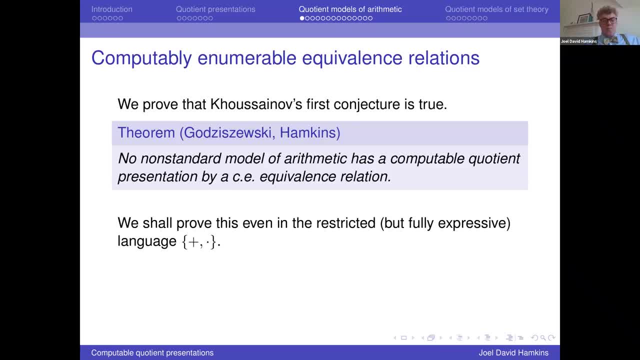 But we can prove this theorem even just with plus and times. OK, so the claim is that there's no computable structure whose quotient by a CE congruence relation gives you a non-centered model. OK, So let's do the proof. 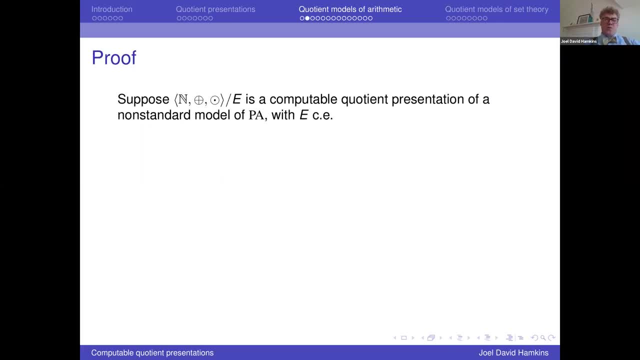 So suppose we had one, Suppose we had a computable quotient presentation that was forming a non-centered model of PA. OK, so of course there's some natural number that's representing the number 0 and some other numbers representing the number 1.. 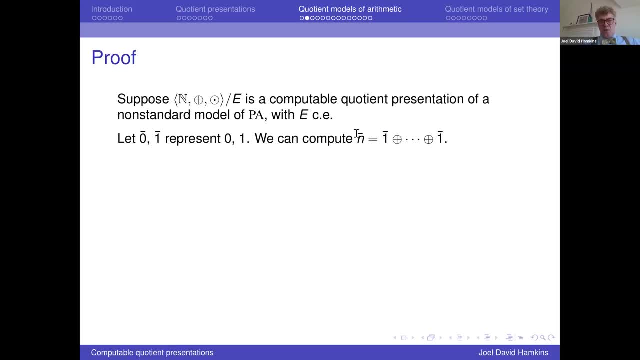 And because this plus operation is a computable operation, we can compute the number that's going to, that's going to represent n. For any n, we can compute a representative of n. Of course it might have many representatives And this is just going to be one of them. 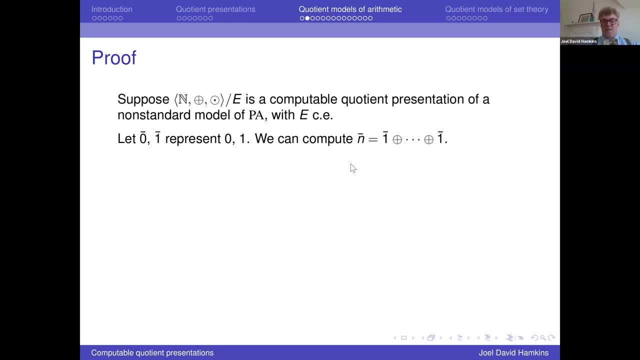 But we can compute. one of them is the point using the fact that plus is computable, And now again, just like in the Tannenbaum proof, fix computably inseparable CE sets And we can interpret the programs that do the enumeration. 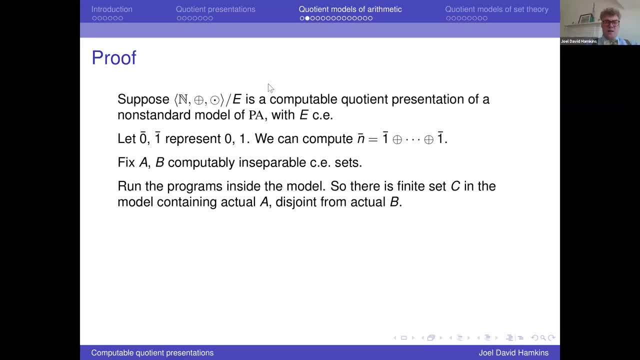 We can interpret those programs inside this model. This is a non-centered model of arithmetic, So it is perfectly capable of talking about Turing machine computations. And so if I again go to some non-standard stage of the enumeration procedure at which the programs are still 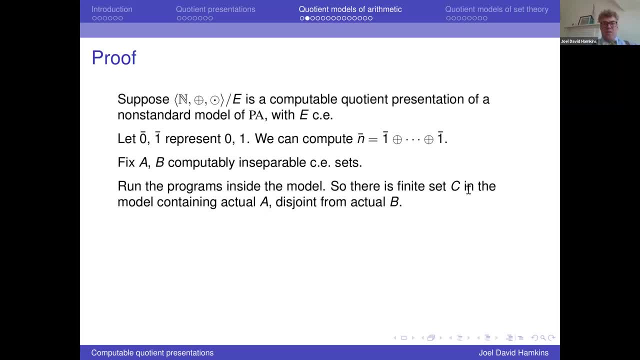 enumerating disjoint sets, then there will be some set inside the model that the model thinks is finite. It's actually infinite, but it's a pseudo-finite set. It's a non-centered finite set And it contains the actual set A and it's disjoint. 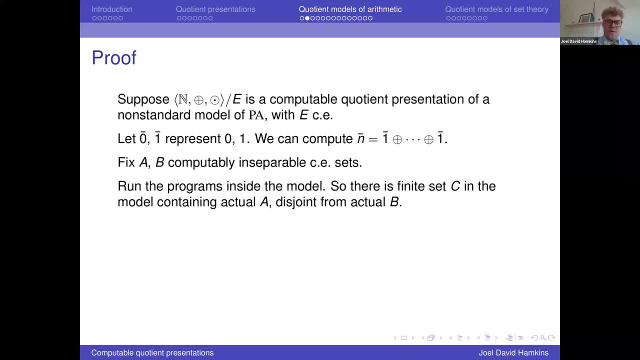 from the actual set B. And now of course we can code this set C with, say, the prime product coding. So inside the model it's a definable set. I'm going to multiply all the primes together that are indexed by elements of that set inside the model. 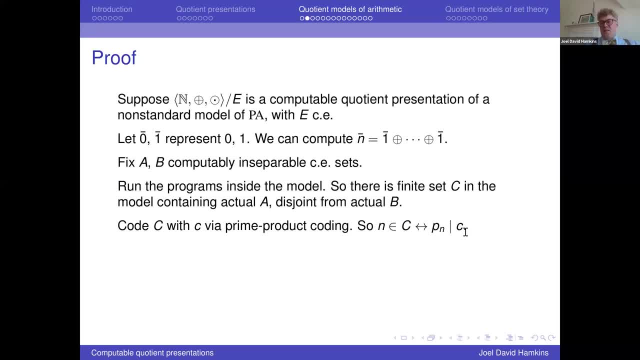 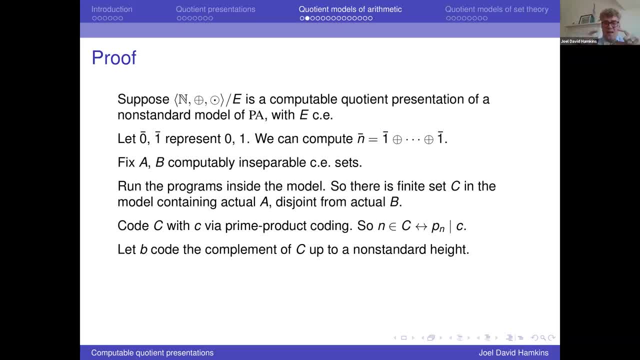 to that same height. So I've got these two finite sets and their complements up to that non-standard stage. And now for any given n. this is a standard n. This is what we're going to do now, outside the model. 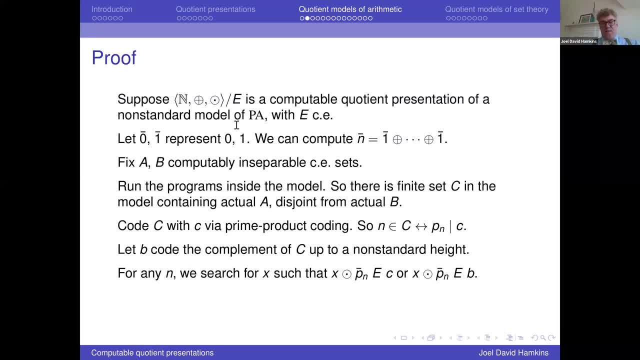 For any given n. we're going to search for an x in the natural numbers so that if I multiply x by Pn bar, which I can compute, I want to ask: is it E equivalent to C, Or can I find an x so that if I multiply x by Pn bar? 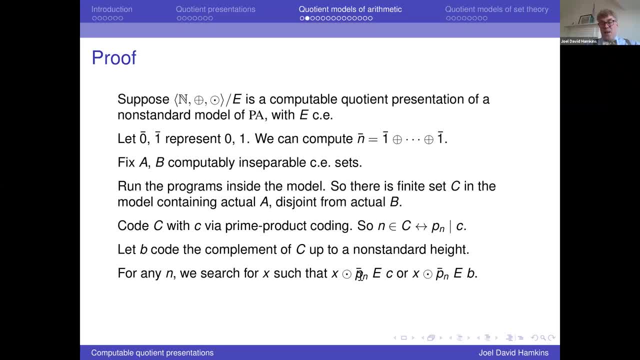 it's equivalent to B. So in other words, I'm asking: does Pn divide C or does it divide B? It's going to divide exactly one of them because they're complements And the model thinks that exactly one of those things. 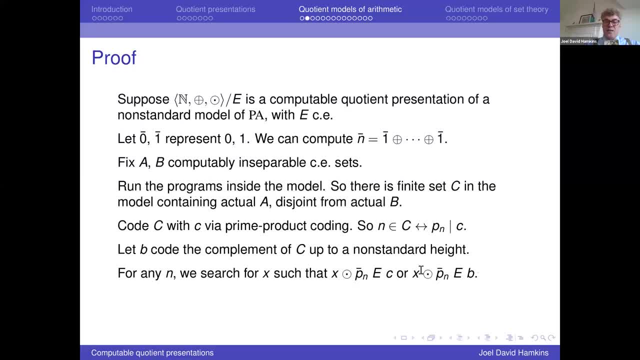 is going to have a solution. So we're going to find a solution one way or the other here, And E with C, E, And so we'll know whether or not Pn is dividing C or is it dividing B, And so in that way we can decide membership. 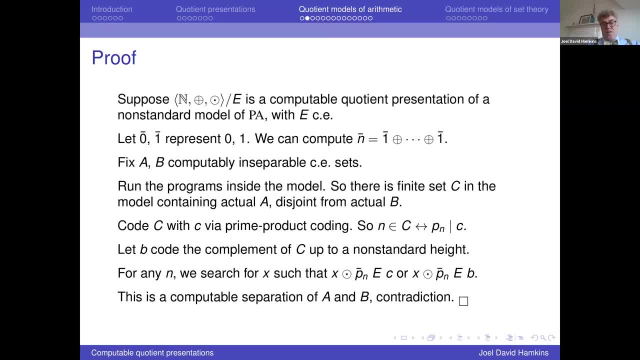 in C for the standard number n. So that's a computable separation because all the elements of A, C is covering A and discerning from B. So all the elements of A are going to be put into the set and none of the elements of B are. 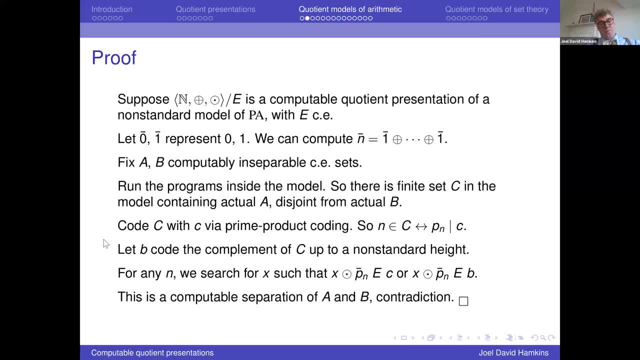 going to be put into the set, And so we found a computable separation. Joel, Can I ask a question? Sure, please, In this setup at the top of the page, so you have this plus with a circle and times with a circle are computable recursive functions, right. 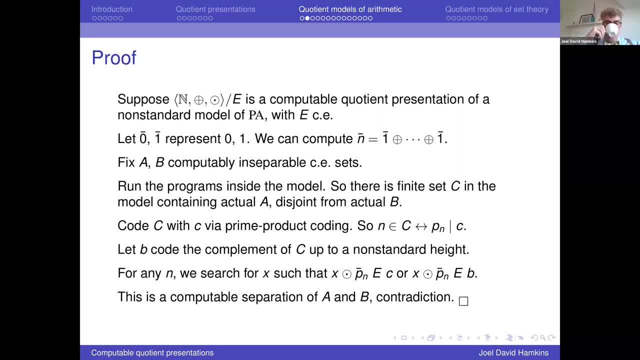 Yes, And are you requiring that they are invariant under E? It should be a congruence, So they don't have to be well defined with respect to E. That's much, much too strong. They only have to be a congruence. 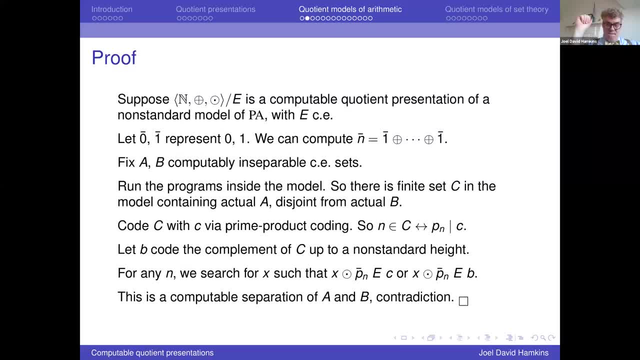 A congruence. So E respects those operations. Yeah, Otherwise the quotient doesn't make sense, right? Well, you could say there is. Yeah, you're right. So that's what I mean. OK, fine, Thank you. 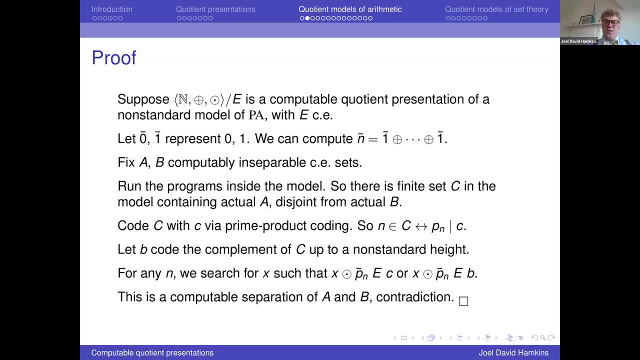 Yeah, Thank you. So yeah, OK, thank you. I don't insist that it's well defined with respect to E, Because that's almost never true when you define with. A lot of people misuse the word well defined when they really should be saying congruence. 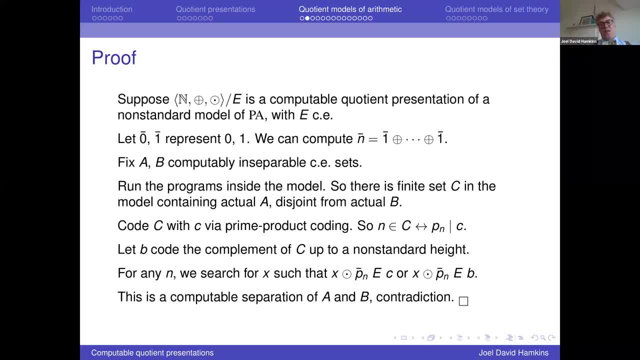 I think in many applications of mathematics, when you define a function depending on an equivalence relation, But you Like, for example, modular arithmetic- is addition well defined. mod 5?? No, because the answer that you get when you add mod 5 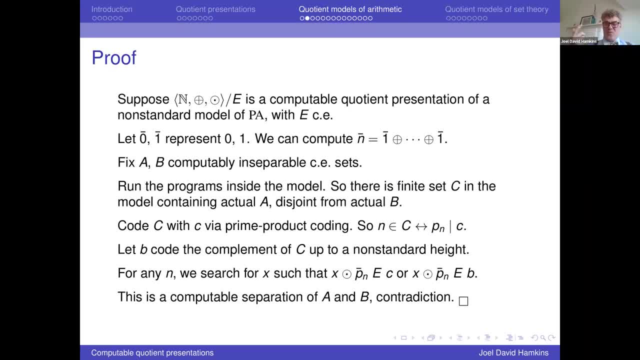 is not the same, It's just equivalent, mod 5.. So that's the difference between being well defined and being a congruence, And so here we only have the weaker notion. We only need the weaker notion- But that's what you should mean- in order to form that quotient. 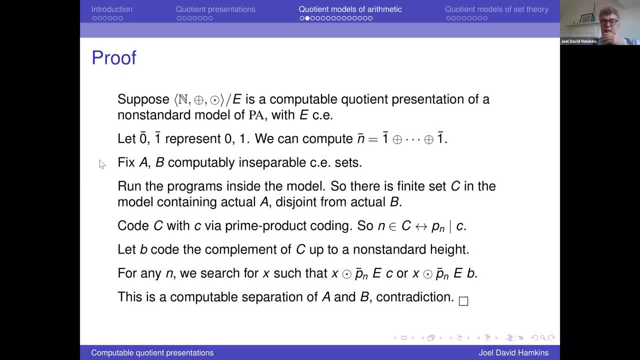 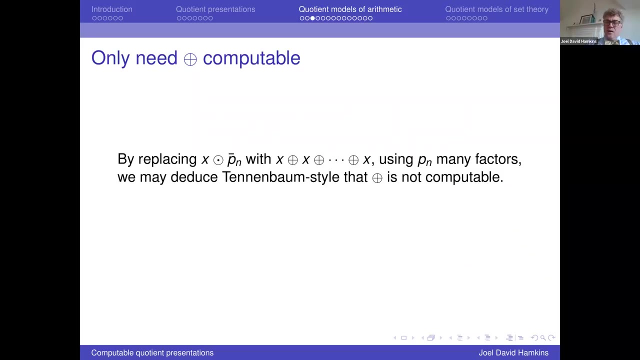 Thank you. OK, so right. OK, so that's a proof of the quotient version of the Tenenbaum theorem in the case when equivalence is CE. So that's proving Buckhider's first conjecture. OK, so in fact we can weaken the hypotheses in a similar way. 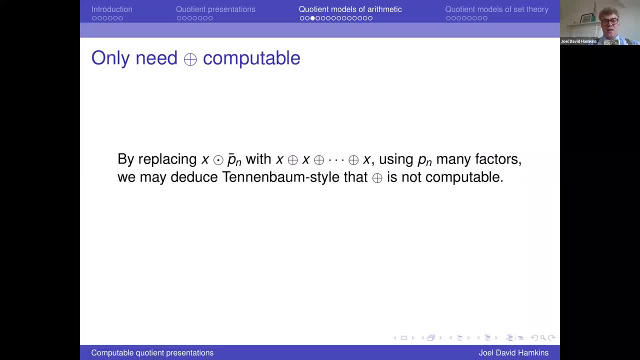 So Tenenbaum proved actually a stronger thing than what I had said earlier, Namely, he proved that you can't even have a nonstandard model of arithmetic such that the plus is computable, let alone time. So the way I stated it, we assumed both of them. 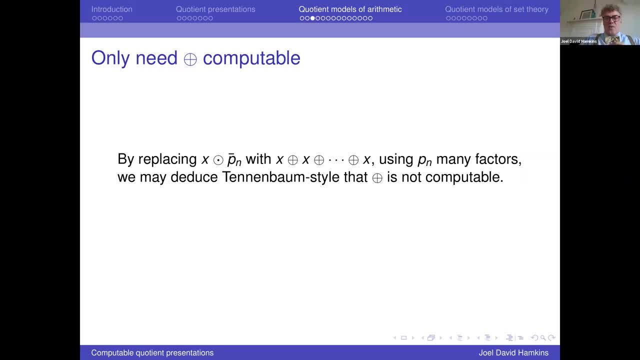 were computable, But in fact Tenenbaum proved neither one of them can be computable. And we can get that stronger result here. And it's very simple, because what we needed in the proof was to multiply x by Pn bar. 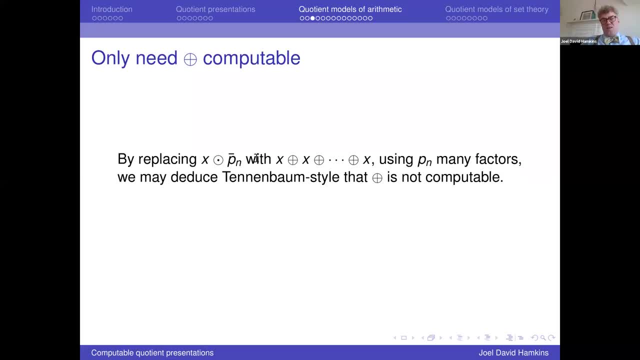 But this was a standard finite number, And so we could have just added instead. We didn't need multiplication to do the decoding, We only needed addition, And so what we can deduce is that there's no quotient presentation whose plus is computable. 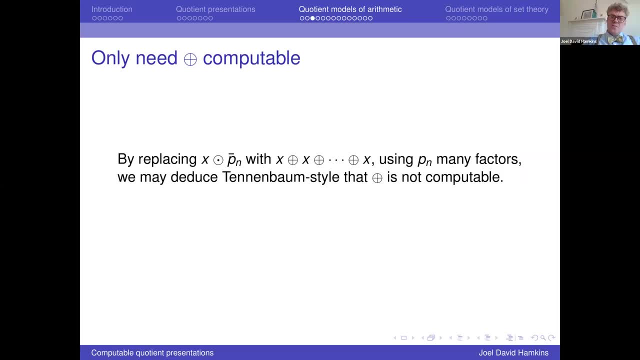 and whose equivalence relation is CE. that gives you a nonstandard model. And you can also do a similar thing with the multiplication, only if you just push all the coding into the exponents instead of with the primes themselves, And then when you're multiplying, of course, 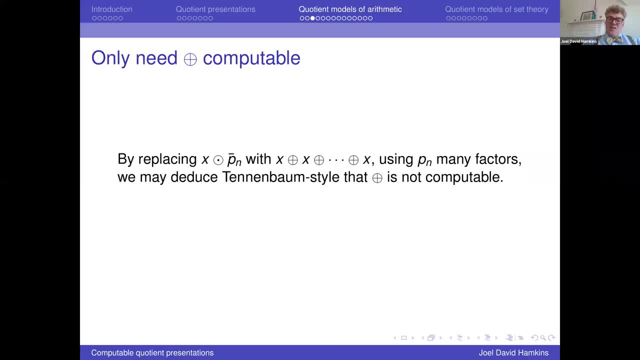 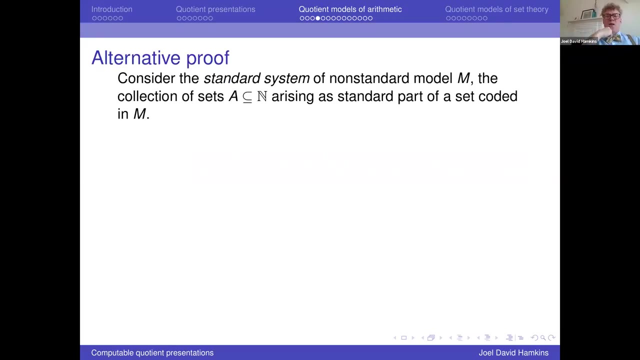 exponentiation turns multiplication into addition, And so we can do the same argument, assuming only that times is computable and we never need to talk about plus. OK, right, So let me give now an alternative proof of that theorem, using what's called the standard system of a nonstandard model. 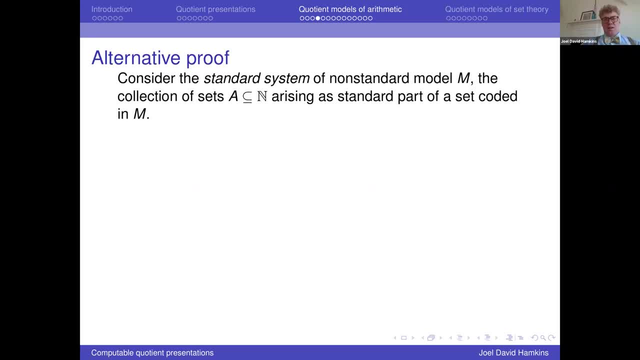 When you have a nonstandard model of arithmetic, then you can look at, say, all the definable sets with parameters, definable with parameters, And those definable sets have a certain trace on the standard numbers, And so we take all those sets of standard numbers. 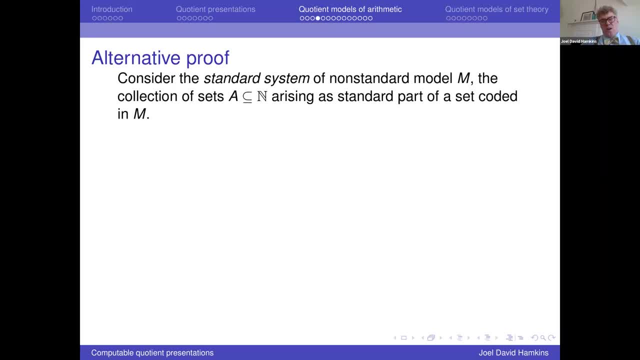 That's the standard system. It's the trace of all the definable sets on the standard part, And that's equivalent, of course, because these are models of arithmetic. If I have a definable set, maybe it's infinite inside the model. 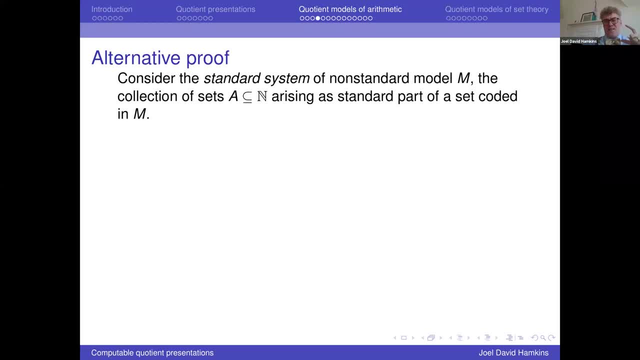 But I can chop it off And now inside the model I've got a finite set And that finite set can be coded inside the model. So you can define the model with prime power coding or whatever coding you want, And so you could also equivalently. 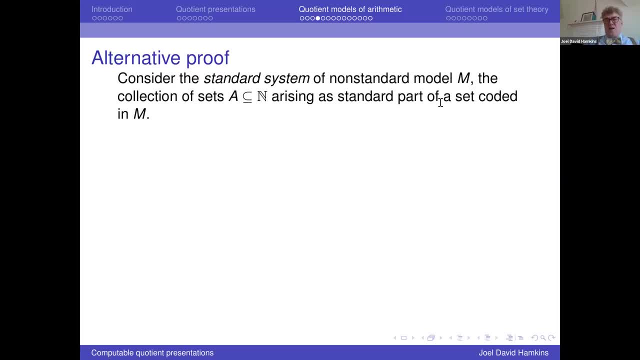 define the standard system as the collection of sets that arise as a coded set in the model in that way. OK, so for example, we could do the coding- This is the coding that we used before- Namely for any number c in the model. 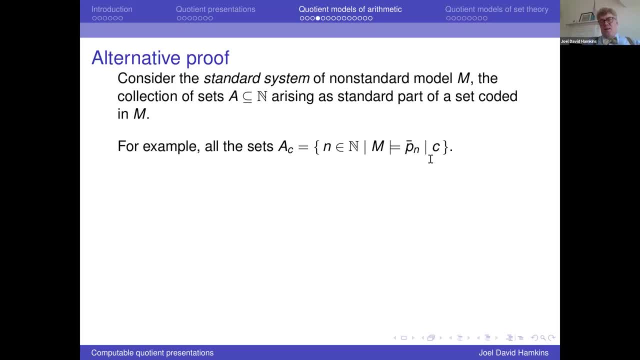 we can look at the set of n so that the n prime divides c. That's a set of natural numbers, and that's what it means to be coded in the model. Now, of course, what I'm saying is that if I just throw all these sets together, 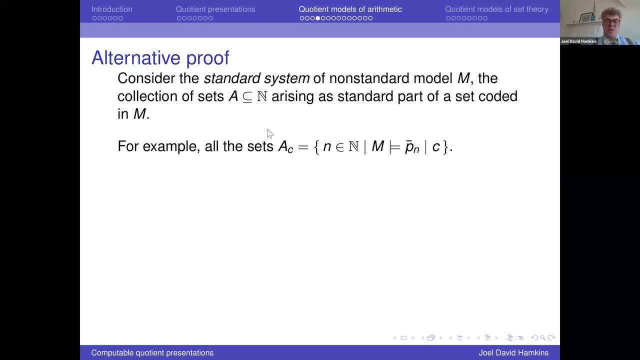 that's the standard system. So any set that you can define at all, of course, is going to be coded this way, because you can chop it off inside the model at some non-standard point, And then the trace will be the same. OK, that's the standard system. 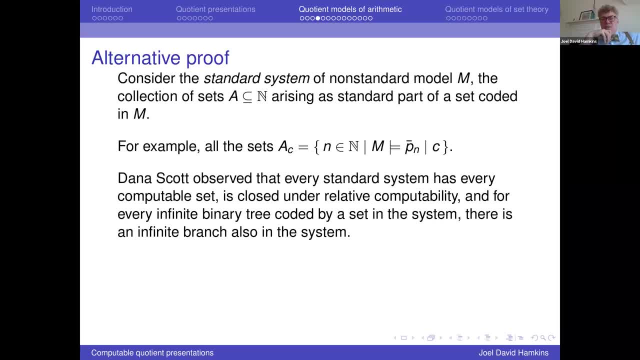 And Dana Scott had observed a couple of things about these standard systems. Namely, every standard system of course has all the computable sets in it And it's closed under relative. So if I have a set in the standard system, 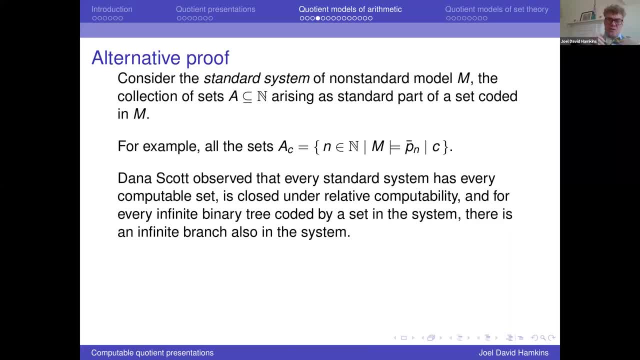 then anything I can compute from that should also be in. So it's downward closed in the Turing degree. And furthermore, whenever I have an infinite binary tree that's coded in the standard system, then it will also have an infinite branch through that tree. 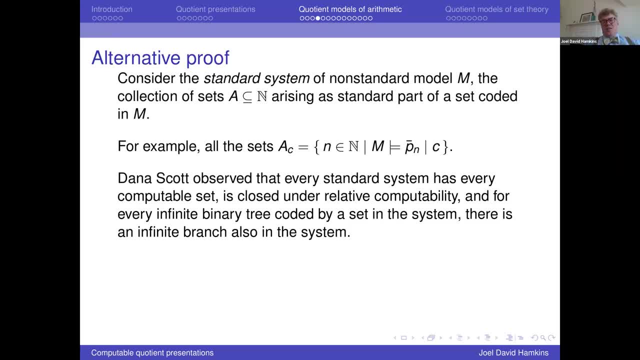 Because if the model thinks that I have a number coding a set that's an infinite tree, then by overspill it will be an infinite tree to some non-standard height, And so the model will be able to do that. So the model will have a branch that 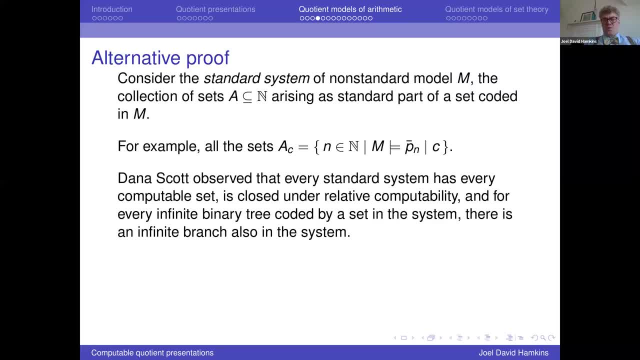 reaches into the non-standard part, And that will be an infinite branch through the actual tree. So basically, that's showing that the standard system is fulfilling the weak Koenig's lemma, And he proved, let's see. so Scott proved that in fact those properties 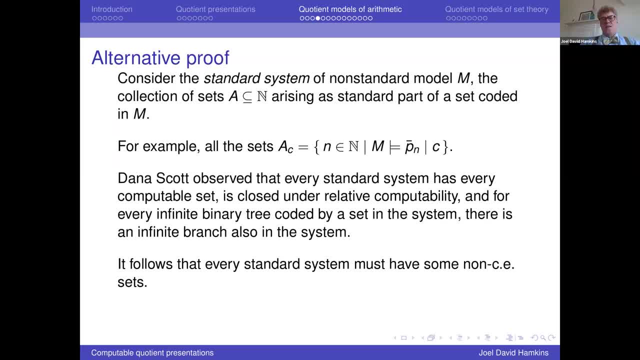 characterize the standard systems in the countable case. If I have a countable family of sets of natural numbers and they contain every computable set and they're closed under relative computability and they have the property that whenever there's a tree coded by one of those sets, 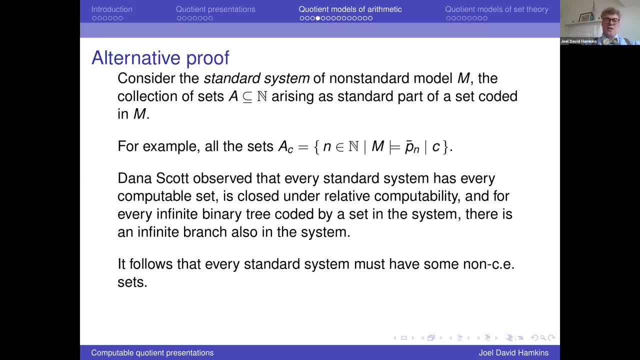 then there's a branch through that tree coded by another one of those sets, then it is the standard system of a model of PA and also the standard system of a model of set theory, and so on. So in the countable case it's an if and only if. 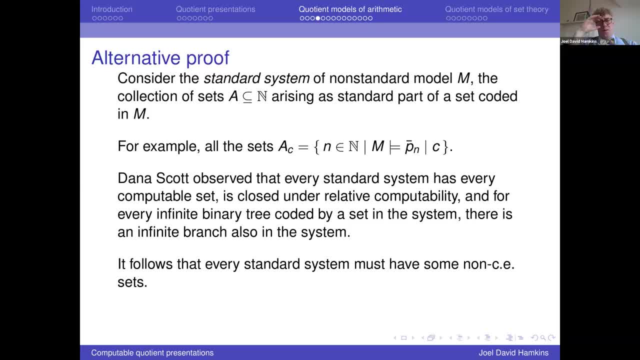 characterization And that was later extended to the case of omega 1-sized family. So every omega 1-sized Scott set- these are called Scott sets with these properties- is the standard system of a model of PA. So under the continuum hypothesis, 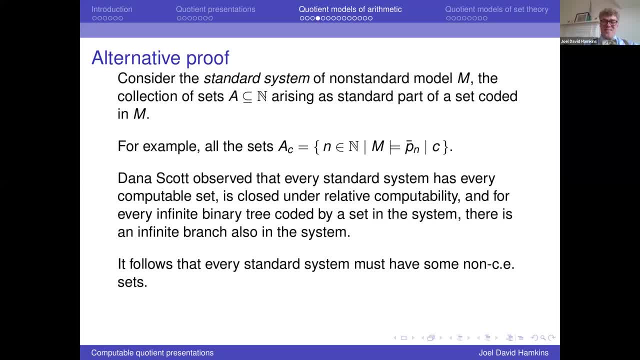 that's a complete characterization, But we don't know. unfortunately it's still open. If the continuum hypothesis fails, then we don't know whether every Scott set is the standard system of a model of PA or not. OK, what I want to take from this: 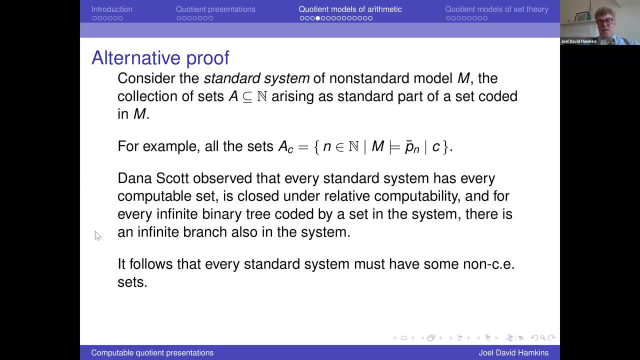 though, is that every standard system must have some, say, non-CE sets. The branches through the computable trees might not be computable, OK, but the argument we gave before showed that if the equivalence relation is CE, then every set in the standard system. 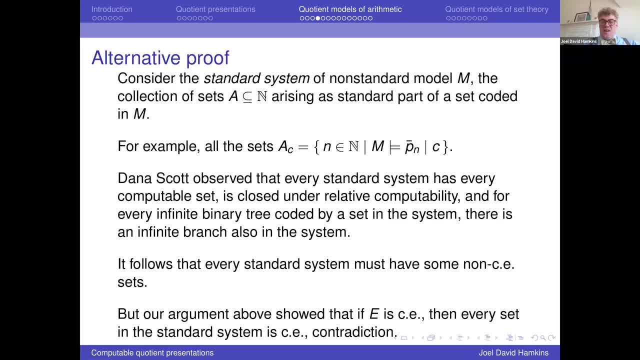 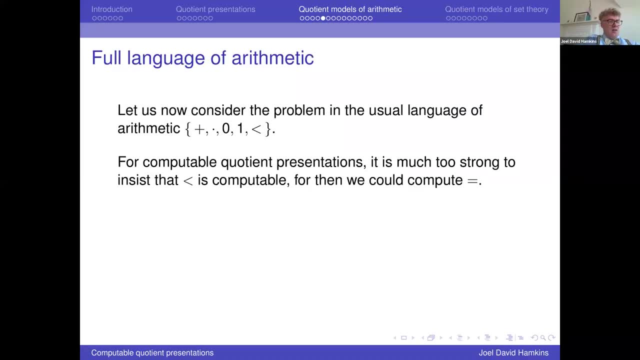 is CE because we described how to do the decoding And so we can enumerate the members of any coded set, And that's a contradiction to the fact that the standard system must have non-computable elements. OK, So let's now go to the full language of arithmetic. 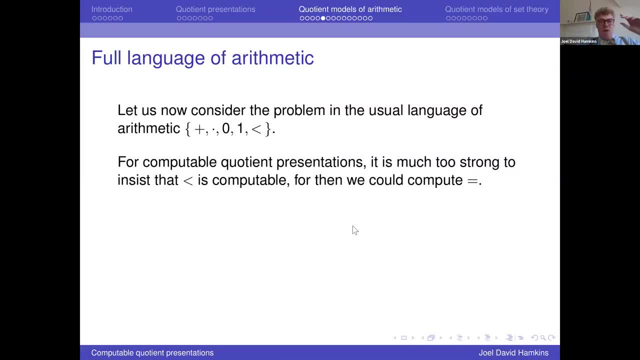 I want to make sure. oh, let's see what am I doing on time. OK, So now let's add the rest of the less than relation. Now, of course it's much too strong if we insist that less than is computable. 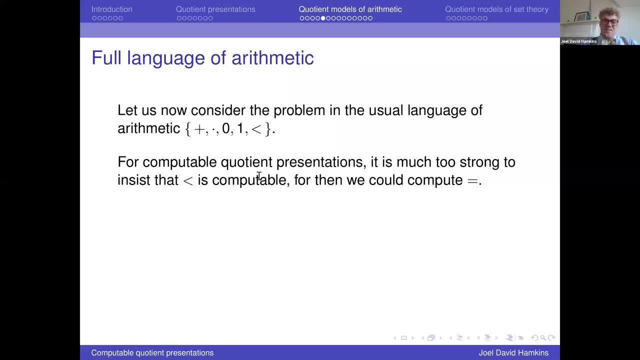 because then we could compute equality. If less than is computable, then to be equal just means that neither one is less than the other, And so if I could compute less than, then I could compute equality, And so I'm not really doing a quotient. 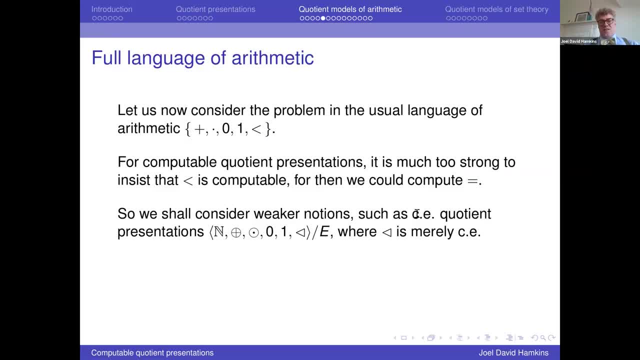 So we really want to look at weaker notions such as CE quotient, where the less than relation is just the CE relation instead of fully computable. And also I want to look at the reflexive order. Of course, these are by expressive. 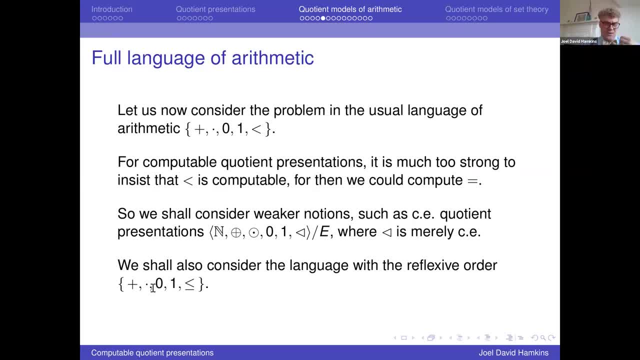 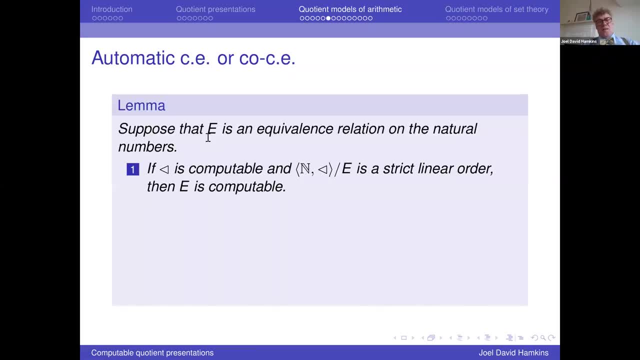 We don't need the order at all, But it's natural. Both of them I find natural OK. there's some easy lemma here: If you have an equivalence relation and you have a computable relation whose quotient is a strict linear order like less than, then E is computable. 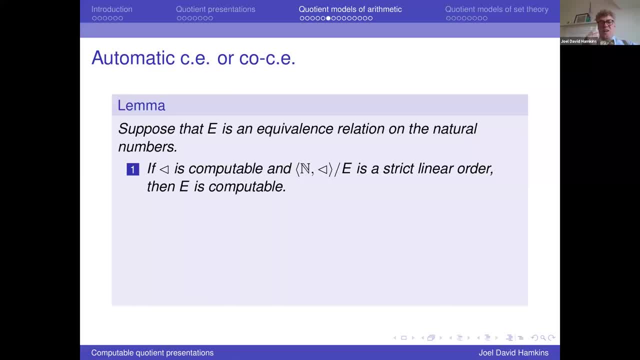 That's just what we said before, Because to be equal means that neither one is strictly less than the other, So if this is computable, then the equality is going to be computed. If the relation is only CE, though, and the quotient is a strict linear order, 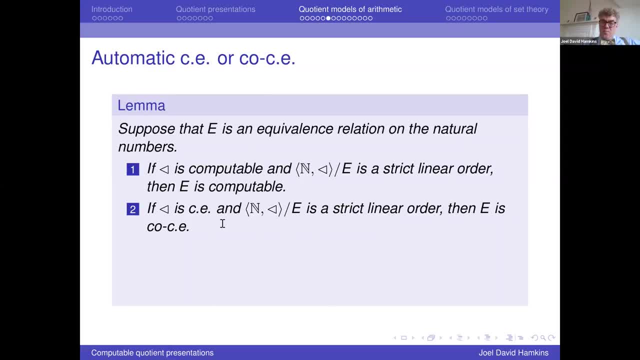 then, automatically, E is going to be cos E, Because to be unequal means one of them is less than the other, which is something that you'll be able to observe. And then, in the reflexive case, if you have a reflexive order whose quotient is a linear order, 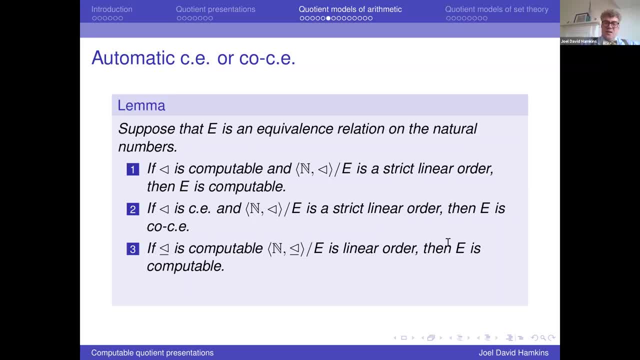 meaning reflexive, transitive and anisometric. then E again has to be computable. And that's just because things are equal if, and only if, they're less or equal to each other. And that's just the way it is. 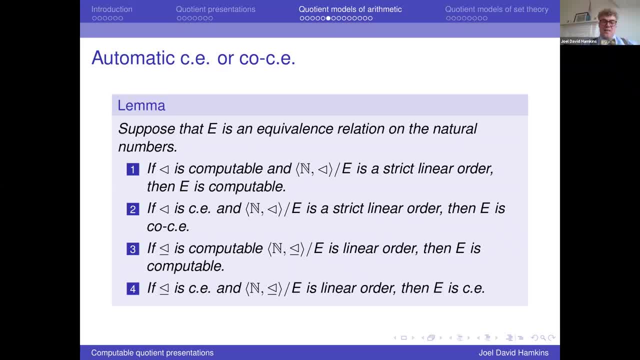 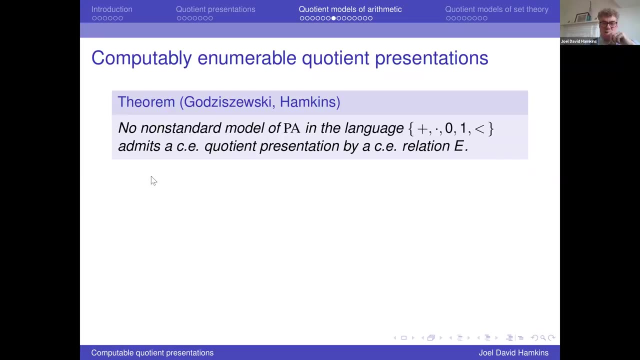 OK, And that's what you can compute. And similarly, if the reflexive order is only CE, then E will have to be CE, OK. So this kind of easy reasoning basically answers the question in the case with the orders. So you can't have a nonstandard model of PA in the language. 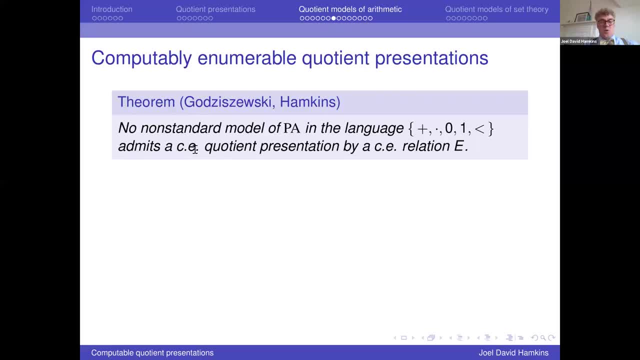 with the order that has a computably enumerable- not only just a computable quotient presentation, but a CE quotient presentation by a CE relation. And the reason is that if this quotient was a nonstandard model and E was CE, well by the lemma it would have to also be co-CE. 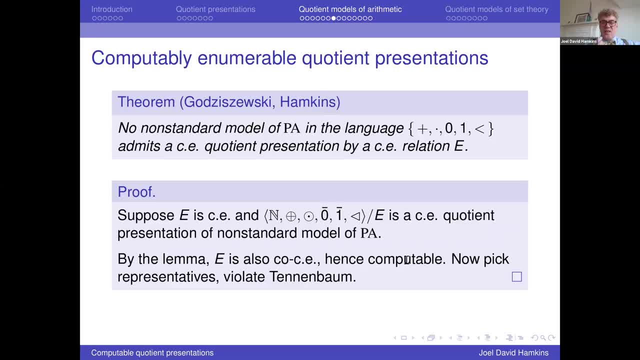 And so it would have to be computable And so we could pick representatives. If E is computable, then we can pick representatives And we'll have basically a computable presentation, which would violate Tenenbaum. So of course there's an alternative. 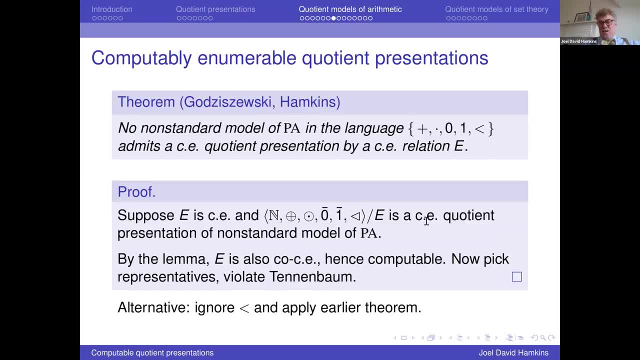 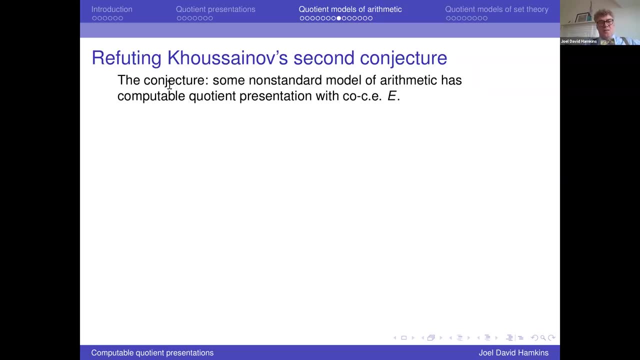 It's just ignoring the quotient, Ignore the relation, And then we're talking about a CE quotient presentation of a functional model, which we already handled with the first theorem. OK, So let's go to the second conjecture. So Kosanoff had conjectured that there's 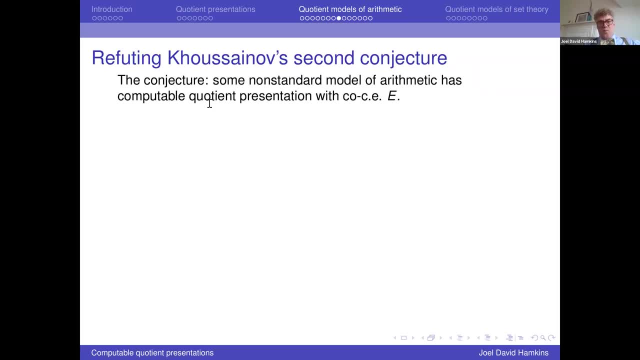 some nonstandard model with a computable quotient presentation using co-CE equivalence relation. So let's refute that And we can find out that there is no nonstandard model in the language, in this language, even for the CE quotient presentation. OK, 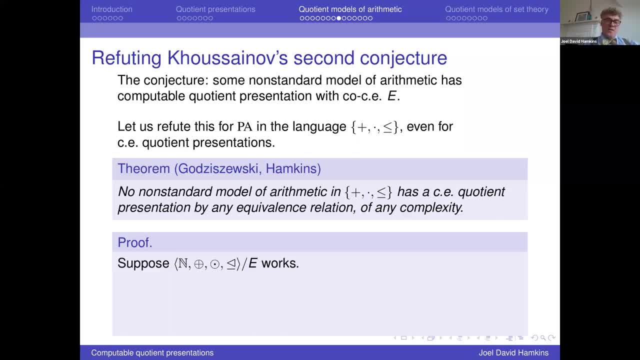 So suppose we had a CE quotient presentation. In fact you can't do it by an equivalence relation of any complexity whatsoever, And the reason is: well, suppose that you had a quotient like this, where this was a CE structure. So the operations are computable. 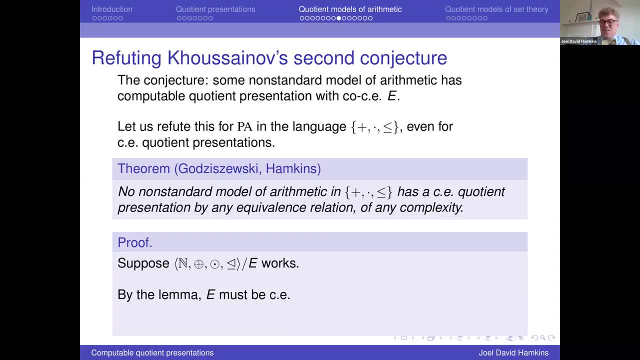 It has to be CE, because that sort of trivial reasoning shows there's this automatic computability of equality when you have an order, And so it's just the first theorem again, because the equivalence relation must be CE in this case. OK, So you can't do it in the reflexive order version. 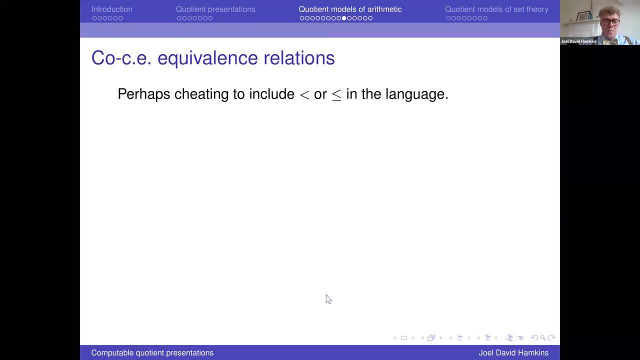 by any equivalence relation because it would have to be CE. OK. So it's maybe cheating. OK To put the order into the language. I think that's how I view it. It's cheating to look at quotient presentations when you have an order because it's too tightly connected. 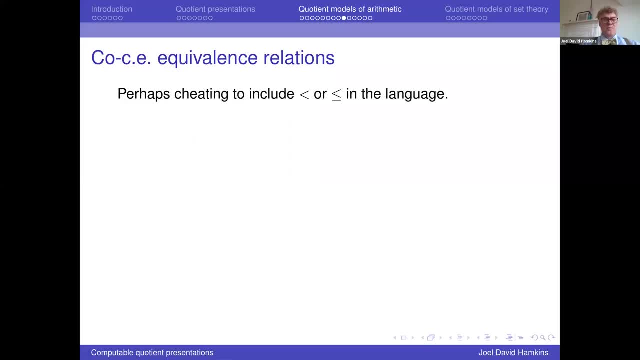 with equality And it just reduces to the computable case too easily. So let's go back to the functional language And I want to prove a version of the second conjecture. I'm going to refute the second conjecture in the case of true arithmetic. 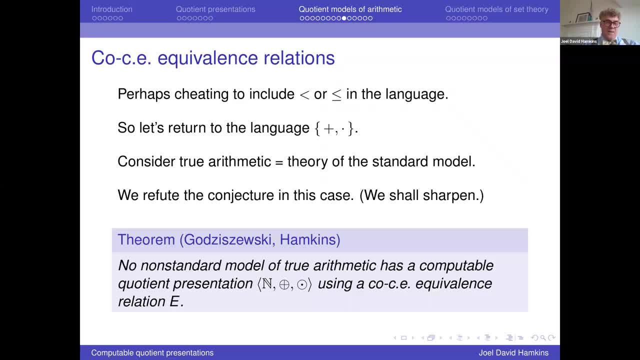 So you cannot. Yes, So there's no non-centered model of true arithmetic. We're going to sharpen this. We don't need all of true arithmetic, but just very little actually. But let's just first do it for true arithmetic. You can't have a computable quotient presentation using 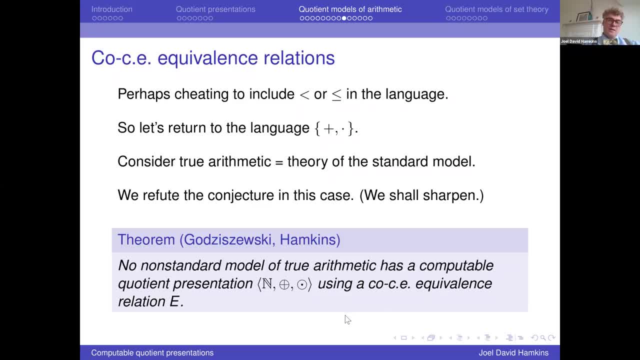 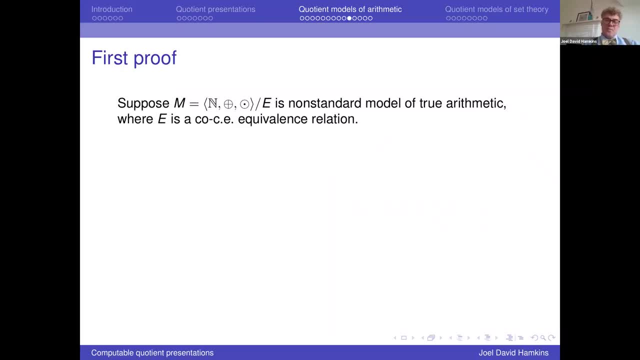 a co-CE equivalence relation. So suppose you had such a model by a co-CE equivalence relation. So let 1 bar be the number that's representing the number 1 inside the model. OK, So by adding 1 plus 1 plus 1, we can represent any number n. 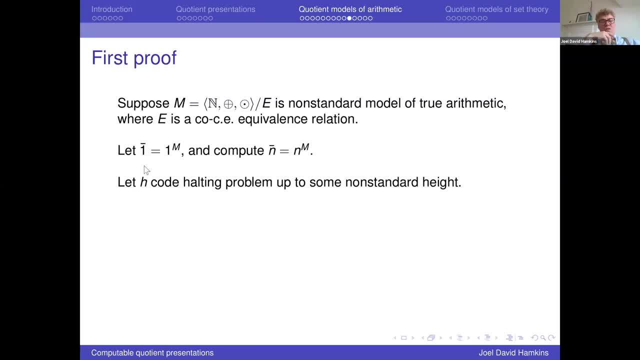 That way we can compute And let H code the halting problem up to some non-standard height. It's a model of true arithmetic, so it agrees with us about which programs halt. So therefore the actual halting problem is coded in the model up to some non-standard height. 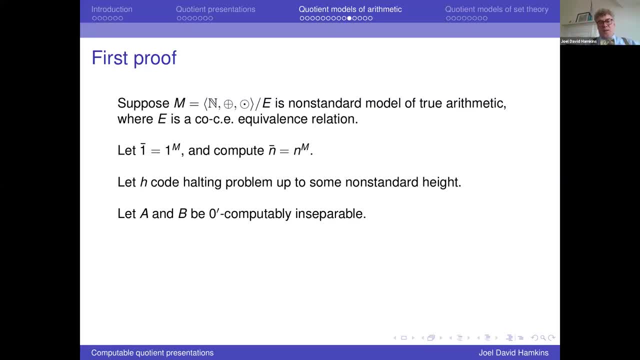 And now let A and B not just be computably inseparable, but let them be computably inseparable with respect to an oracle for 0 jump. OK, So we ask for 0 jump computably inseparable sets, So they're both innumerable, with 0 jump as an oracle. 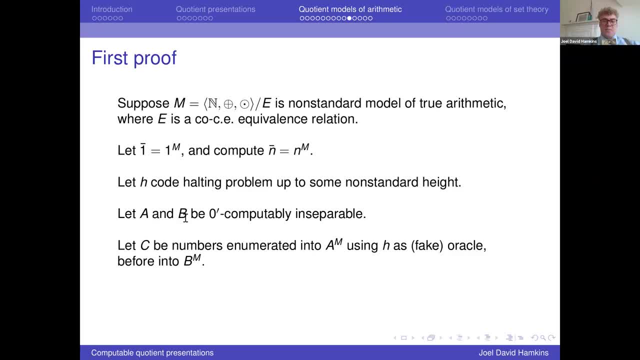 and they're not 0 jump separable. And then we can use this fake 0 jump. It's the non-standard version of 0 jump up to some non-standard height. The model thinks it's finite, but it agrees with the actual 0 jump. 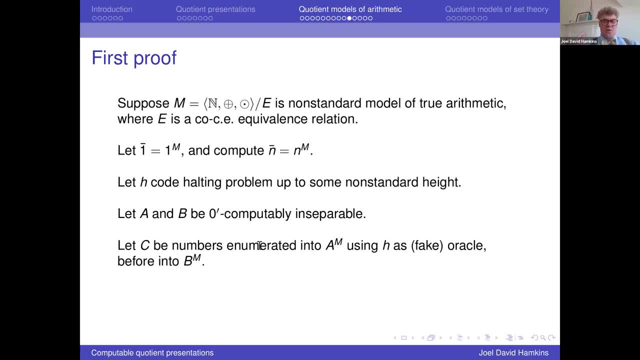 on the standard numbers, And so I can use that as an oracle for computation and I can let C be the numbers that are put into A using that fake oracle before they're put into B. So this is going to be a separating set. 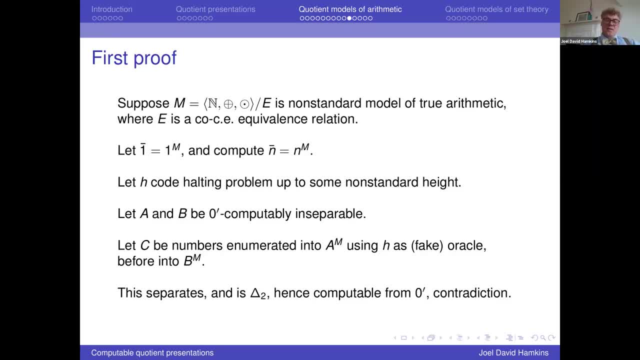 And if you think about it, it has complexity. delta 2, because with 0 jump as an oracle, we can compute E, And what we're asking for is a solution of this divisibility equation by a co-CE relation. So that's a sigma 2 statement and the negation is also. 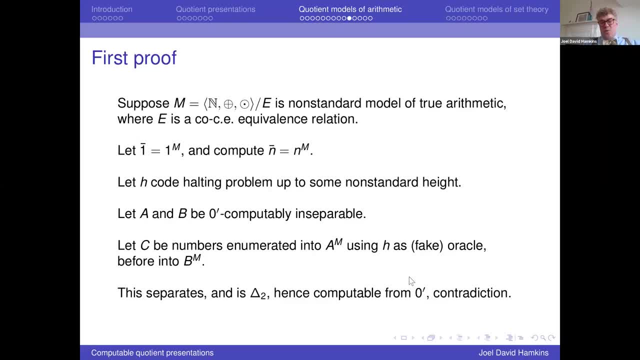 a sigma 2 statement. So it's delta 2, and therefore computable from the actual 0 jump. And that's a contradiction because it's a separating set. but these were supposed to be 0 jump, computably inseparable. OK. 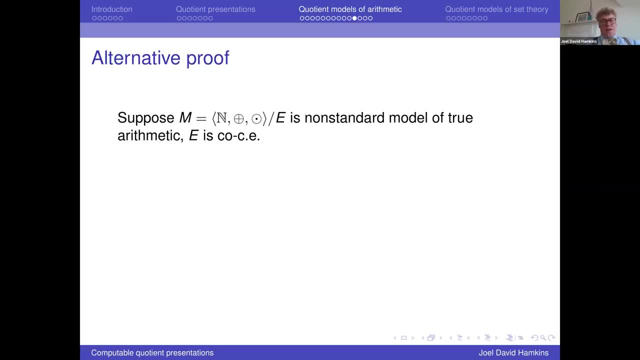 Let me give a different proof now. Suppose I had a computable model by a co-CE equivalence relation of true arithmetic. Therefore 0 jump is in the standard system because the model agrees with us about which programs hold. So it computes 0 jump correctly. 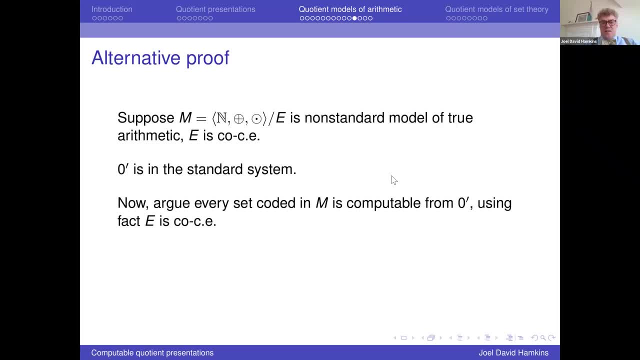 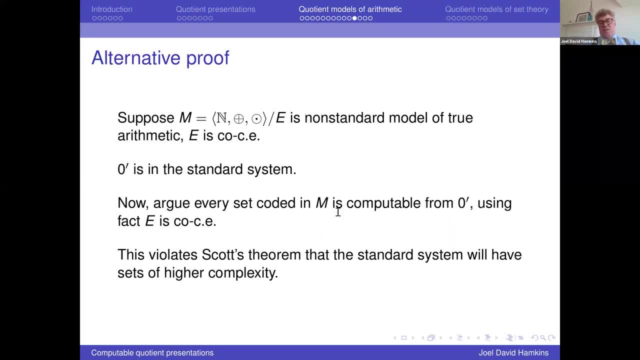 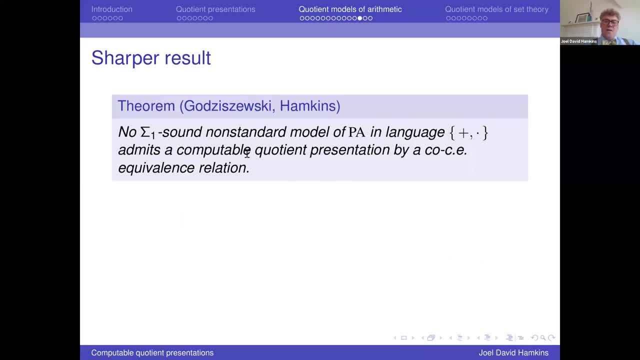 that aren't computable from 0 jump. But every set, we argued, is computable from 0 jump. So that's a contradiction. OK, So in fact we don't need true arithmetic at all. All we need is much, much less. 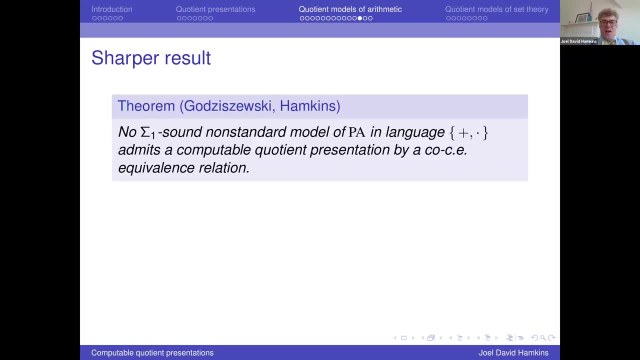 Sigma 1 sound is enough. So the model should simply have the same sigma 1 truths that we do in the standard model. So you can't have a sigma 1 sound non-signal. So you can't have a sigma 1 sound non-standard model of PA. 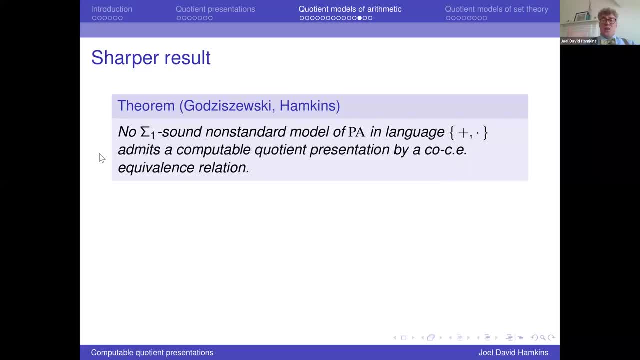 that has a computable quotient presentation by a co-CE equivalent equation. So this is refuting the second conjecture. in the case of sigma 1, sound models. OK, Well, we already showed. it's enough if 0 jump is in the standard system. 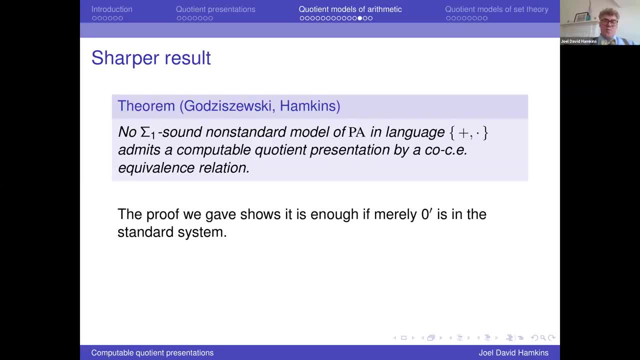 And if it's sigma 1 sound, then it's going to be correct about which programs fault, And so the 0 jump is going to be in the standard system. But in fact we can prove the theorem even just knowing that 0 jump is in the standard system. 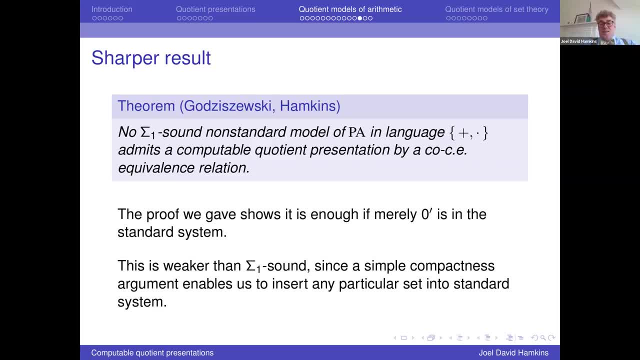 And that's weaker than 0 jump. It's weaker than sigma 1 sound, because we can put 0 jump into the standard system of any model that we want. I mean any theory. by compactness argument, you can always put 0 jump into the standard system. 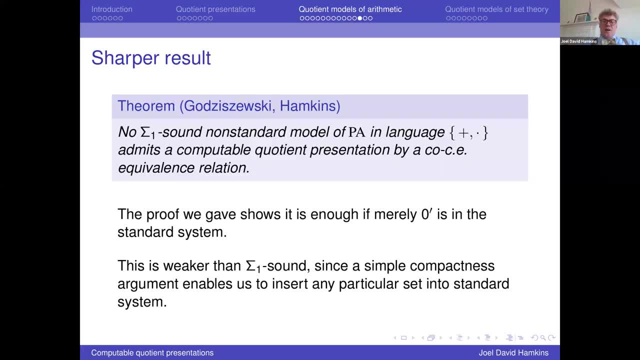 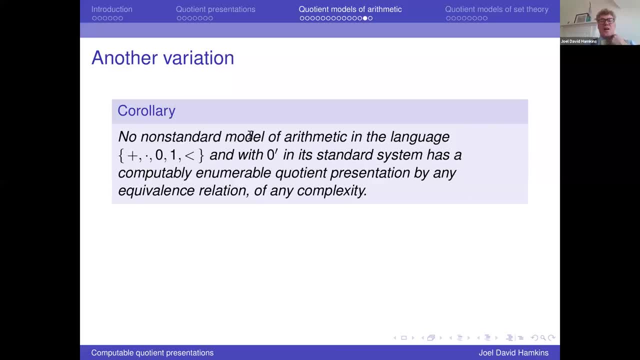 of a model of that, And for any extension of PA there's a model of it that has 0, jump in the standard system by a compactness argument. So what we really proved is that no non-standard model of arithmetic, we don't need less than here. 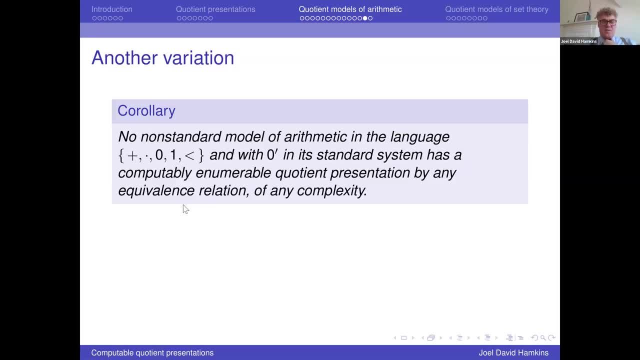 Let's see: Oh, this is computably enumerable quotient presentation. So the relation less than is CE by a relation of any complexity. And the reason is that if this is CE and we take the quotient, then E has to be co-CE. 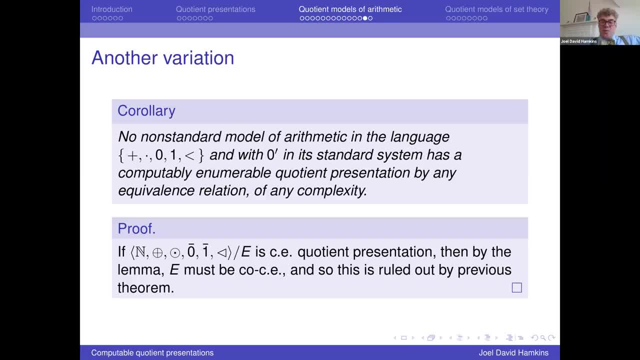 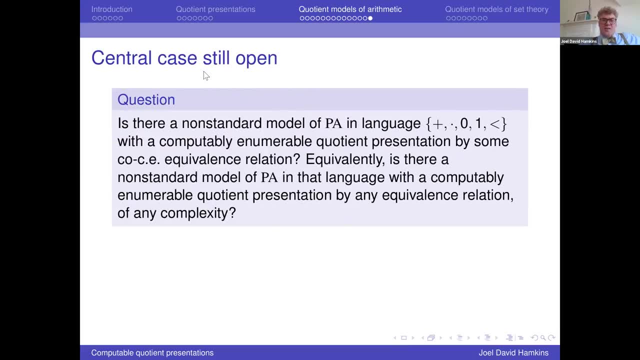 But then we already ruled out that case when 0 jump is in the standard system. OK, So the central case. So the second question, though, really remains open. So can you have a non-standard model of PA in the usual language with less than which? 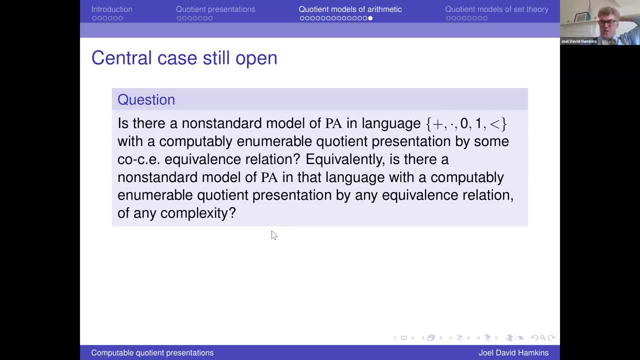 has a CE quotient presentation by some co-CE equivalent solution. We had to make these extra assumptions, either that it was sigma 1 sound or that 0 jump was in the standard system, or we had to use less or equal instead of less than. 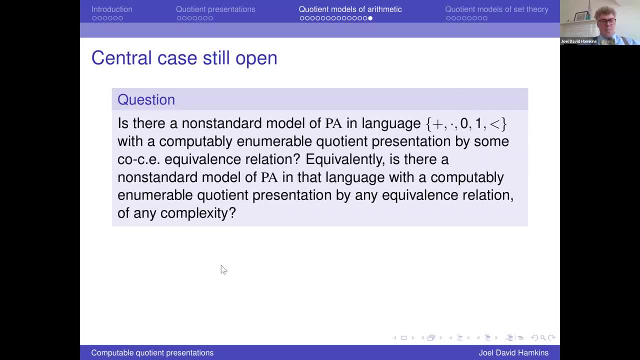 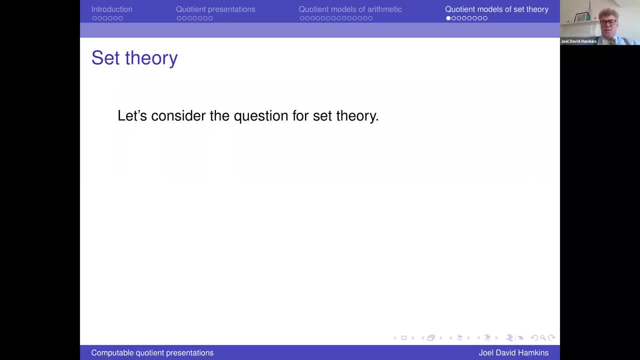 And so we don't technically know the answer to this question. OK, So let's go on To set theory. what time is it? Oh my gosh. OK, Let's see. So is it OK if I go a little bit over the 45 minutes, or maybe I'll? 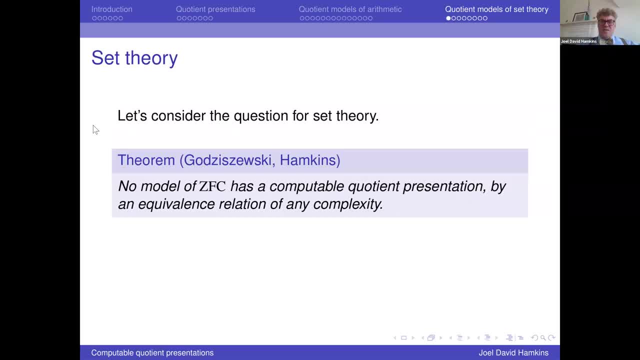 Yes, the home time is one hour. We can have less questions, OK. OK, so the main theorem is that no model of ZFC has a computable quotient presentation by an equivalent solution of any complexity. So in set theory we get the full. 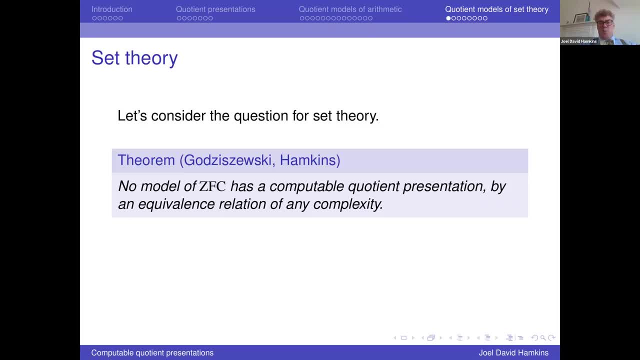 We get the full Result. You just can't have computable quotient presentations of models of set theory by an equivalent solution of any complexity. So in other words, there's no computable relation epsilon and the equivalent solution E, such that the quotient is a model of ZFC. 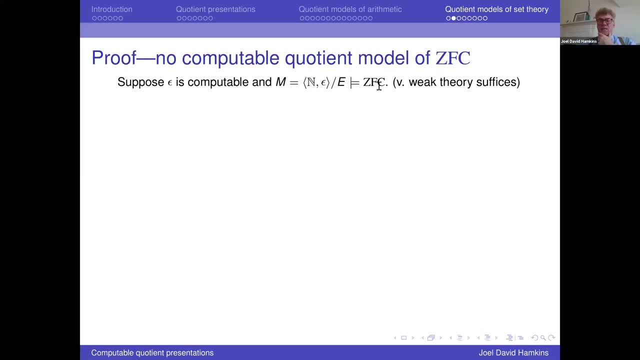 OK, so let's describe the proof. Suppose that you had it. We don't need ZFC. Very, very weak theory is enough. Now there's this annoying thing: that proof involves this really detailed consideration of what's going on with coding and interpretation in set. 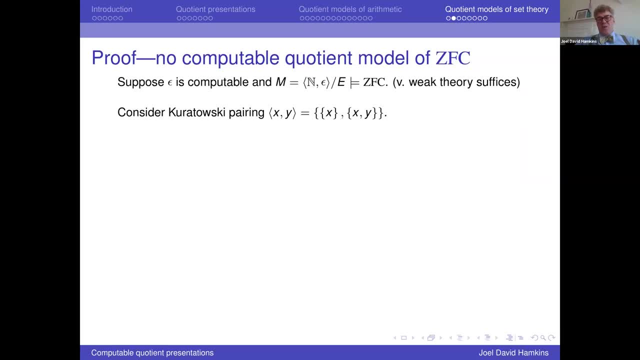 theory, because if all you have is the epsilon relation, you can't compute what's the number 7 or what's the number 65. That's basically impossible to compute. We can prove. So we're going to need these parameters, So I'm going to fix a number in the model that's representing. 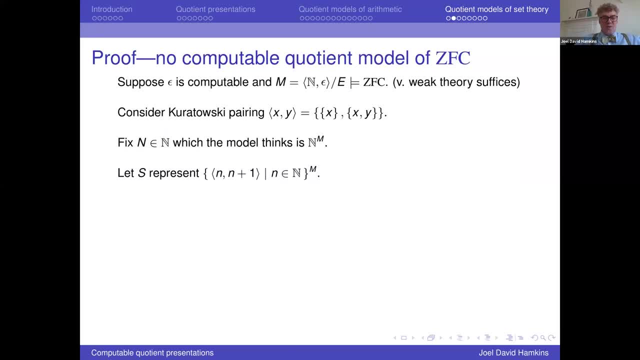 the set of natural numbers. It's a model of set theory, so it has a set of natural numbers And it has a set that represents the success, The successor function on the natural numbers And it has a set that represents the set of singletons. 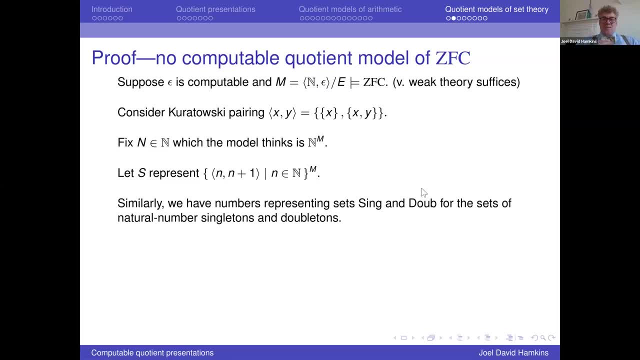 of natural numbers and another set that represents the set of doubletons, I mean with actually two elements of natural numbers. And now, using all these parameters, I can compute the function that takes a number n to the set that's coding it inside the model. 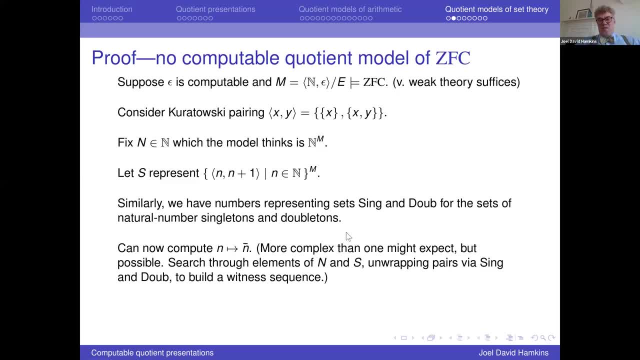 And it's just irritating. It's more complex than you expect, But the way it works is OK. you give it a number n, now we can give ourselves the number 0.. And now, how do we find the number 1?? 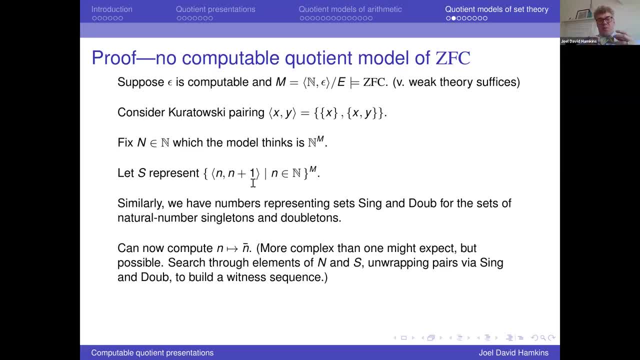 Well, we have the successor function but we can't just apply it because we don't have it as a function. We only have it as this set of elements. But the elements of it are just other sets that happen to be pairs, And the pairs are: this Kertowski pairing thing. 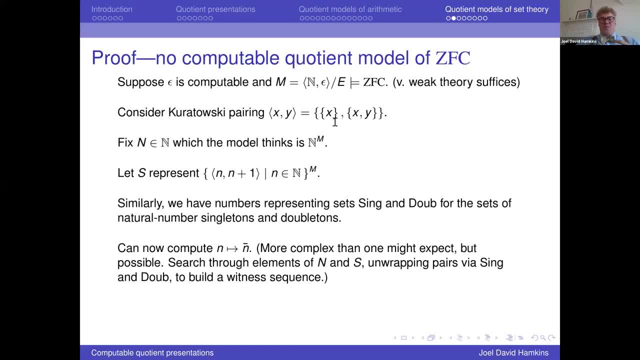 And so the elements of s are themselves sets that have two elements which are themselves, one of which is a singleton and the other of which is a doubleton. And I can recognize which are which using these sets, because if it's an element of sing, then it's a singleton. 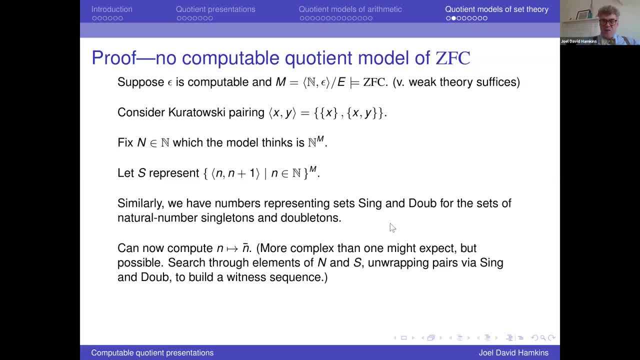 And if it's an element of dub, then it's a doubleton, And then I can look for the sets that are elements of those things and so on, And in this way, unwrapping all that coding, I can find the number 1.. 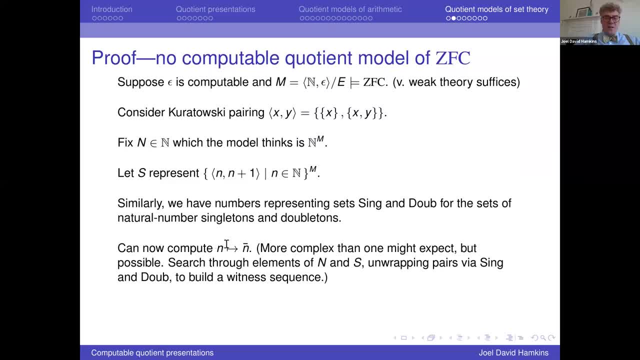 And then I can find the number 2, and so on. I can iterate it. So that's how we can compute the number that represents n for any given n. And now it follows that every set in this standard system is computable, because every set 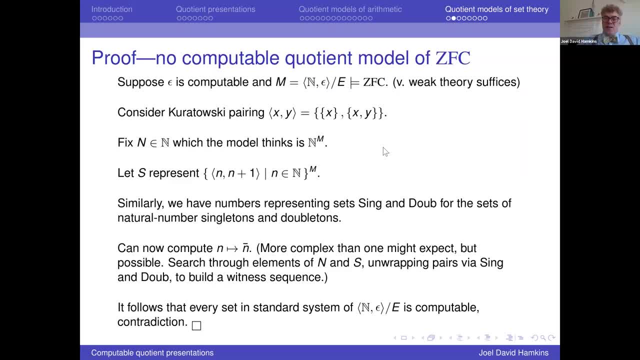 is represented by some number And its elements are represented by the things that are epsilon related to it. And if I can compute this map, then I can compute what are the sets of natural numbers that are represented in the model, that are coded in the model. 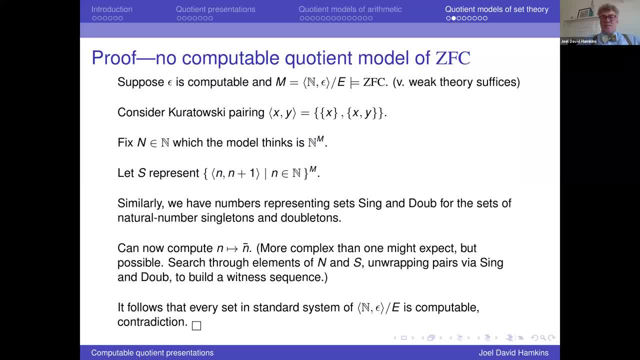 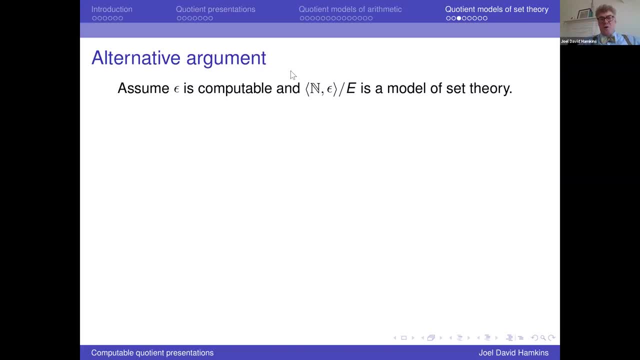 And so every set in the standard system will be computable, and that contradicts Kertowski. OK, here's an alternative argument. Suppose I have a computable relation and the quotient is a model of set theory. Well, by extensionality, two sets. 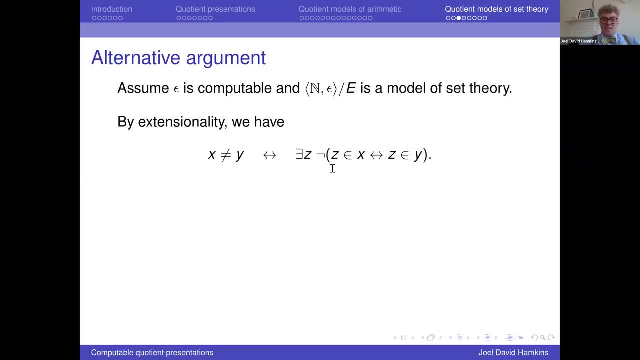 are different, just in case there's some set that's in one of them and not the other. So I can look for that to happen. So that's saying that two sets are inequivalent, just in case there's an existential witness that there's. 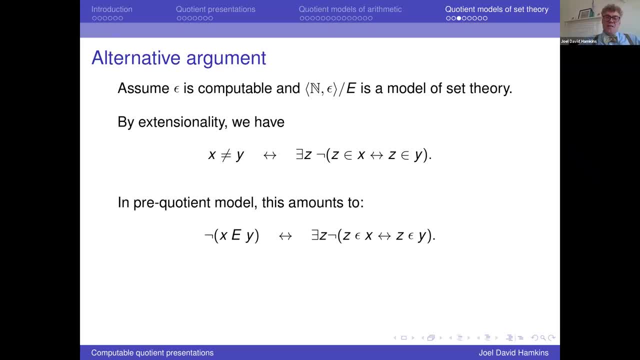 some object that's an element of one and not in the other. So therefore E has to be co-CE. If you have a quotient and it's a model of set theory of extensionality, then E has to be co-CE. 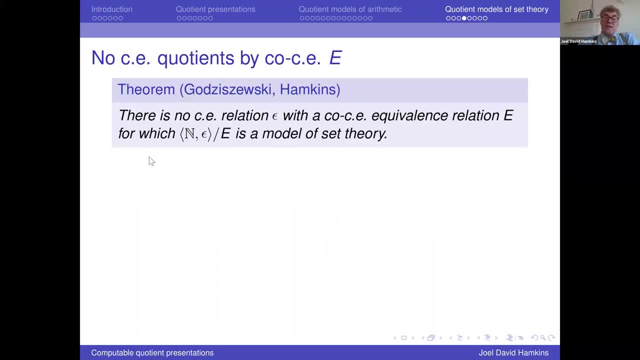 And so we can just argue now from the co-CE case. So let's do that. You can't have a CE relation, even It doesn't even have to be computable, but CE is enough so that it has a co-CE quotient, which is a model of set theory. 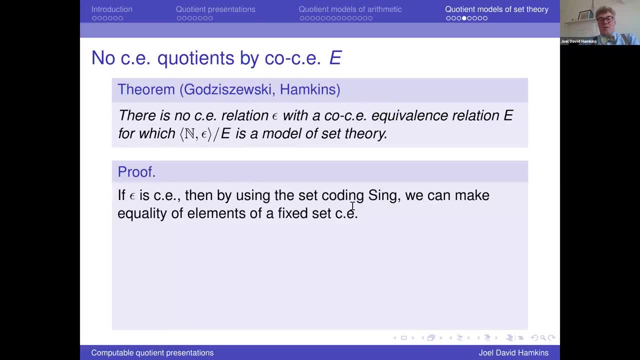 So suppose that we have such a model. Well, we have a number that represents the set of all singletons of natural numbers. So if I have two numbers, if there's a singleton that they're both elements of, then they have to be equivalent. they're equal. 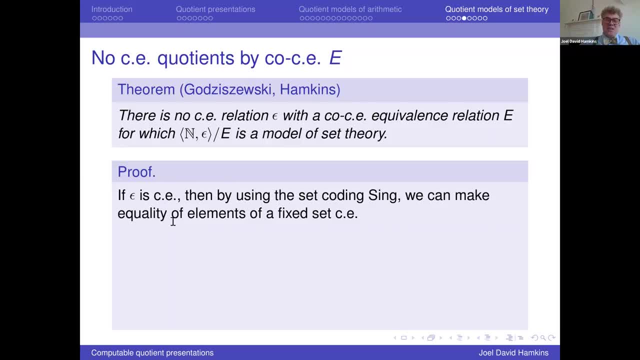 And so that means that equality becomes computable. It's co-CE because the relation was co-CE, but it's also CE because I can look for a singleton that they're both an element of And therefore it's going to be for the numbers that 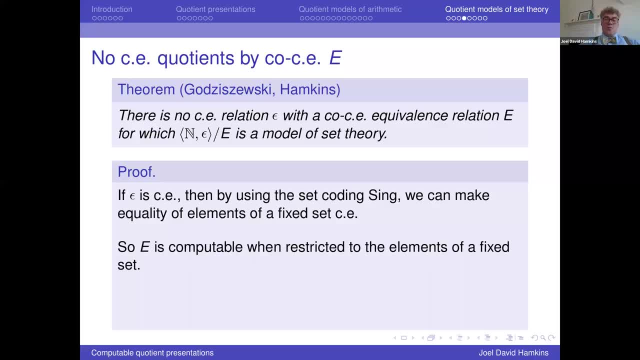 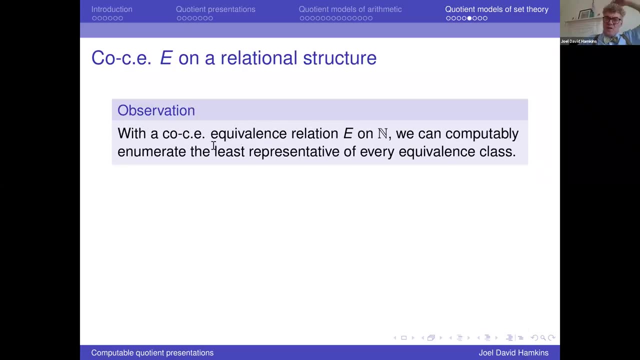 are natural numbers in the model. it's going to be a computable relation And therefore I can reduce to the classical Tenenbaum case, because now I have a computable equivalence relation and I can pick representatives and so on. There's a general observation to make about this co-CE quotient. 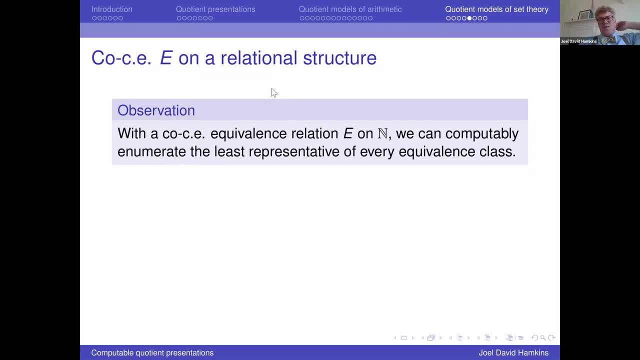 namely when you have a co-CE equivalence relation. it means you can recognize when things are different. If it's co-CE, it means you can get the answers for when things are not equal in the quotient, But therefore you can tell when you have a number that. 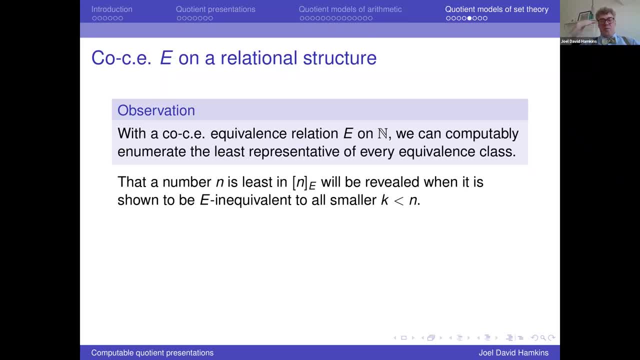 isn't equivalent to any smaller number. that's going to be the minimal element of its equivalence class. We can recognize that. So therefore, when you have a co-CE equivalence relation, you can enumerate the set of minimal representatives from each class. 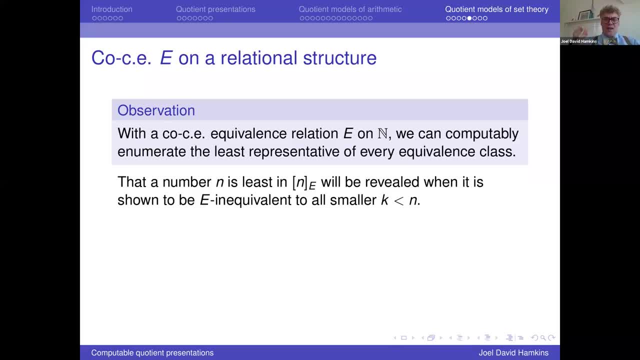 So in a purely relational language, it means that you can reduce to a computable presentation because you can pick. So if you have a computable quotient presentation by a co-CE relation, then you can build a computable presentation by using those minimal representatives. 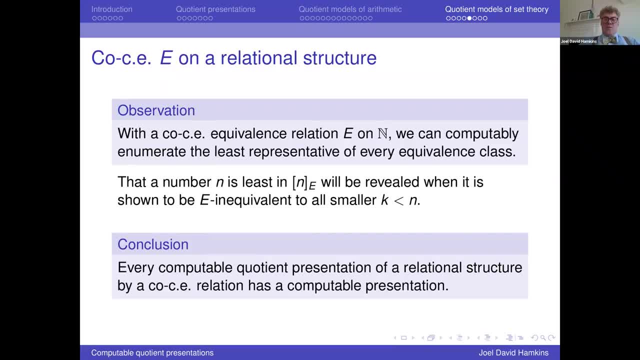 It doesn't work when you have functions in the language, for precisely the reason that Anand brought up earlier, namely that if I have functions in the language, then having the set of minimal representatives isn't good enough, because when I apply the function to those things, I might not be still a minimal representative. 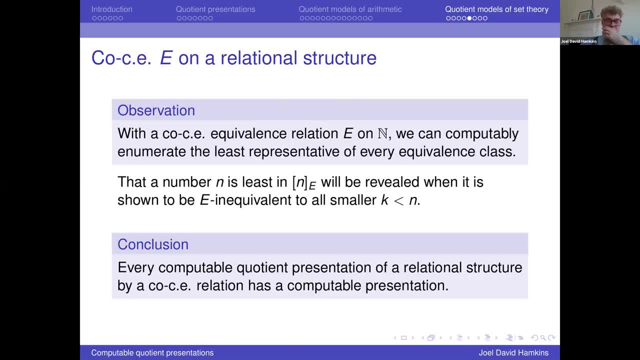 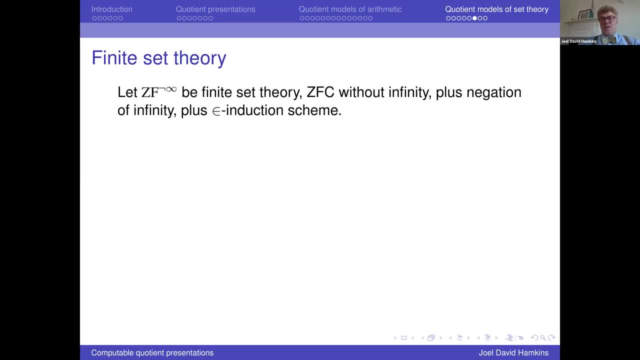 and I won't know which ones it's equal to, And so it doesn't work with functions in the language. And then, lastly, let me just mention quickly, you can handle the case of finite set theory. So why don't I just skip this, since I'm over time? 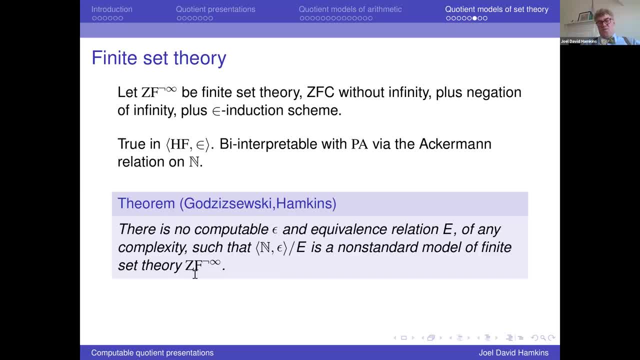 and I'll just say it quickly: If you work in finite set theory, where you don't have any infinite sets but only finite ones, it's equivalent to PA basically. Then we can also prove it. So OK, and that's the co-CE case for finite set theory. 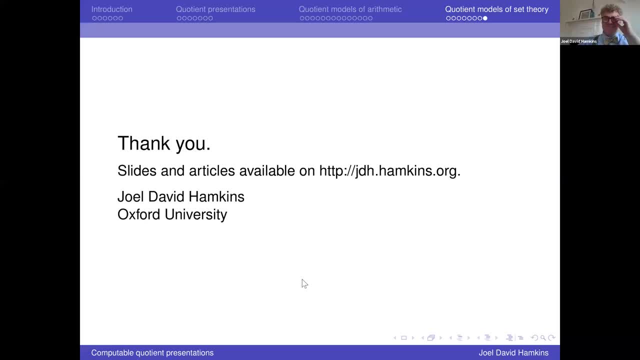 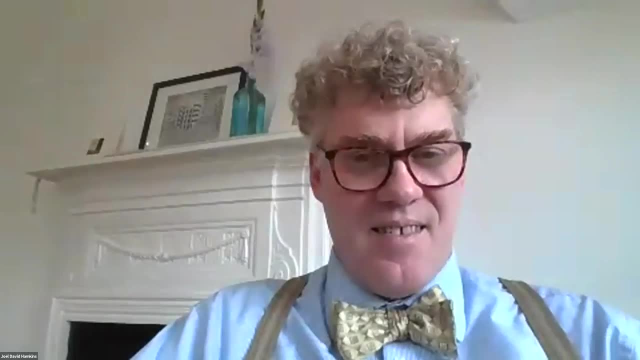 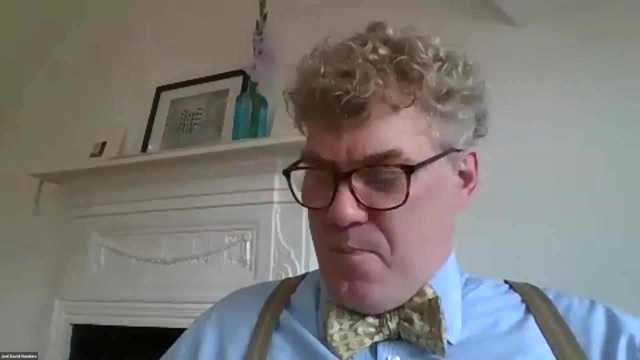 So thank you very much. That's it. Oh, thank you. Professor Anand, Do you have a question? I had a question. This is a silly question. So at the end of the talk you said that ZFC doesn't have. 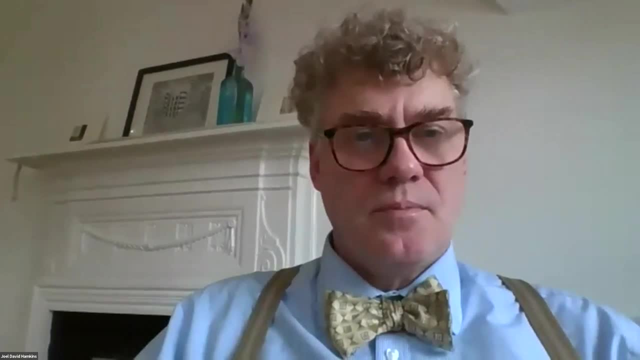 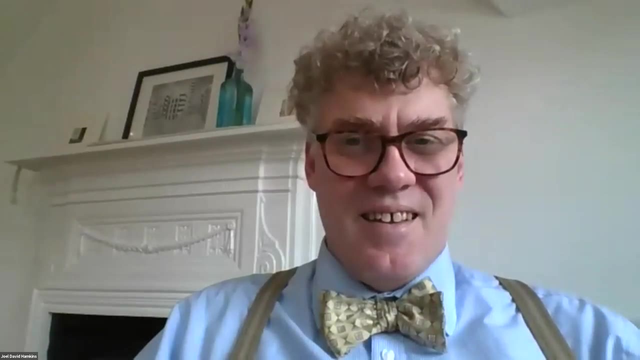 any computable model quotient present in the set theory, And I'm sorry, I forgot the terms. Earlier. there was a thing that every theory, consistent theory, has a computable quotient. Was it only for functional languages or something? Yes, exactly. 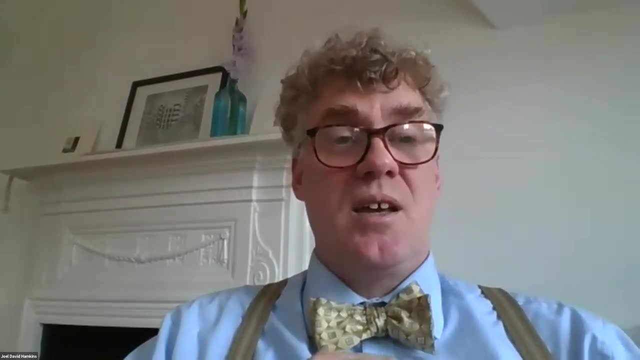 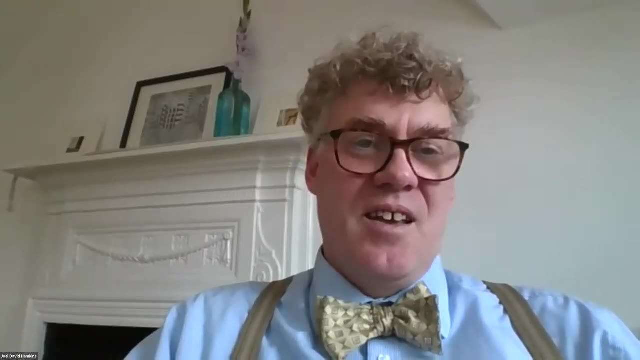 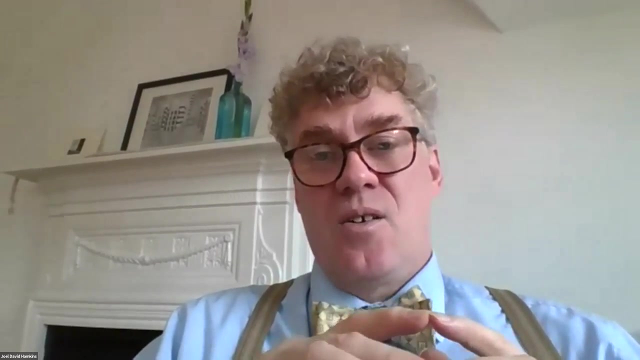 So the theorem that I mentioned earlier was only for functional languages, because we took the quotient of the term algebra, But we don't have a term algebra. in set theory There's no functions at all. In fact, the previous theorem needed there to be only functions and no relations at all. 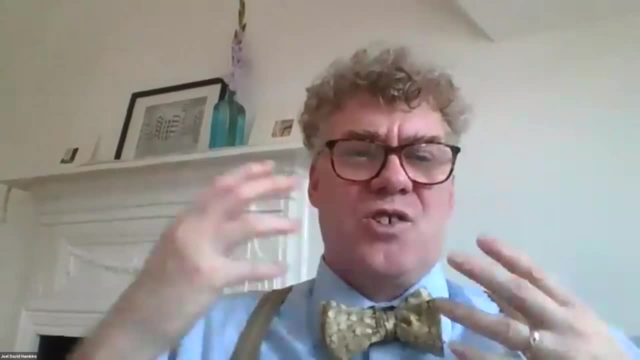 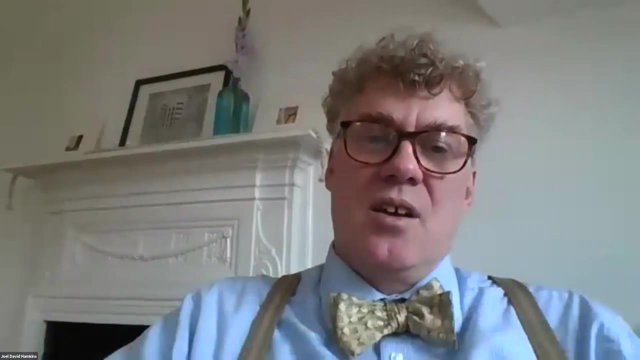 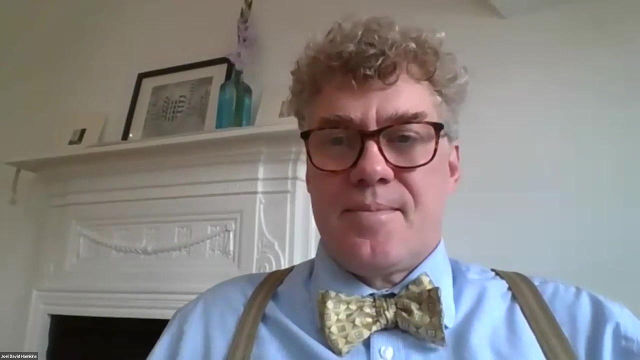 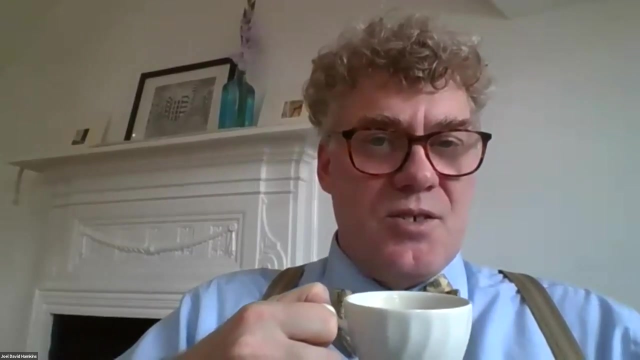 So if you had something like this and you had a set theory, if you had some sort of functional language approach to set theory, then you could talk about the term algebra and hope to get a version in that language. OK, Thanks, I have a question. 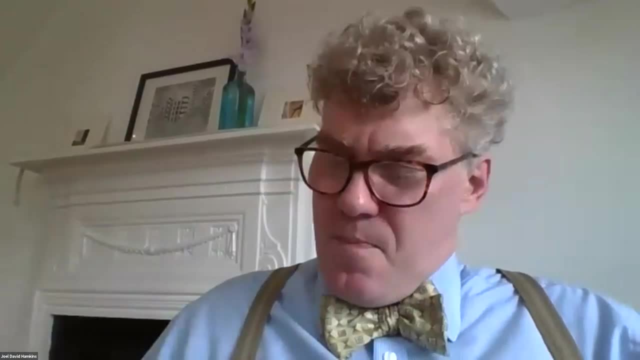 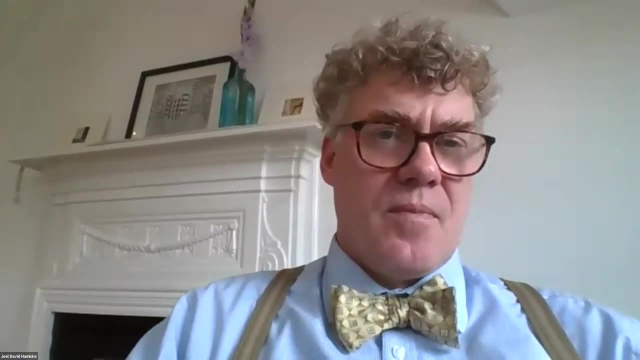 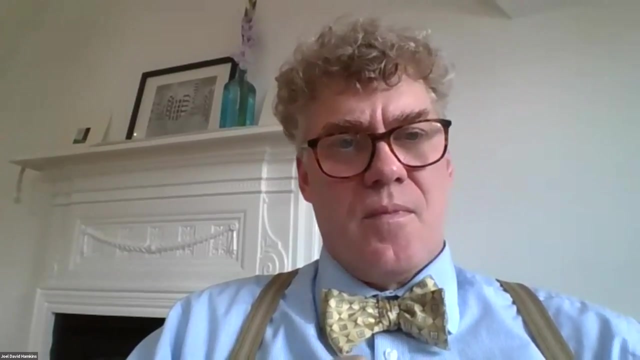 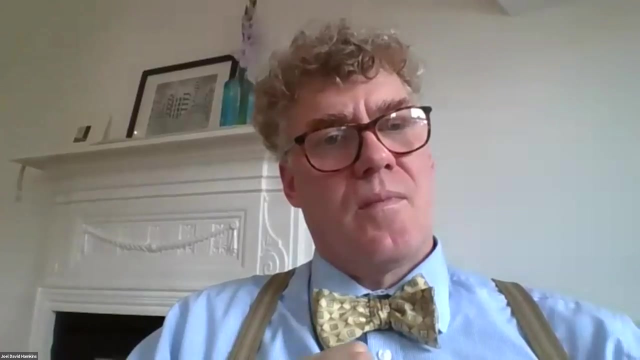 Sure Is it. one could also consider: maybe it's equivalent. It's considered natural numbers and equivalence relation. On n mod e, you have the structure of a non-standard model of arithmetic And you make some conditions on the equivalence relation and on the pre-images in n to the 3 of the graphs of plus. 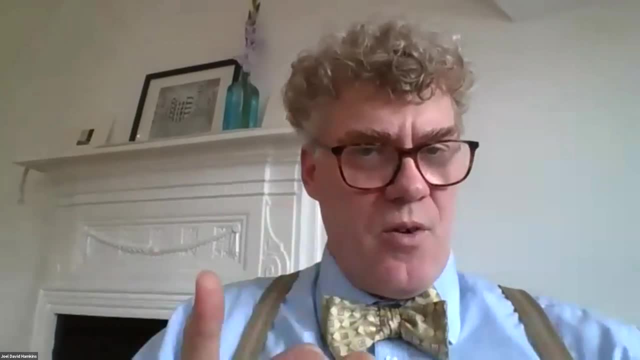 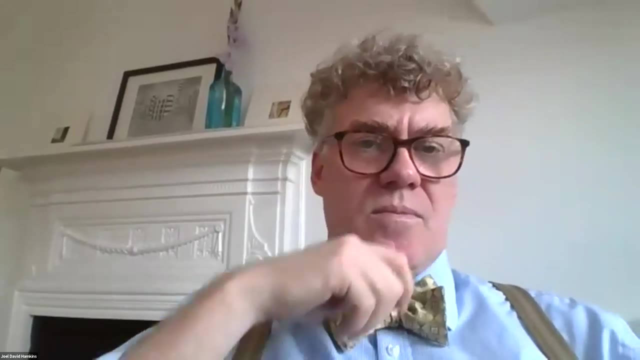 and times. Well. so you want to replace the functions with their graphs and go relational. You just take the function on the quotient, take its graph and just take the pre-images. You take the pre-image of that graph in n cubed. 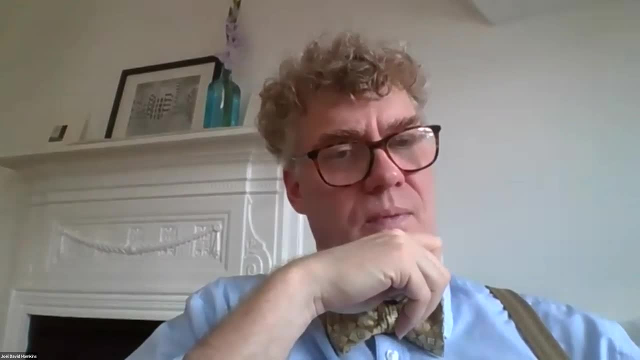 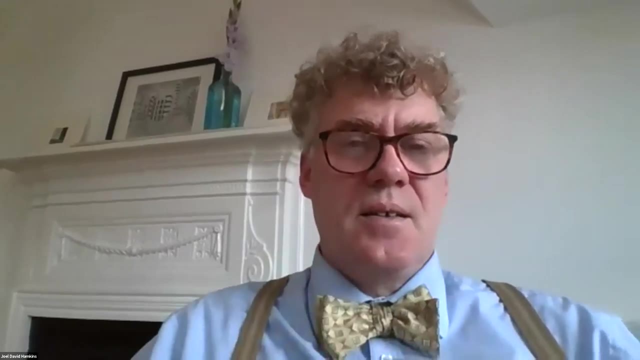 And you require something about that having some complexity, And you make some requirements that both e and those two graphs have some level of complexity. OK, Now, is that kind of set up equivalent to what you're doing, Or is it more general? 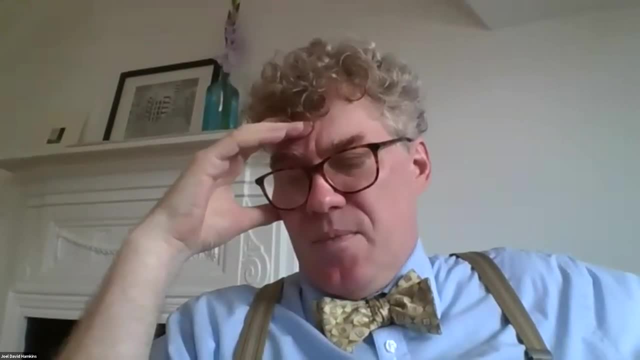 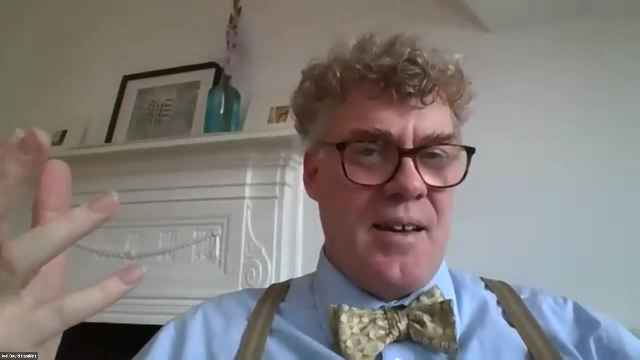 Let's see. Well, it depends. OK, if you have less than or less than or equal in the language also, then you get this kind of automatic decidability. Yeah, So you're going to have to look at that lemma for equality, that lemma, those four cases. 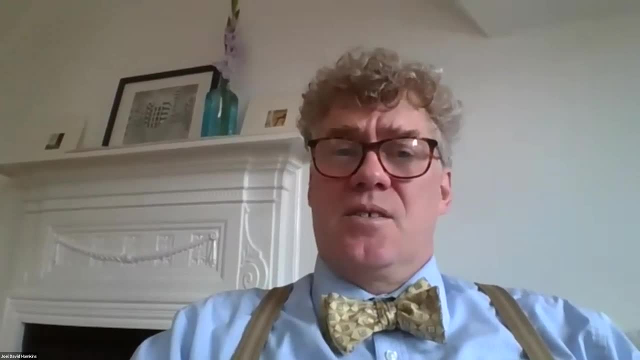 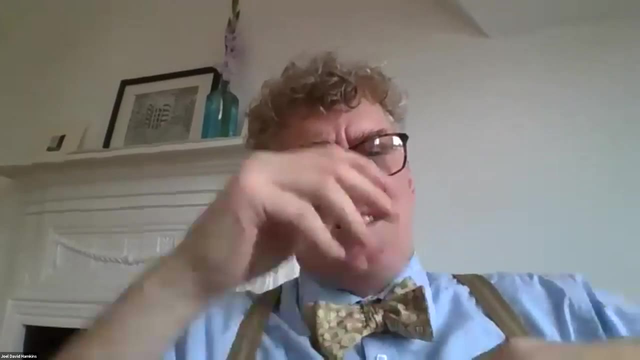 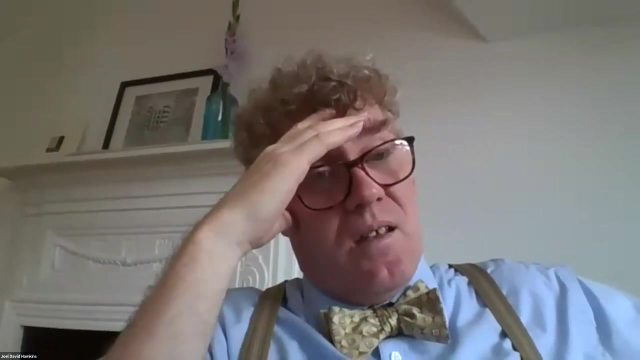 So maybe it would be more sensible, what you're talking about, to look at the functional language only so with just plus and times, And so you're going to turn them into relations. So I mean, and having say a recursive or computable, 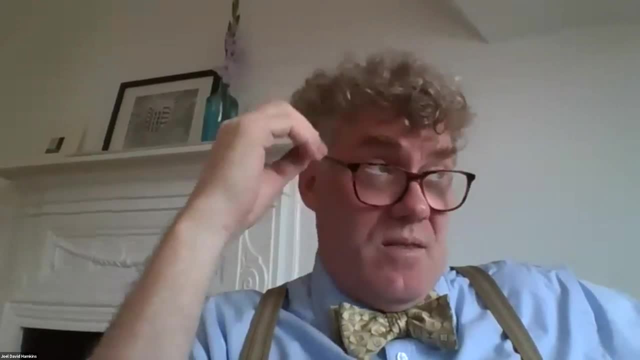 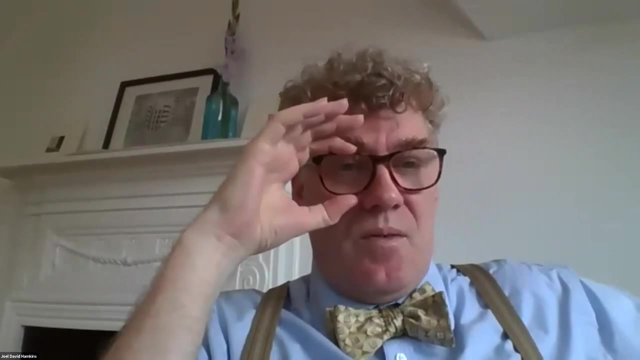 relation into the cubed, it doesn't mean that this is represented by an actual function You know. So It seems to be more general And also natural from the point of view of you know, natural from the point of view of interpretability of structures. 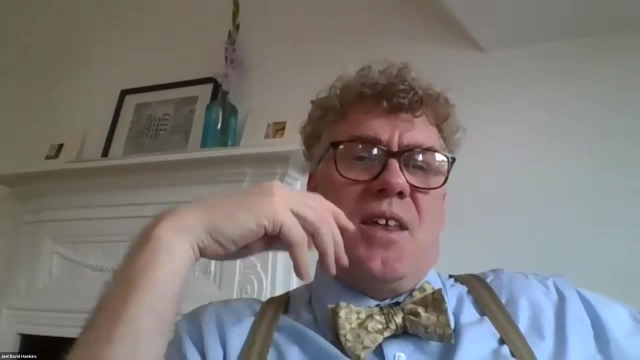 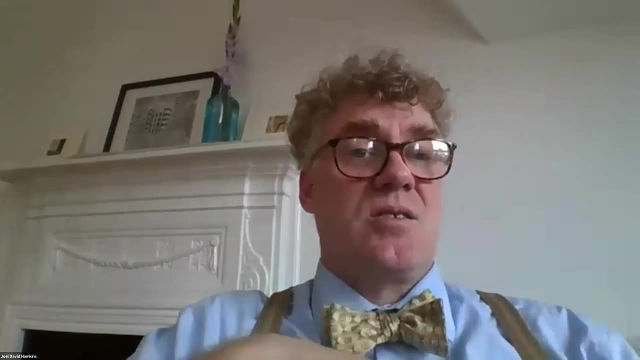 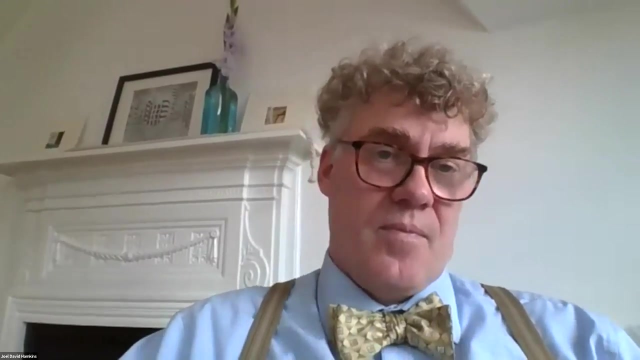 It's a kind of natural, I think it does become representative. You want the relation that you're talking about on the pre-quotient structure to be sort of full, in the sense that it's working with all the representatives. No, you simply take: you have a quotient map n to n, mod e. 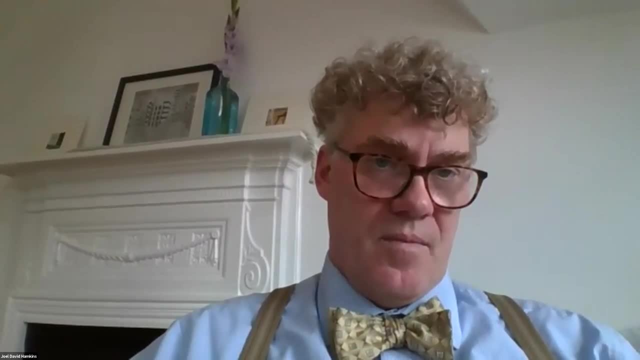 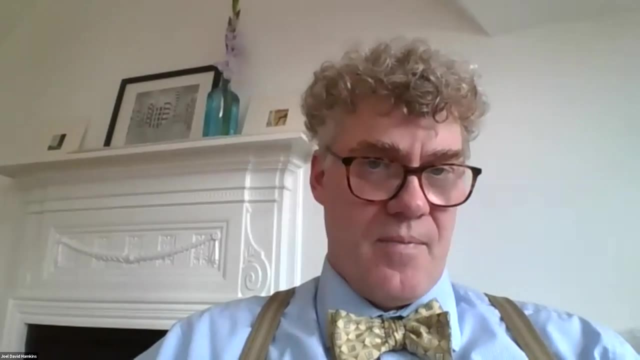 On e cubed. I have a. Yeah, I have the graph of On n cubed, you mean, And then you take. now you take the pre-image, Now of course you have. e goes to n mod e. 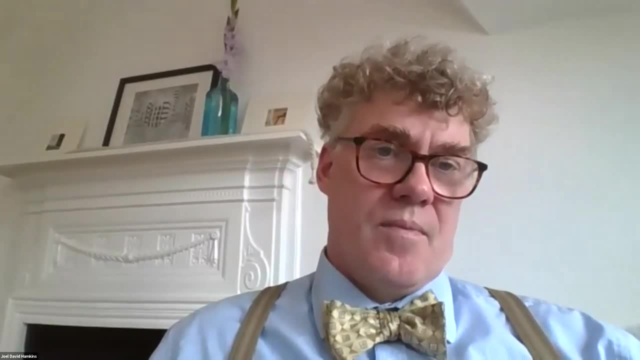 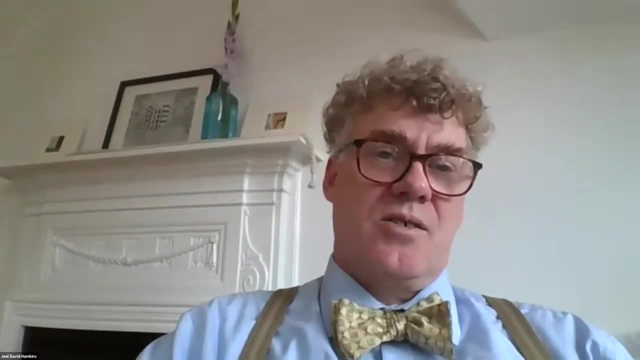 You have n cubed goes to n cubed, mod e on the 3. You take the pre-image. You take the pre-image of that graph, Right, So it has the property that I'm saying. Yeah, So you're sort of filling out all the equivalence classes. 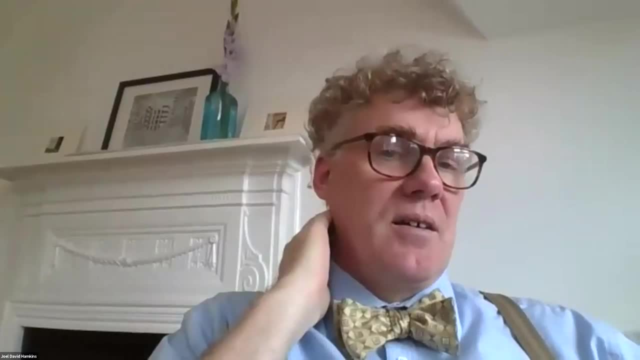 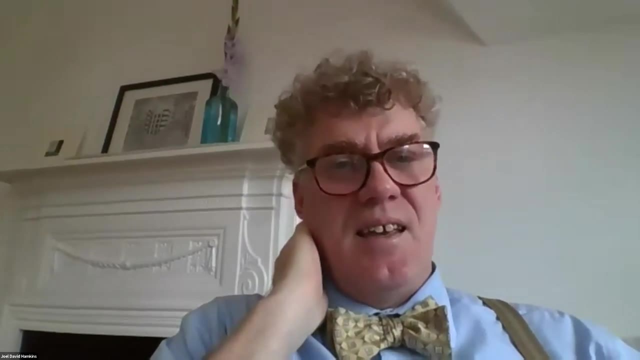 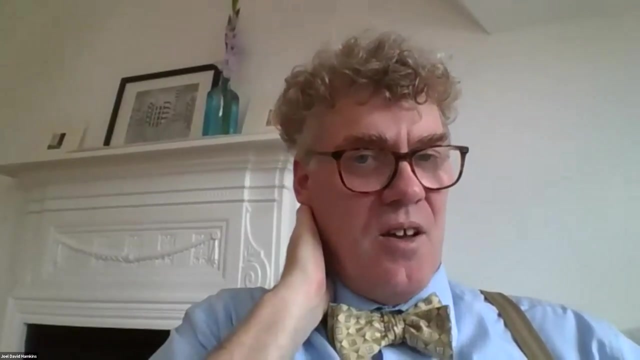 Yes, exactly, Yes, yes, yeah, yeah, Right, yeah, OK, so that's my question. I mean, if it's CE, if that's, for example, if those relations are CE, then you can compute, So it reduces to the computable case. 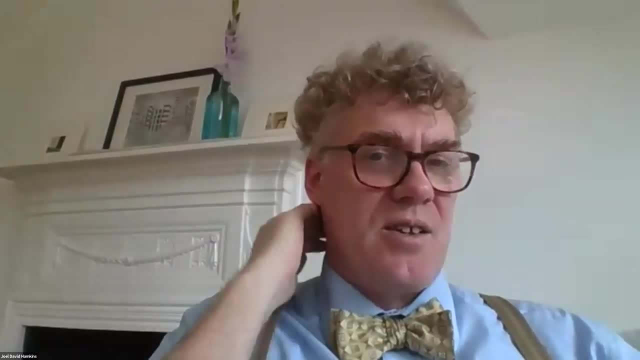 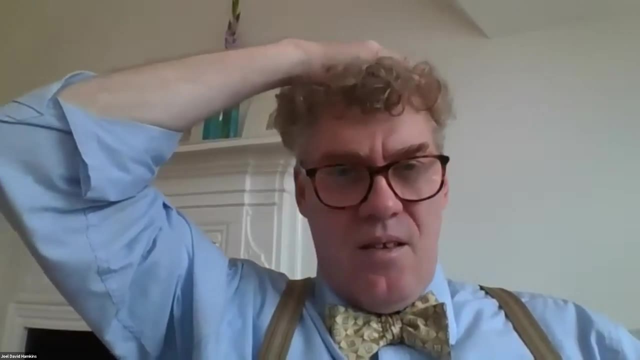 So maybe it becomes interesting if those relations are co-CE or higher or something. Yeah, Or maybe I mean Will was suggesting in the chat that you can actually turn these pre-image of graphs. You can actually pick representatives in some coherent manner. 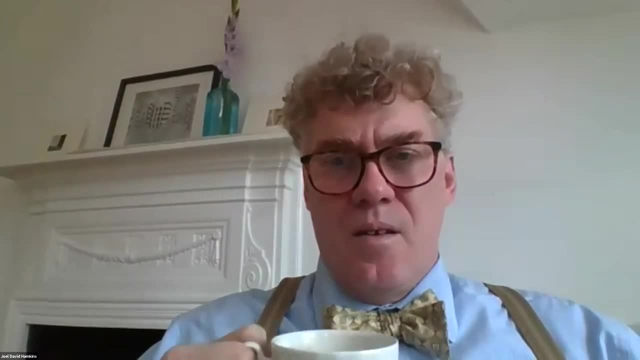 Is that what Will was saying? Maybe that's. Yeah, I think we're all saying that Same thing. I was saying that what Joel just said- that you can pick their representatives. If they're all CE, then I think you can pick their representatives. 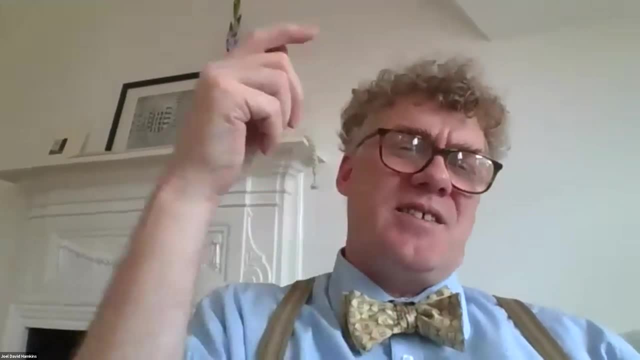 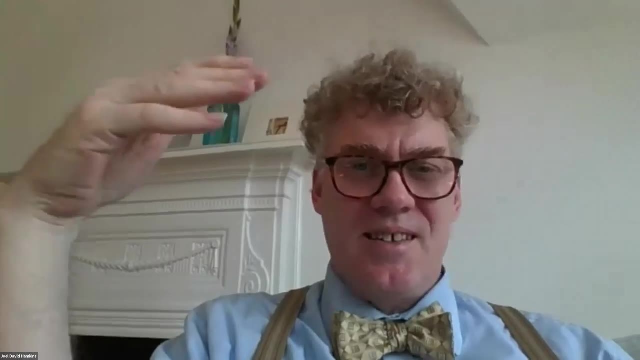 OK, Yeah, so I don't think that case is going to be different. But there's another sense in which the whole idea of looking at these computable quotients: it just doesn't play with relations as nicely as it does with functions. 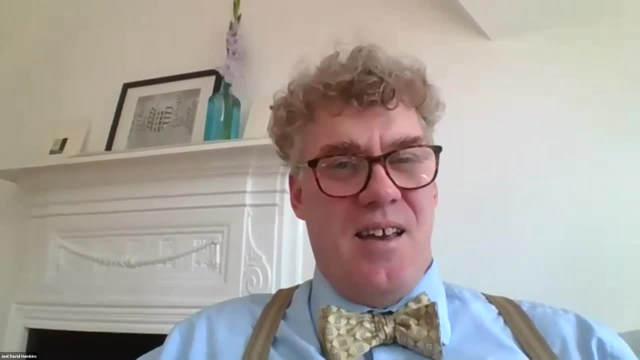 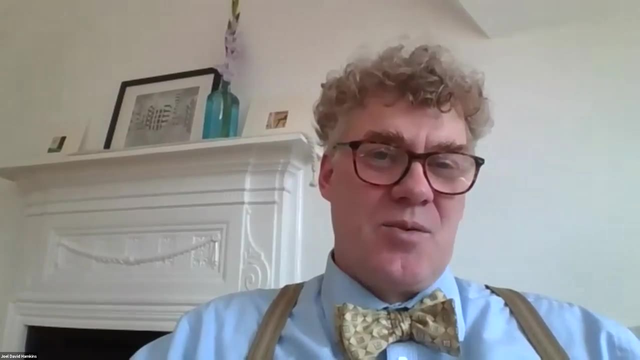 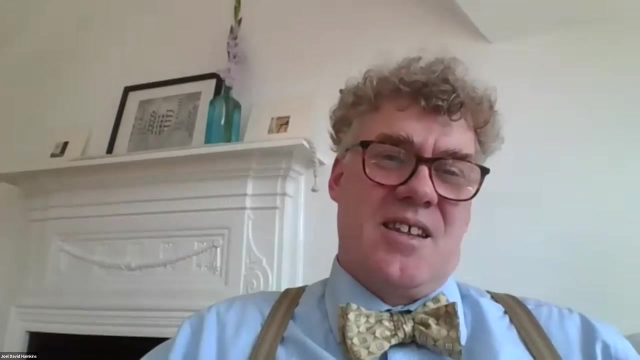 And so replacing the functions with relations is, from that perspective, the backward thing to do. You should be going the other way and replacing relations with functions, so that you can use the term algebra, which is computable, and so on, And so this is Bakayda's perspective. 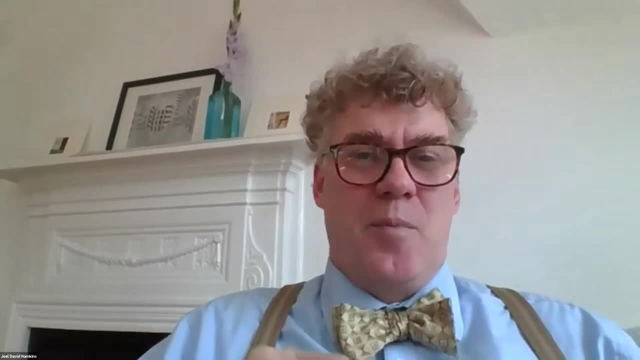 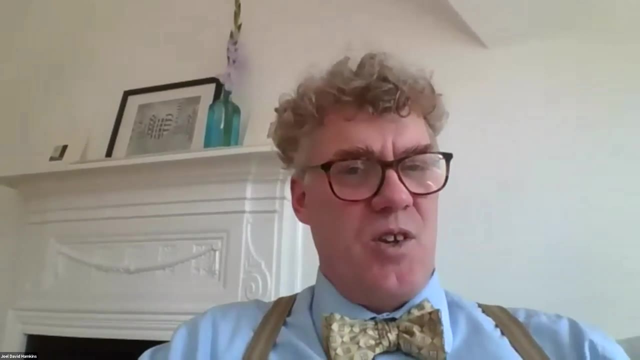 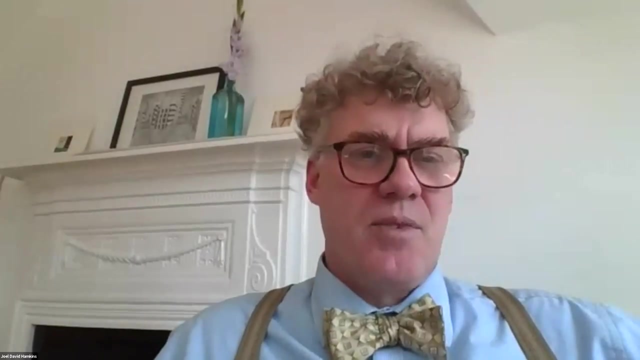 is that really? it's about universal algebra rather than about relational structures and models of set theory. But I haven't thought about the specifics of your case where you ask for the relation to be. maybe it's sigma 2 or arithmetic or projective or something. 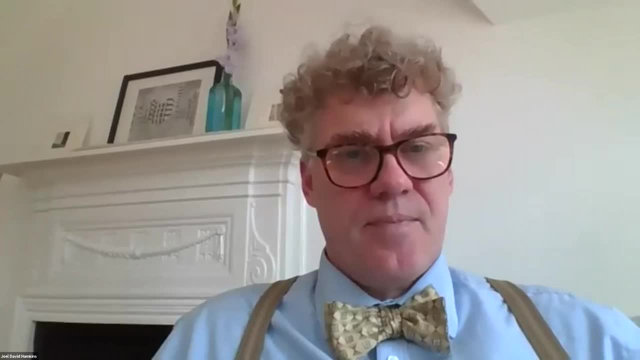 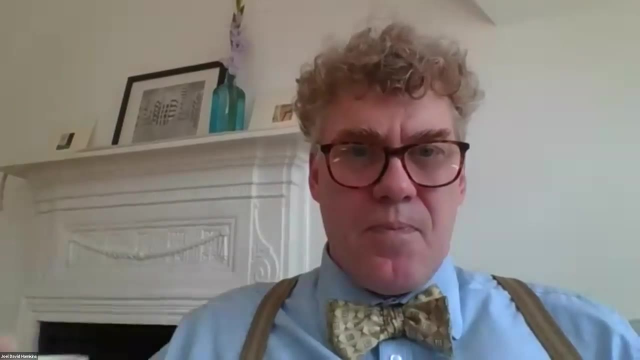 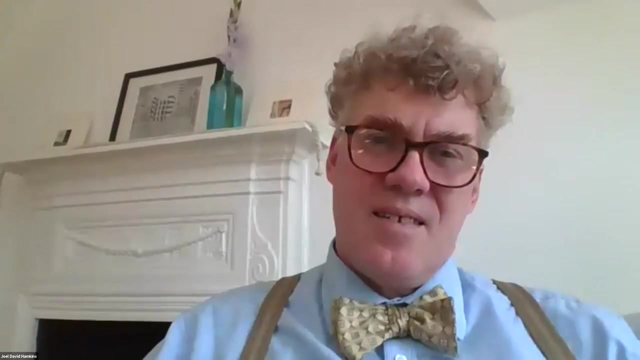 And I think that's an interesting question. I'm going to think about it, OK, Thank you. Thanks for the talk, Joel. Thank you, Oh, we have a, Dave Michael, Dave Marker. Yeah, I wonder if there's any kind of general thing. 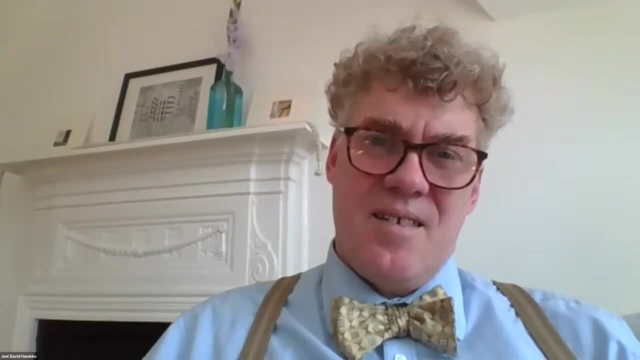 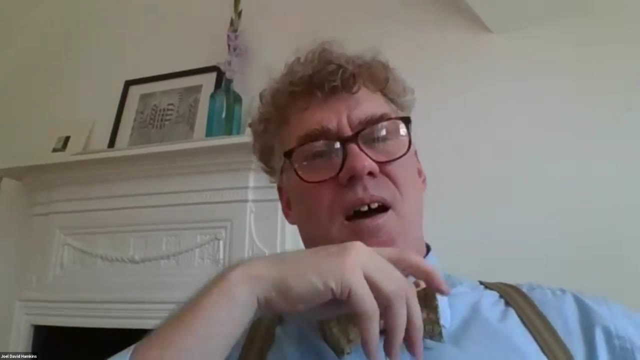 you could do in the case where you add some relation symbols, but only unary relation symbols. That seems to be much tamer than adding binary relations. Yeah, yeah, Hm. Yeah, Yeah, I mean, of course, in principle you can add anything right. 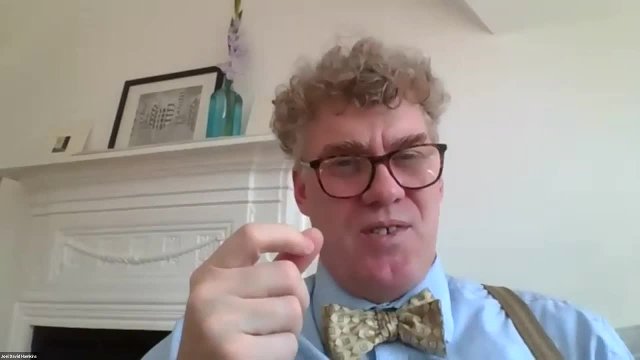 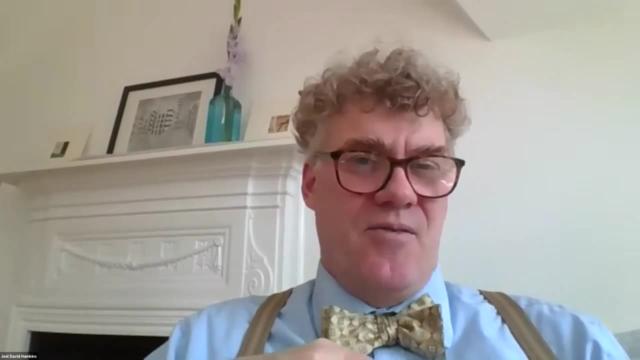 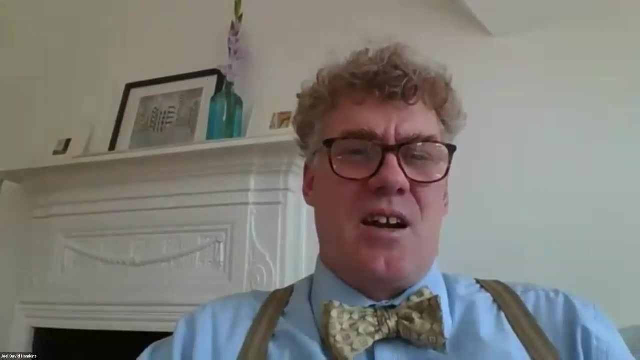 I mean, but I guess it was specifically the orders that carried this consequence for E right, When you have an order relation for which E is a congruence with respect to it, that's what led to the automatic continuity. So even other kinds of binary relations. 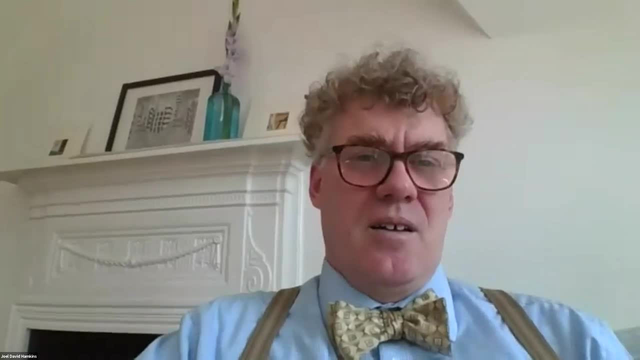 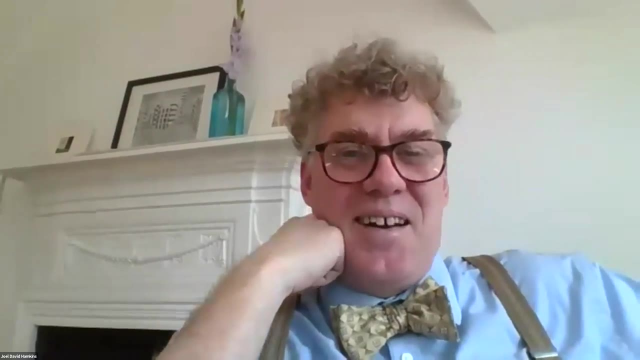 that aren't order relations maybe would be fine, but unary seems like it should be fine also, So I don't really have anything to say about that except please go ahead and look at it. I don't know what one could do with that situation. 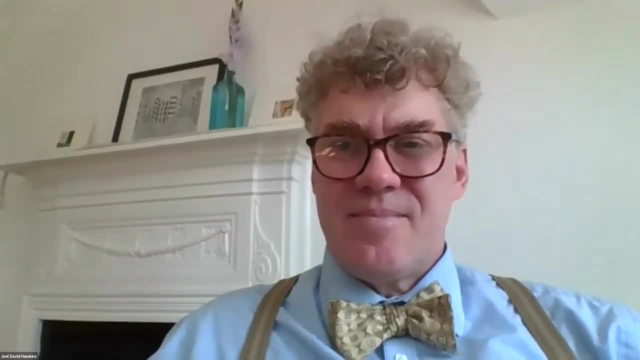 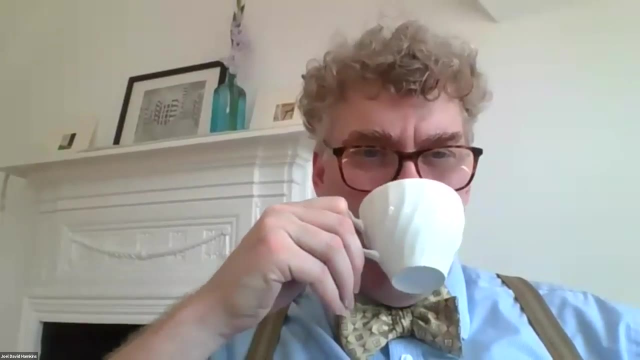 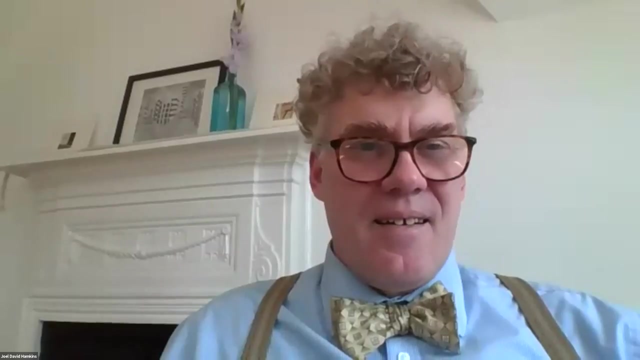 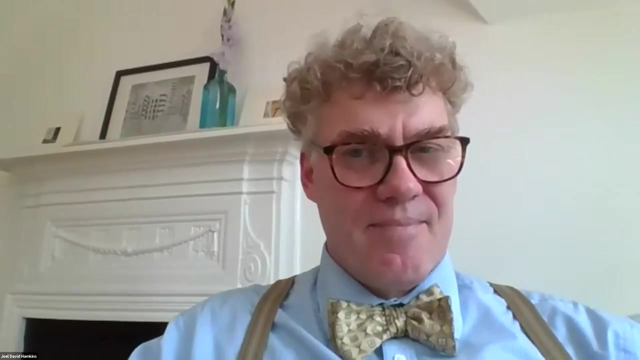 Anna, do you have more to say? I saw you raise your hand. It looks like Anand has another one right. Well, we do have more questions. And may I ask a question? Yeah, look at the kind of model of ZFs. 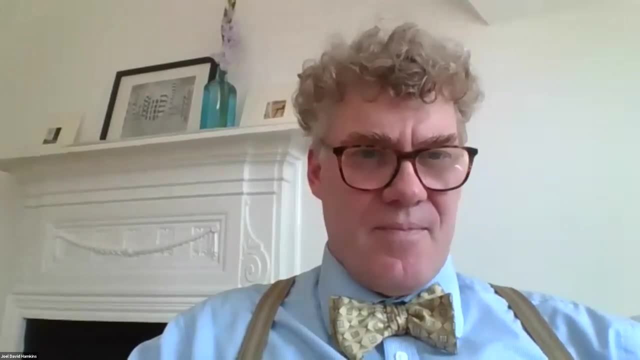 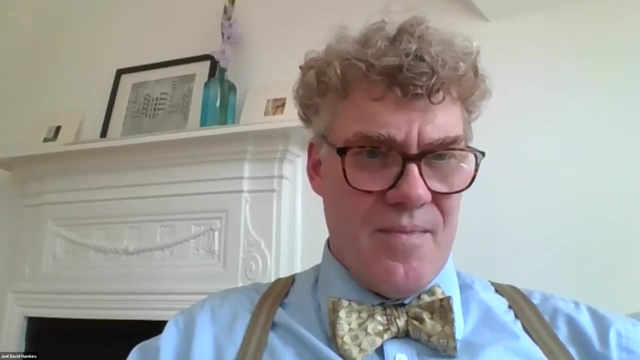 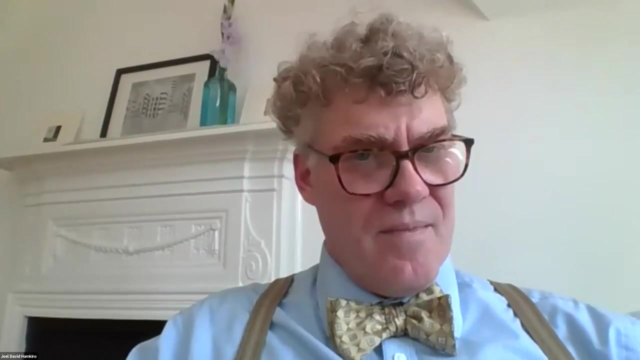 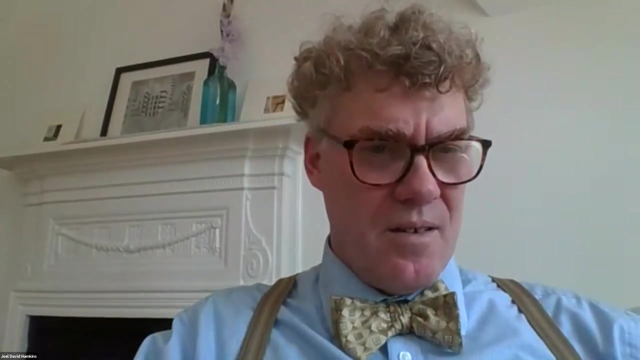 Also the finite set theory. do you have similar results concerning something essentially weaker than even finite set theory, say some extension of biograph, Extension of which? Some extension of just the biograph? Oh, I see, No, I guess right. 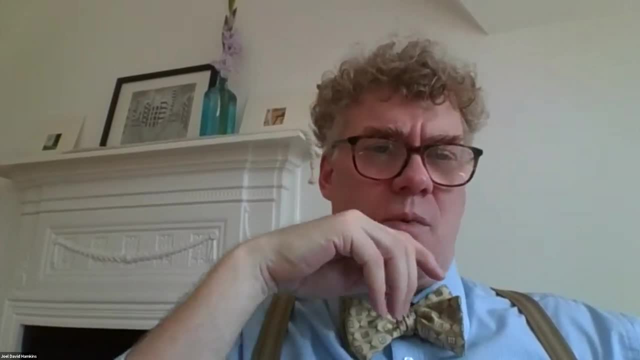 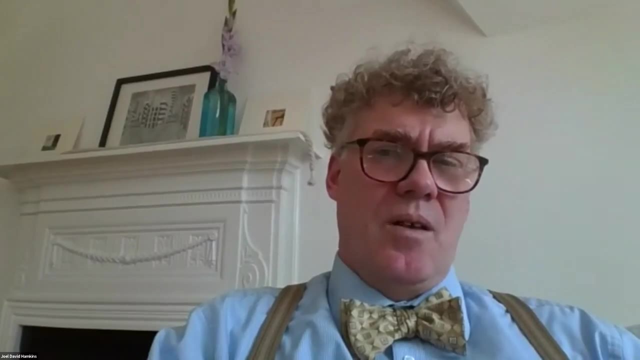 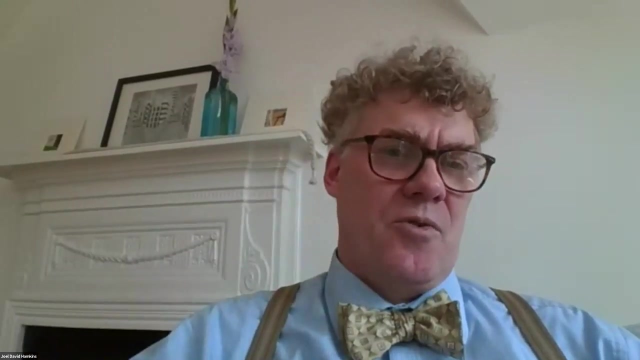 I'm not sure what the optimal thing is known, even in the case of Tenenbaum, about pushing it below PA. I guess it would go. I mean, we just needed the computable inseparability, And so it doesn't seem like we need all of PA at all. 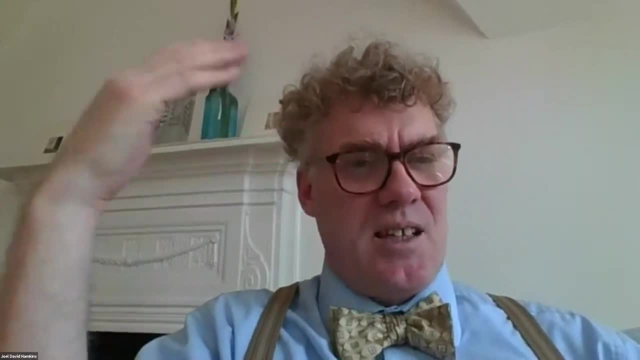 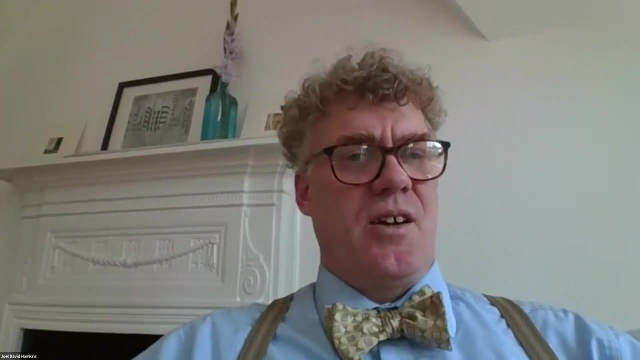 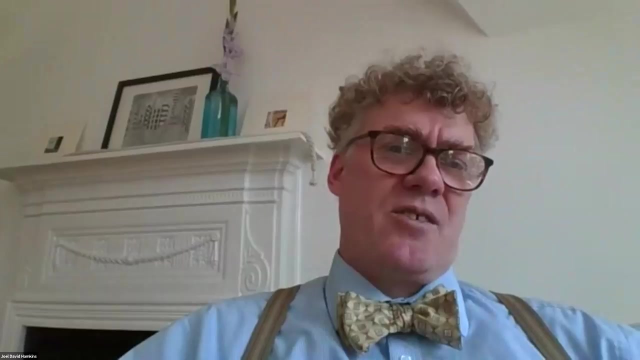 for the usual Tenenbaum thing And in the case of set theory, the finite set theory case basically reduced to the PA argument. Of course, for finite set theory it was about nonstandard models of finite set theory, But of course there is a computable standard model. 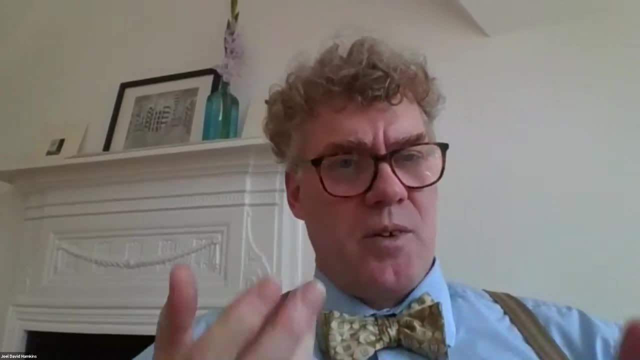 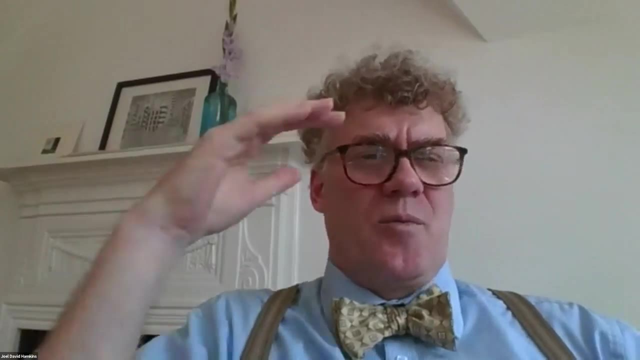 of finite set theory, the Ackermann model, the Ackermann interpretation of finite set theory, I mean the hereditary finite sets, have a computable presentation. So we're talking about nonstandard models there And of course I don't think you. 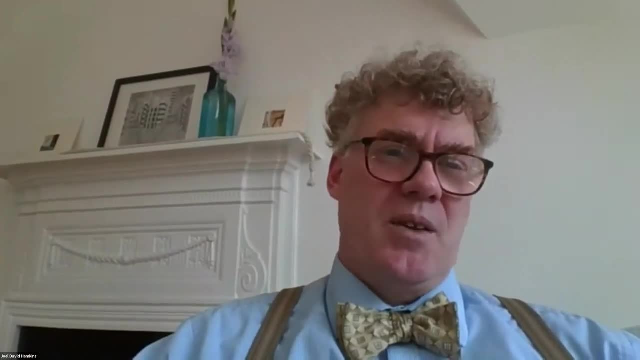 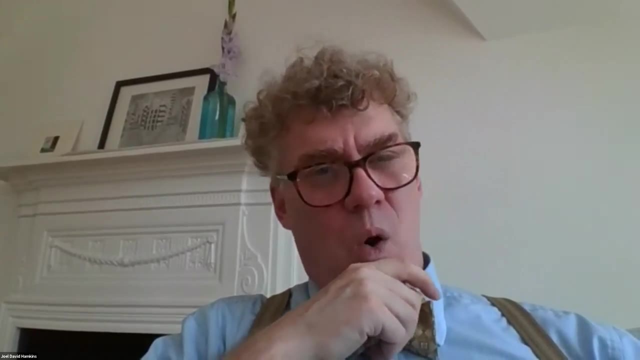 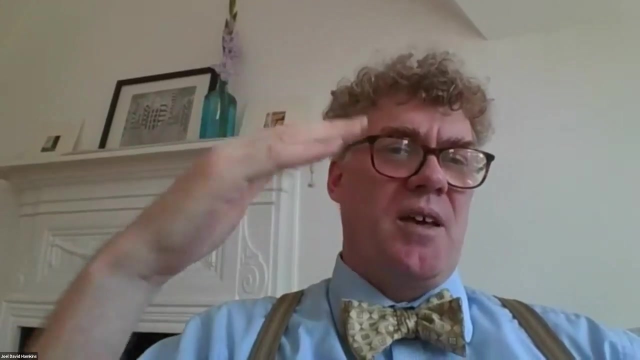 need full separation and so on. Maybe sigma 1 is enough, But probably the models of arithmetic. people know exactly the boundary where the Tenenbaum phenomenon starts happening. I had just stated it for full PA, but you don't need all of that. 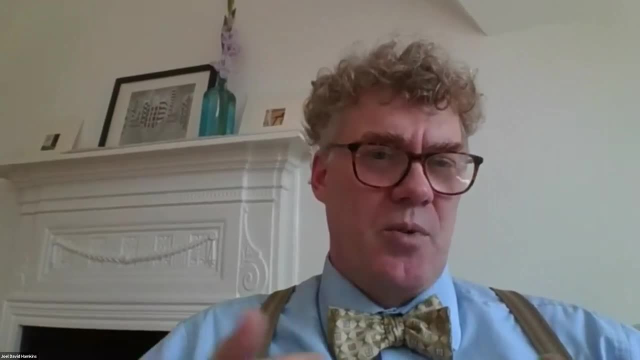 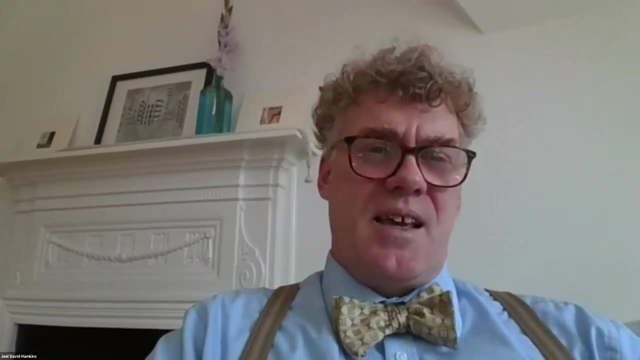 Basically it's at the level of sigma 1, because we're talking about computable inseparability, And I would expect a similar thing to happen for models of set theory, But I don't know exactly where that boundary is. Thank you. 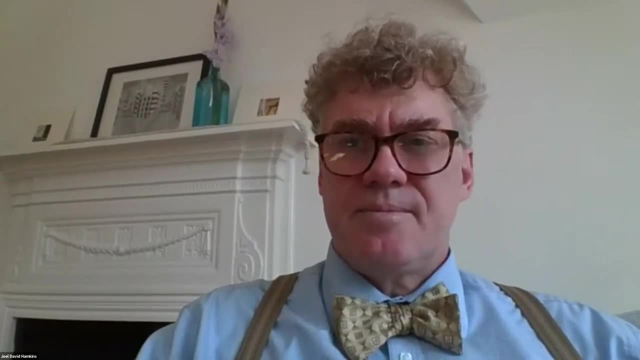 If there's no more questions, that's thanks to our speakers here. Thank you. 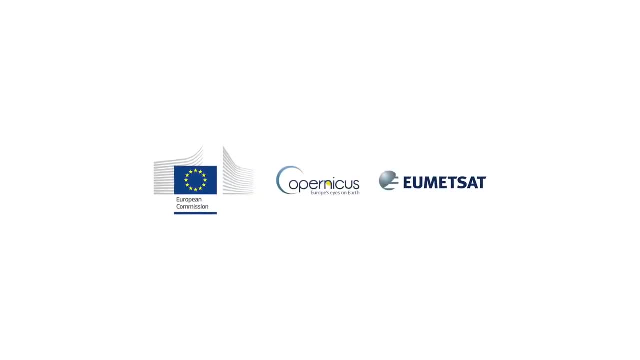 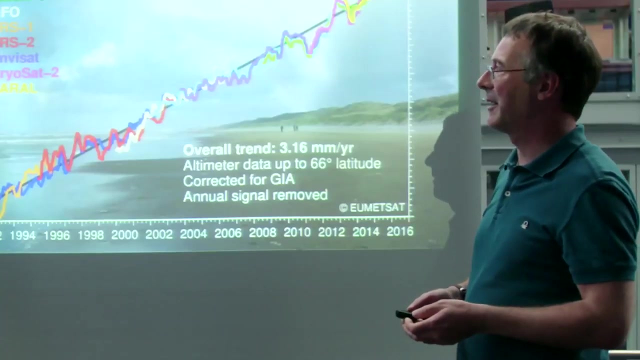 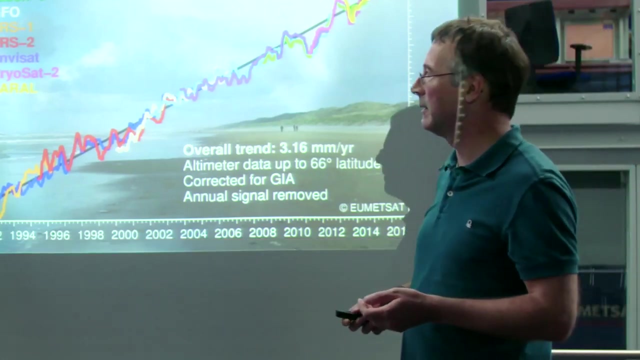 So in general we know that sea level is rising, so presumably you can also measure that using altimetry Exactly, and we have been measuring this basically since 1991 with the first European remote sensing satellite, EOS-1, which was launched. 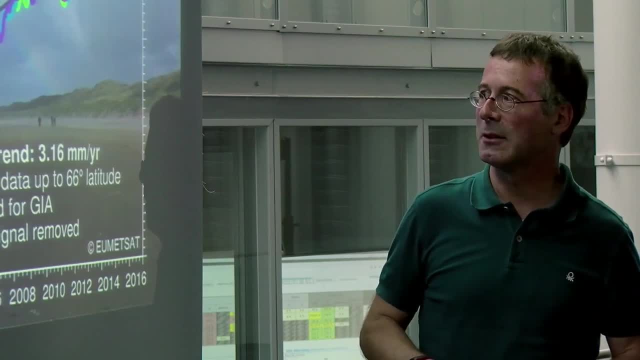 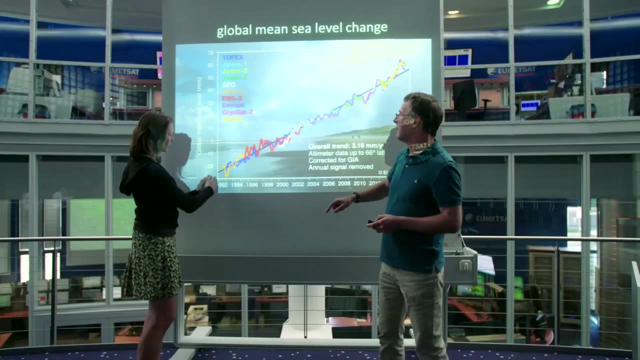 in 1991, shortly followed by Topex Poseidon. And I said already, Topex Poseidon is this reference mission, That's one of the better altimeter satellites. So we've got time going along the bottom 1991 here and today over there. 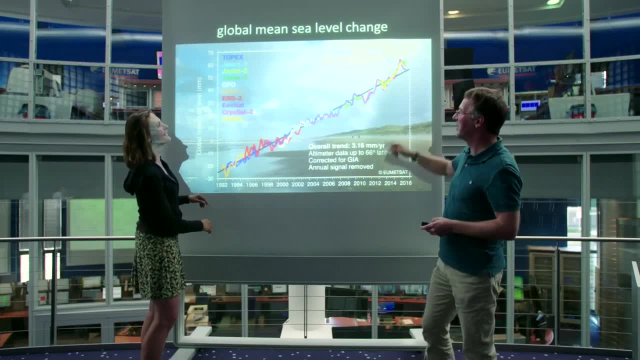 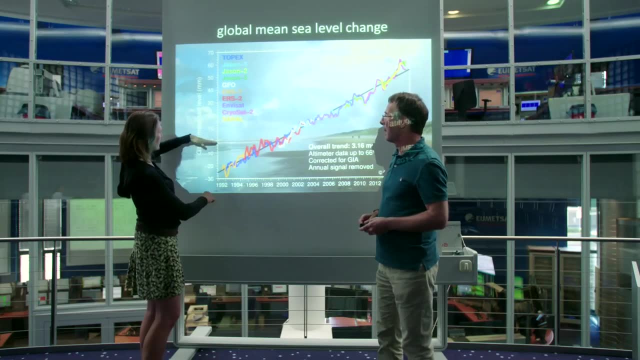 And today at the end. yes, I actually made this plot last week, so it's really up to date. It has even a little bit of Jason-3 in there already, And this is global mean sea level. so you've picked a reference zero here. So this is not. 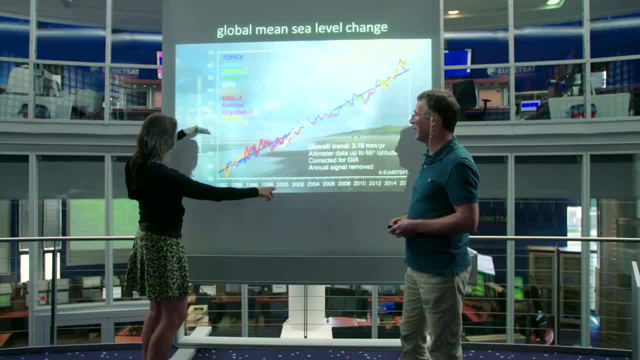 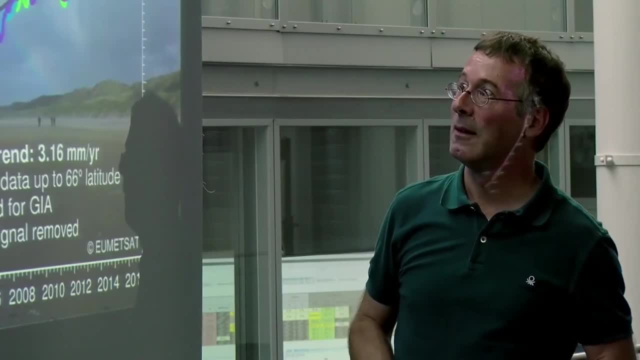 because sea level is negative, but because… 2000.. …compared to the year 2000, it was a bit lower. So it's 30 millimetres lower, three centimetres lower in 1991 than it was in 2000.. And then this…: 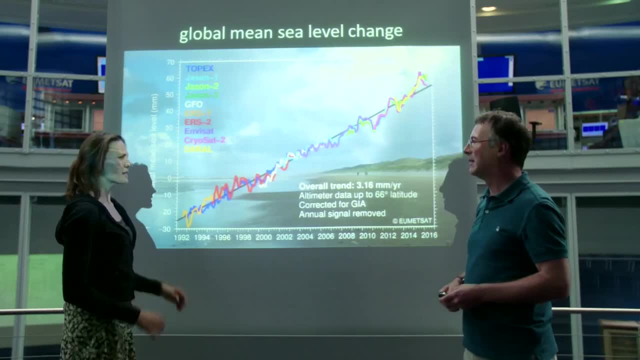 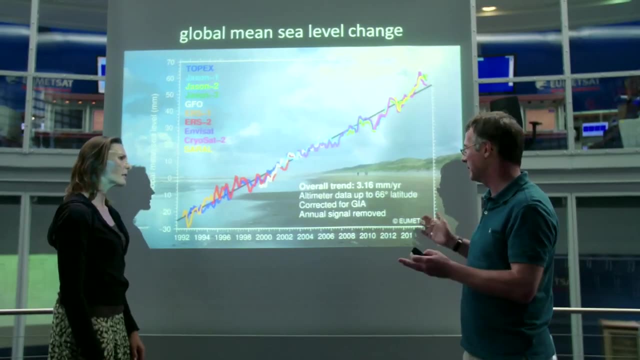 And now it's almost six centimetres higher than in 2000.. So that's a big change. Yeah, we have raised sea level globally in the mean by eight centimetres in just this period. So in the period that I was working on this, we have increased sea level by eight.